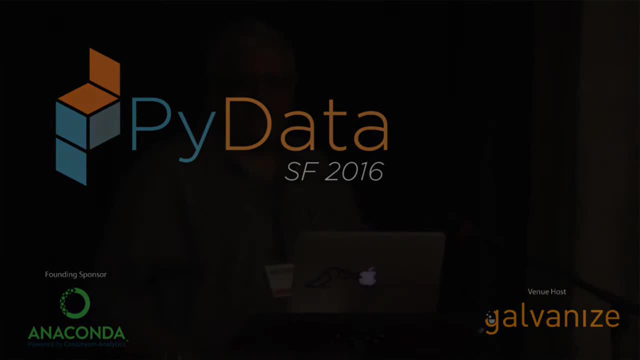 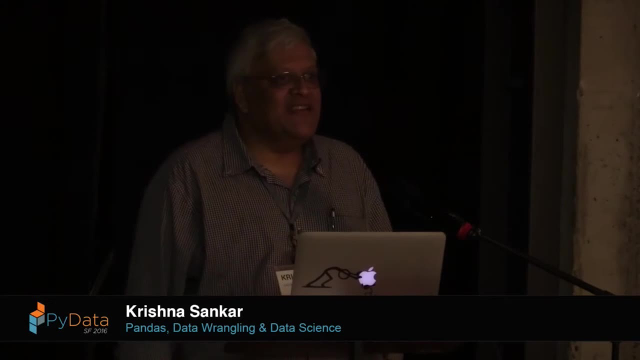 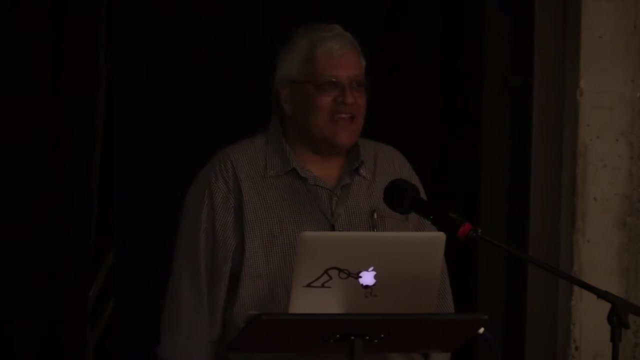 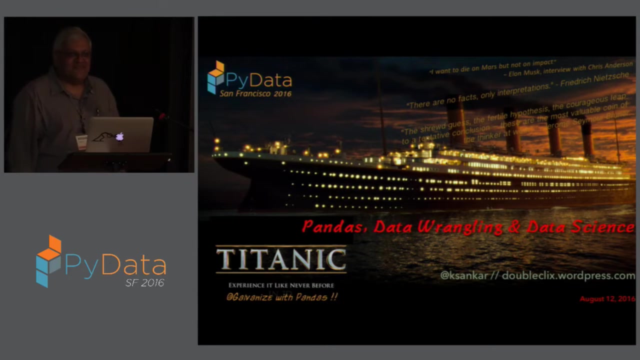 Can you hear me? well, At least you can see it now, right, When we start looking at this thing. So, anyway, I don't know whether you have seen the- what is that? the Polar Express, right? So in that, the Tom Hanks says, if you are looking for penguins, they are on the other end, right, Because the penguins are on the south pole and he's on the north pole. So, like that, if you are looking for recommendations, it's on their end. 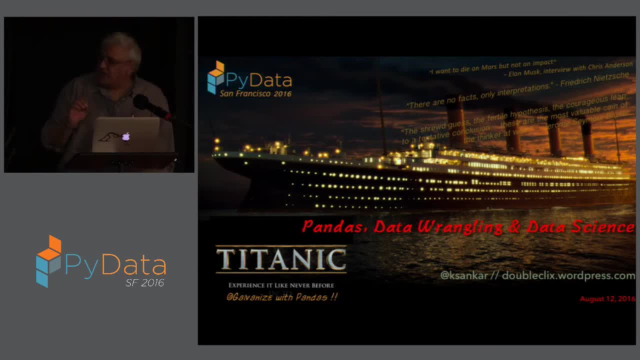 On the other end and we are here. So this is PANDAS, data wrangling and data science. in that order. PANDAS is the main focus, with the data wrangling. I'm not going too deep into data science because it, you know, we could do a whole machine learning tutorial for a whole day or that kind of stuff, right? 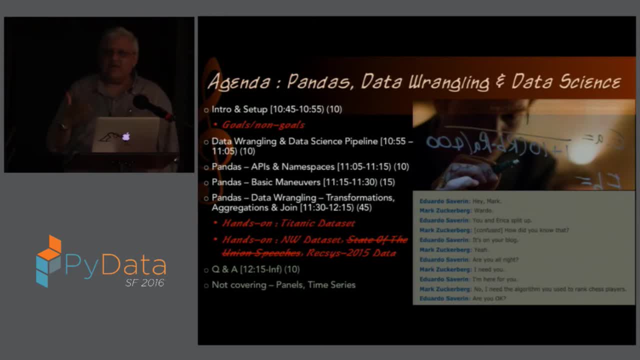 The agenda. we will talk about data wrangling pipeline, just to get a feel, for what does it mean? data wrangling with respect to a machine learning ecosystem, with respect to a data science type of work, right, And then we will go into the basic maneuvers. Is everybody familiar with PANDAS here? Or there are people who haven't used PANDAS before. A few folks are there, right, Okay, So that is a good one. So that is a good one. 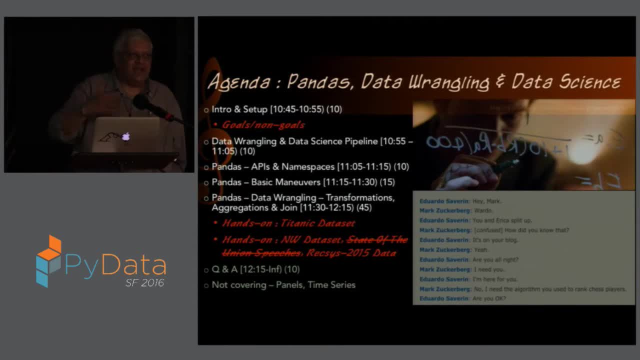 I'm not going to go into all the basic maneuvers because I didn't know that, coming in, I didn't know how many people are in back and forth. We will take a quick: the basic maneuvers, right You do. you know, if you are looking at things, you have to at least look at the basic ones and say what are the primitives that we have. So we will go quickly, go through the basic maneuvers and then we will go through multiple data sets. The idea is to look at PANDAS, to learn PANDAS, to understand the various mechanisms by doing stuff right, Rather than just looking at abstract and saying, well, I don't know what I'm doing. 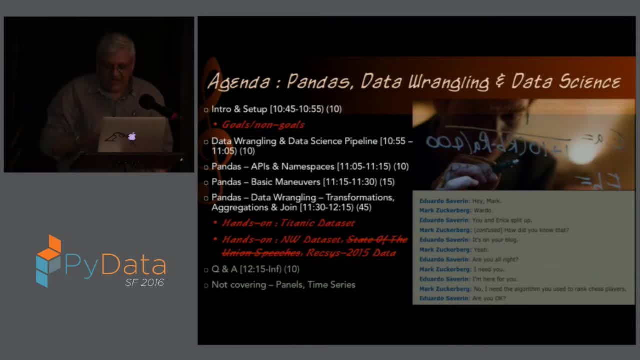 these are the APIs, So that's what we will do. We have 90 minutes and, of course, we have the lunch time. I'm just kidding, I'm not going to take the whole lunch time, But we'll see how it goes. 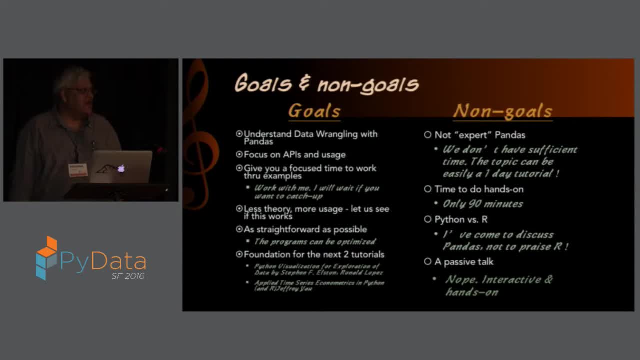 A couple of things: The goals, The goals and non-goals. It's always important today what we plan to do and we don't plan to do. The goals are to understand data wrangling pandas. focus on API usage. give you some focus time to work through the examples. 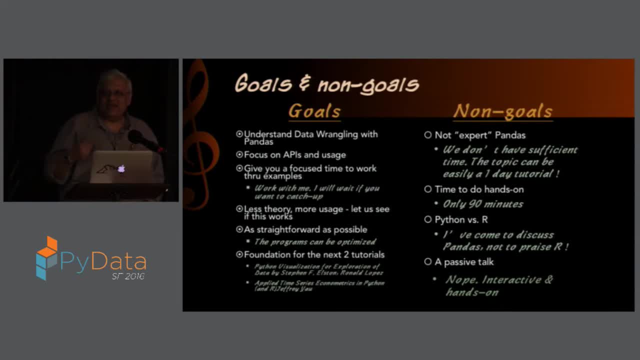 It's 90 minutes. We can't do a hands-on tutorial, that kind of stuff. I don't know whether you folks got a chance to download pandas and the IPython notebook And also the data and the code is in GitHub So you can get it from GitHub and you can do that. 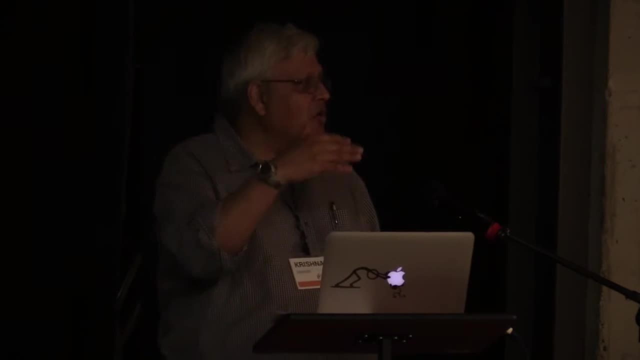 Or, after this is over, you can go and download the notebook, Run them through. The data is there so that you can take a look at it and you can understand the mechanisms and mechanics. Less theory and more usage, and straightforward as possible. These programs are simple. 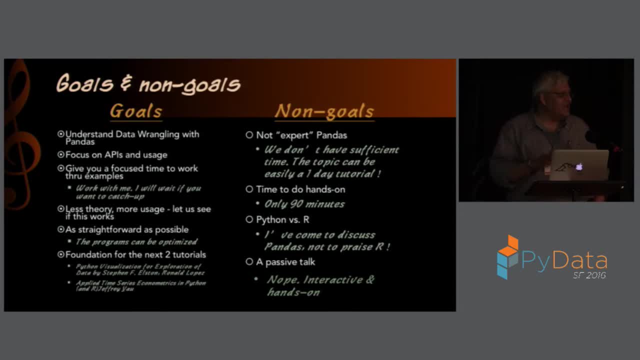 straightforward programs. They are not too. you know that way we go through the pandas, not the rest of the stuff, And this is the foundation for the next two tutorials: Visualization as well as the time series. These are the two things coming up, probably. 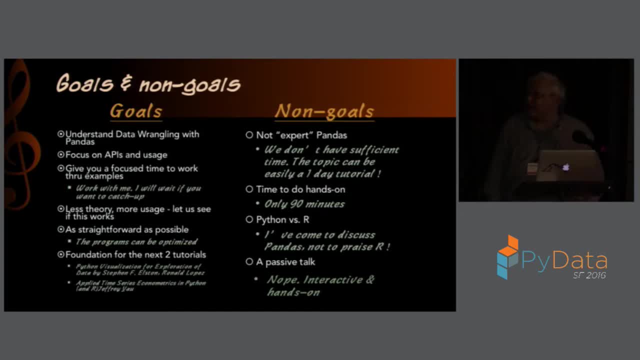 They stack up one after the other. One is set, one you can work on, You know, not on expert pandas, of course Not. you know we have to get through the first level to get to that second level. Time to do hands-on: only 90 minutes, And there is things like you know. one of the questions: 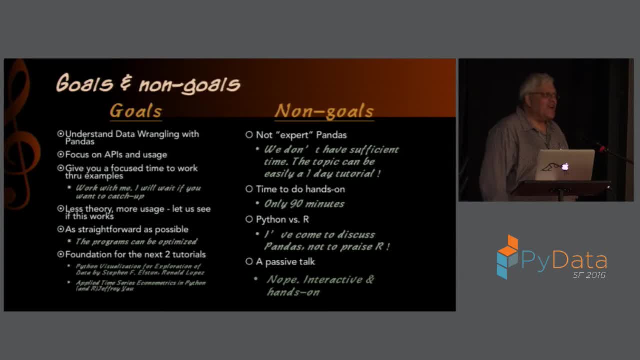 that come up with Python and data science is people look at it and say, okay, how does it compare with R and various other languages? right? So, quoting Shakespeare, I come to discuss pandas, not to place R or whatever it is. 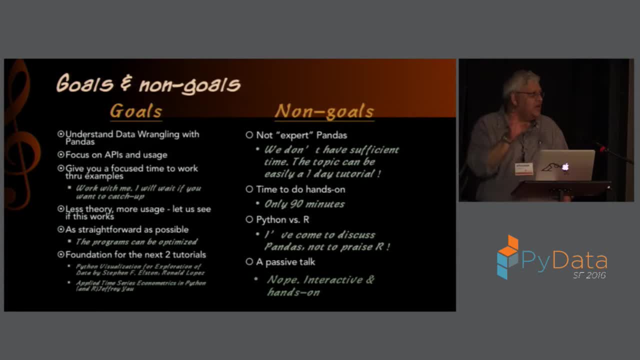 So that one And interactive and hands-on. Stop me any time, anything set, you know time If you don't understand something or if you have some questions, if you have some thoughts, if you have some ideas, stop me and you know we'll go through that one. 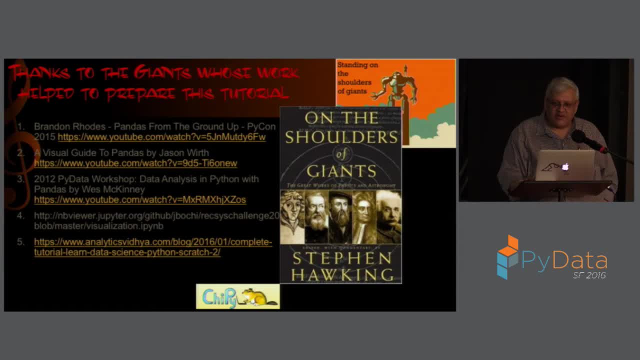 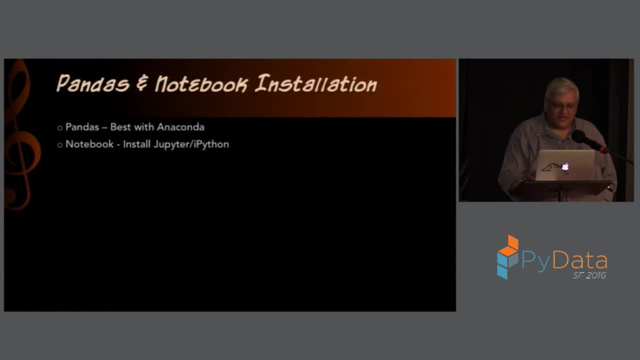 I do want to thank the, you know, folks standing on the shoulders of giants. I have just a blurb about me, the things that I do. I'll skip through because we have 90 minutes. So the installation of pandas. the best is done with Anaconda. 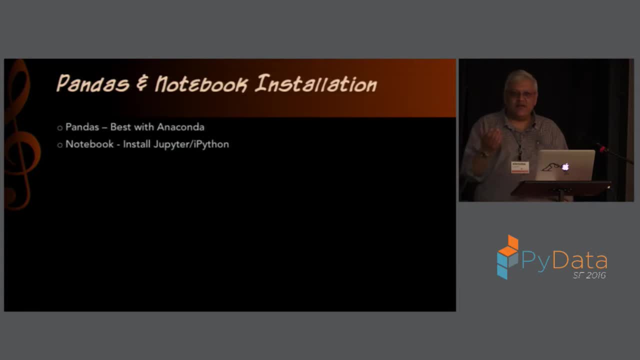 And the IPython notebook. These are the two. the thing, depending on the code, Depending on your operating system- you know whether it is Mac or Unix or Windows- you can install Anaconda. It has, you know, IPython and various other things. 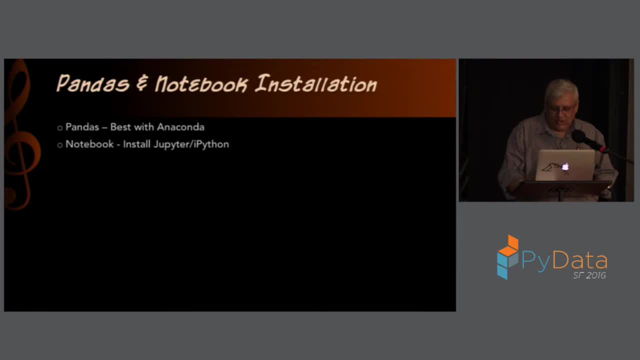 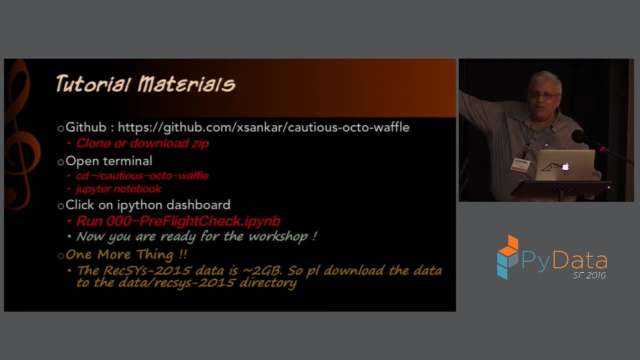 And you can also install the Jupyter notebook. The tutorial materials are here. By the way, if you go to the my GitHub, it is there in the name of the. you know, if you look at the description I do have put there as well. 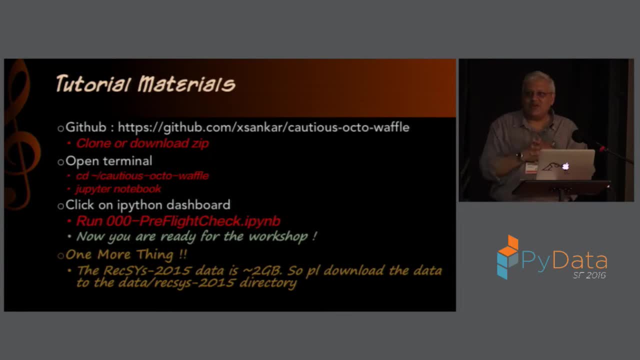 If you go there you also have a link to the slides, So you don't need to write down the link to the slides. Slides are in SlideShare. But if you can't get to the SlideShare, maybe I will put a PDF in here as well. 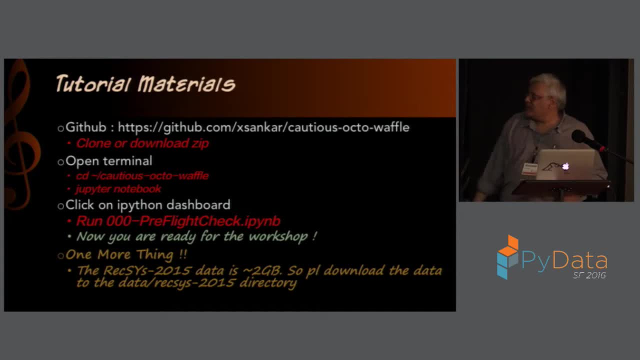 So that way, everything is in there. I haven't done that, but I will do that one. So let us quickly, you know, just to get this up and running right. You have the usually, okay, This is a good one to see how this thing works out. 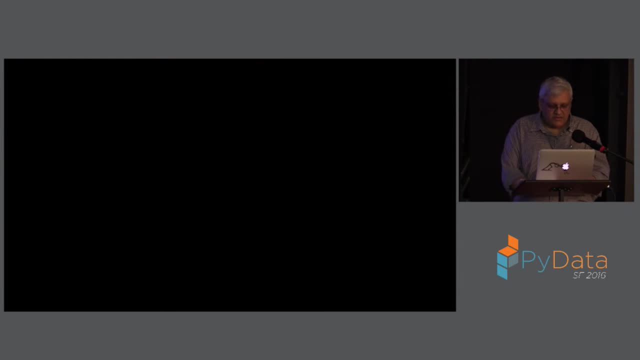 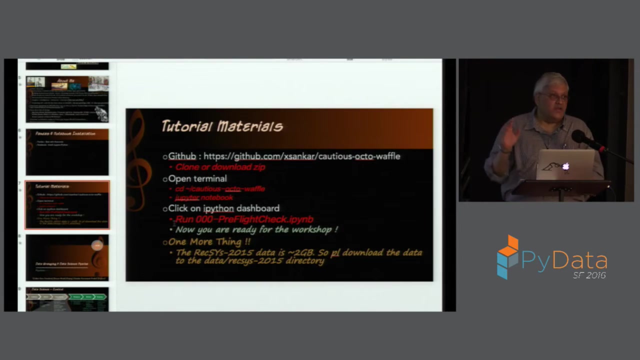 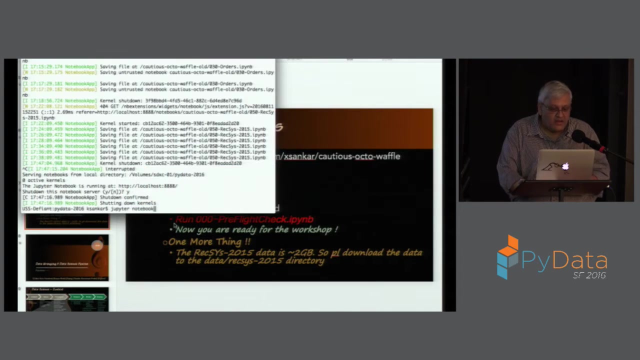 Because most probably I will put it in this mode rather than the slideshow. It's a lot easier And you can see it anyway, right? Yeah, And it is not much in there. Let me see how much you can see this guy. 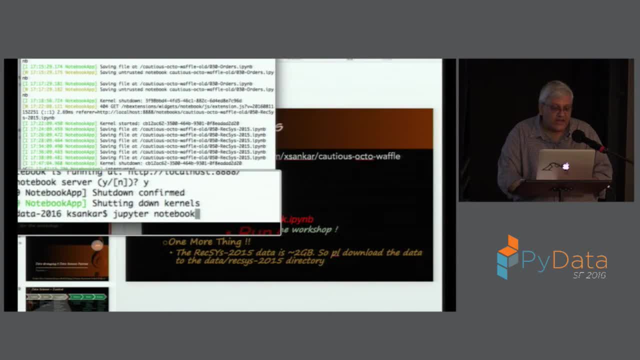 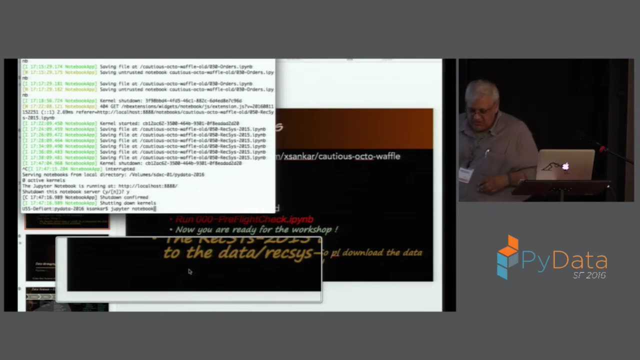 I do have this thing so that I can actually show more. You know more of this thing. How does it look? Can everybody see this one? I want to see, Let me, I'm going to just walk down and see how much. 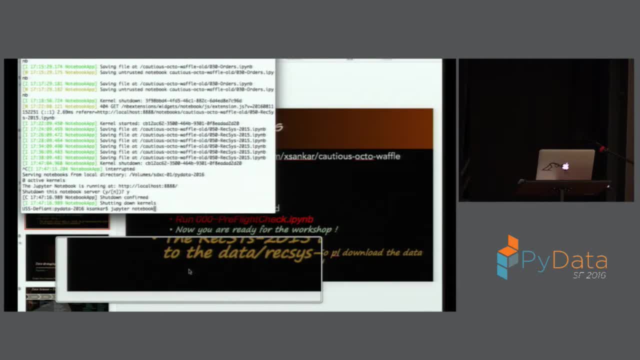 So that way I get a feel for how much you can see. right, Right, Okay. So what I will do? Yeah, What I will do is I will show. if I show this guy, does this make it easier to see? 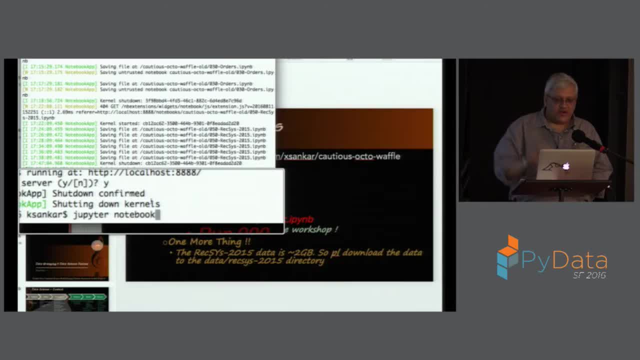 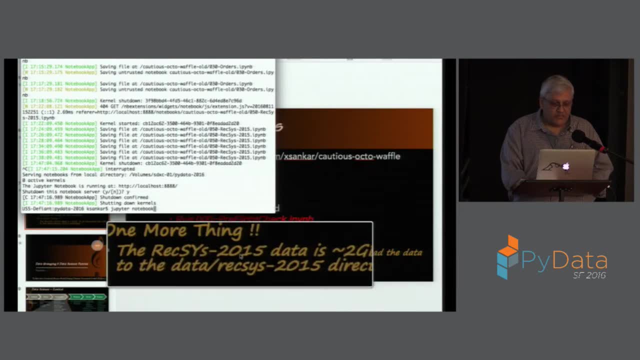 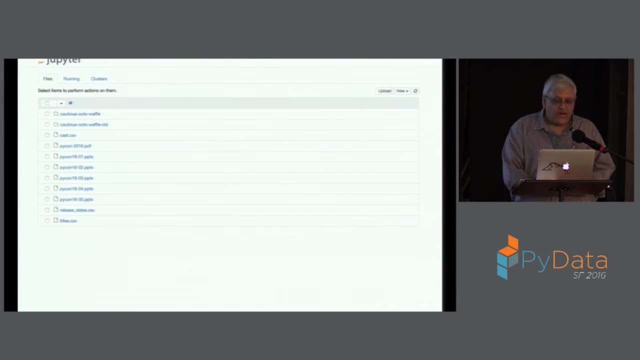 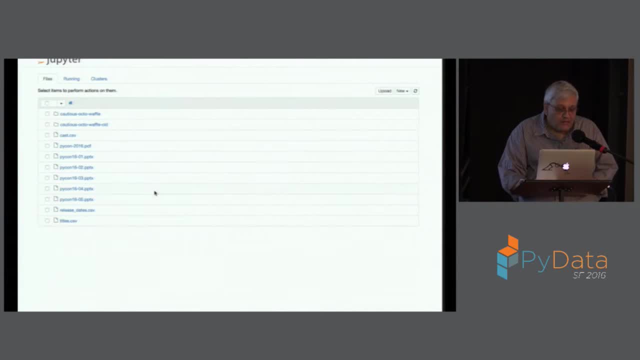 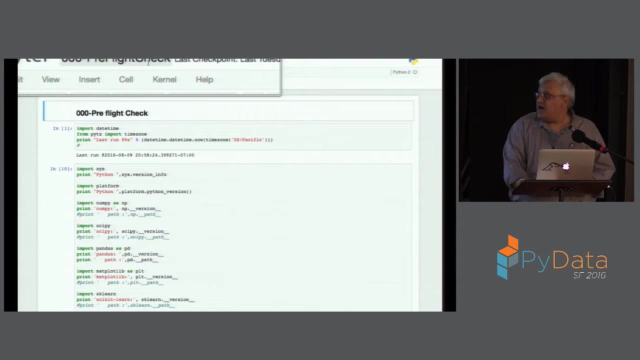 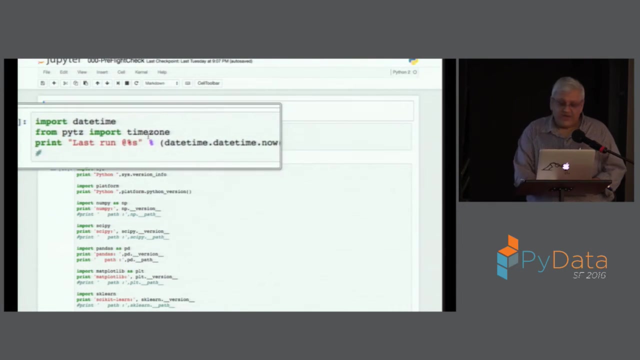 If you had installed IPython and everything, it will start up. So I am using the old directory, but you will see this one pre-flight check. So this is the pre-flight check notebook. You click on the notebook and there is the pre-flight check. 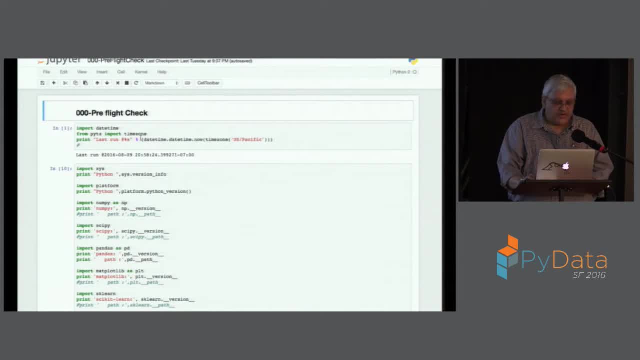 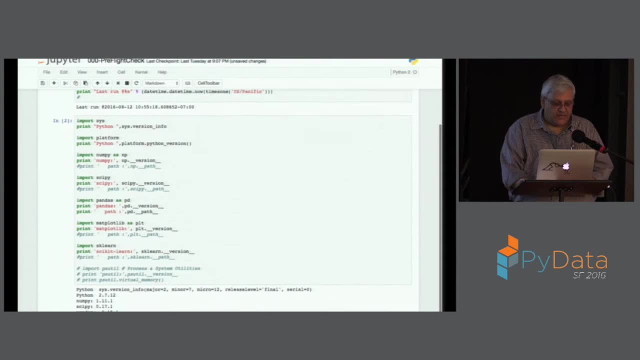 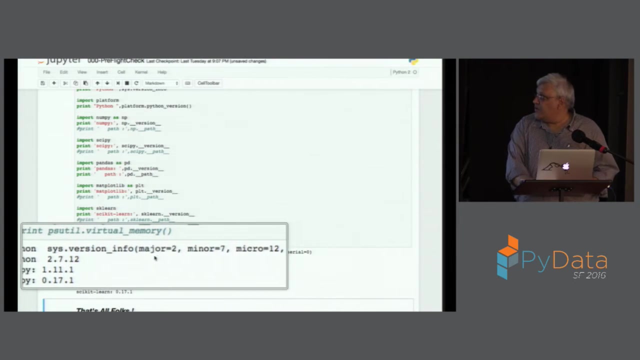 So, in order to run something, what you do is you press Shift-Enter, right, You go to this thing, You press Shift-Enter, You press Shift-Enter, It comes in. You will see that when you do this thing, you will see the version numbers, right. 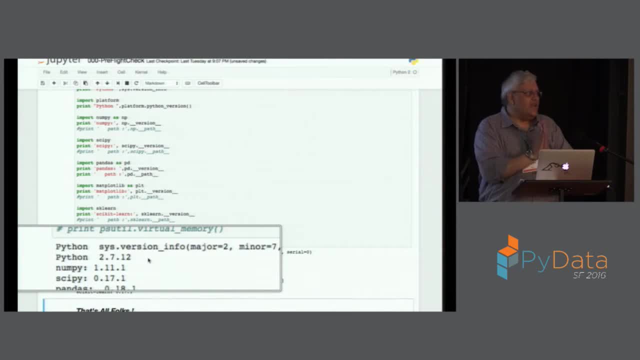 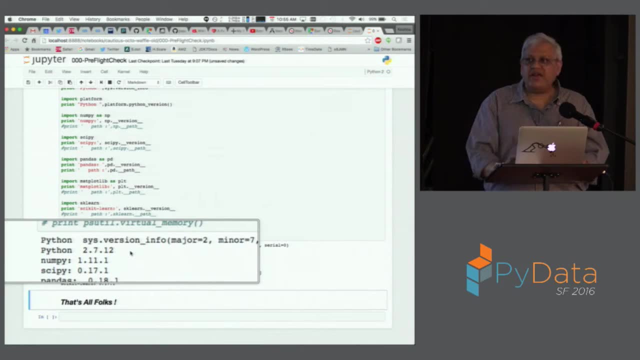 So it is just a starting right. So it tells you that the IPython is installed and you have all the other things in there, So let us hold it there. So this is how you start up. use IPython to start the thing in. 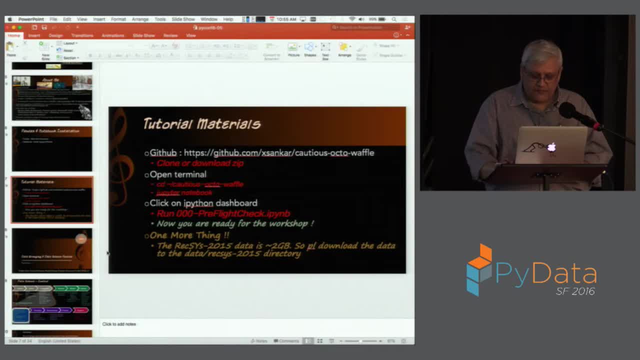 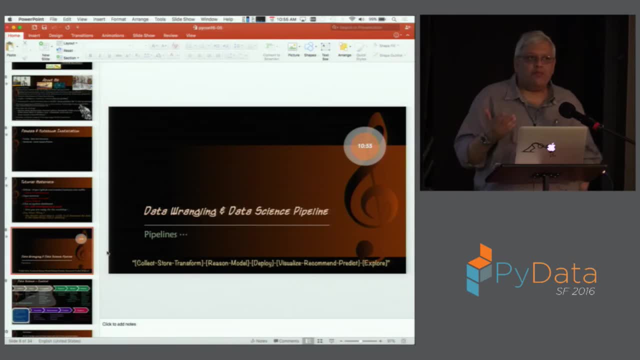 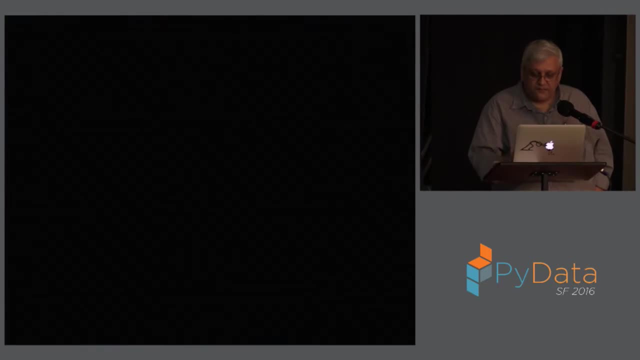 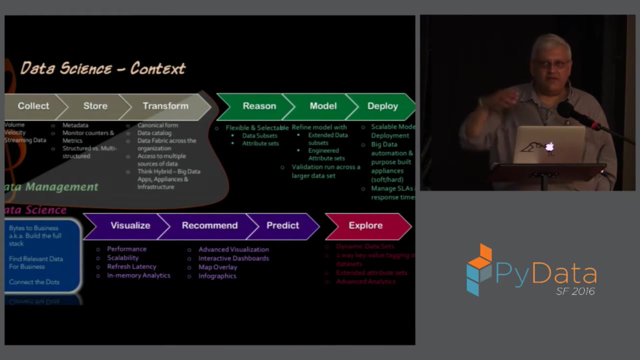 So let us go back So quickly go through. what does this mean in terms of a pipeline? We will do it only a couple of times because I just have a few slides at the beginning. So when you talk about a data science pipeline, right. where does Pandas fit in the demand? 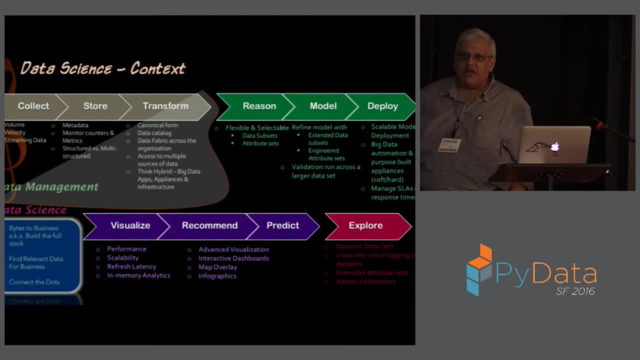 of a data science pipeline. You have the collect, store and transform right. This is where data comes in from multiple places. You start collect and collect also could be distributed. collect the various other things, things like Kafka. There'll be various other infrastructures in place where you collect the data. 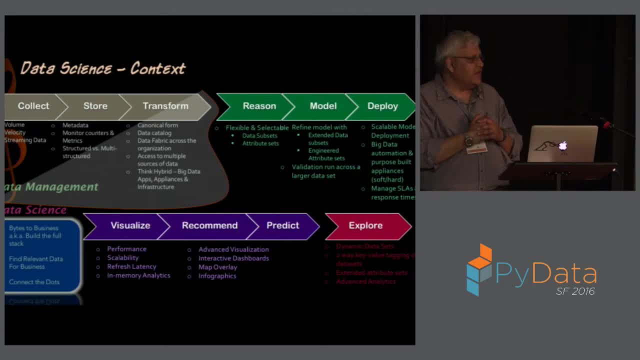 And, of course, store. Again, the store could be HDFS, it could be distributed storage, It could even be things like Cassandra, that kind of stuff, And then you have the transform. So this is where the pandas is right. 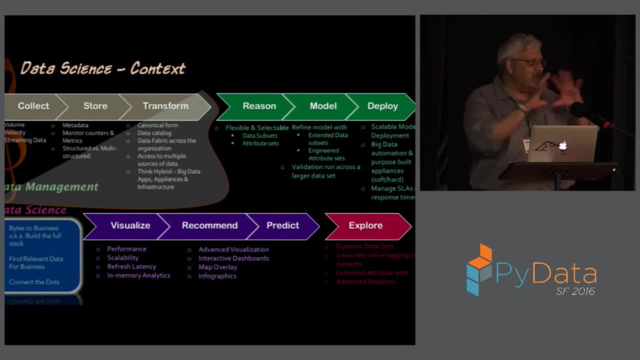 You have data coming in from multiple places. You want to take the data, you want to slice it, you want to change things around, you want to do various things. That is where the first thing comes in: The reason model and deploy. 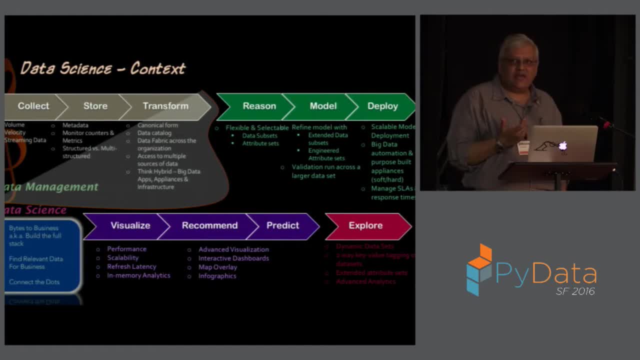 This is a machine learning part, That is a pure data science, where you look at the various parts of the data, you create a model And as iteratively you create the model, in the end you deploy the model right. So now your program, your machine learning, your model. 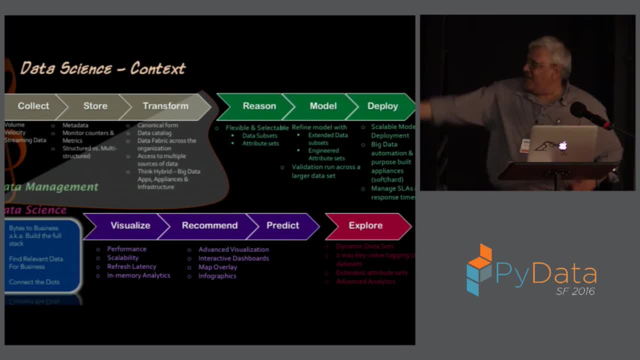 your AI thing is out there in the world Right, And then things like visualization recommend predict. those more are in the UI side right. The UI and the interactive. your application might have multiple things. So that is just the general of this thing. 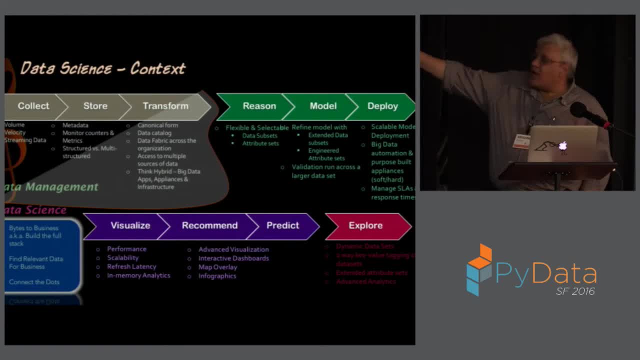 A lot of the work in pandas is in the transform and probably on the model right, Because when you have data, you want to look at the data, you want to look at multiple. we will do some of these things as we move forward. 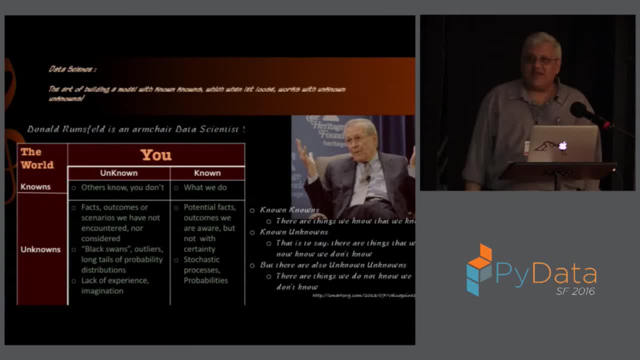 Couple of things, right? Don Rumsfeld probably is, you know, he's been doing a lot of research. He's been doing a lot of research. He's an arms data scientist, right? The key is this: When you do machine learning, when you do data, when you do these things right. 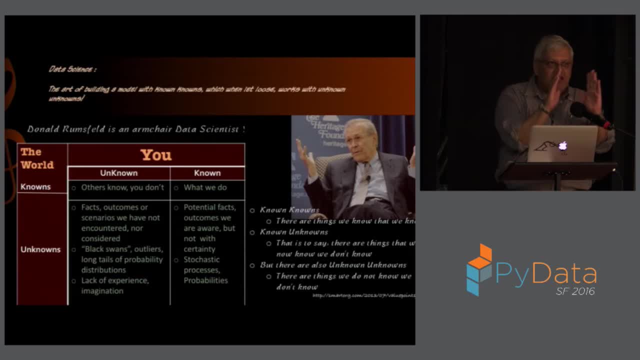 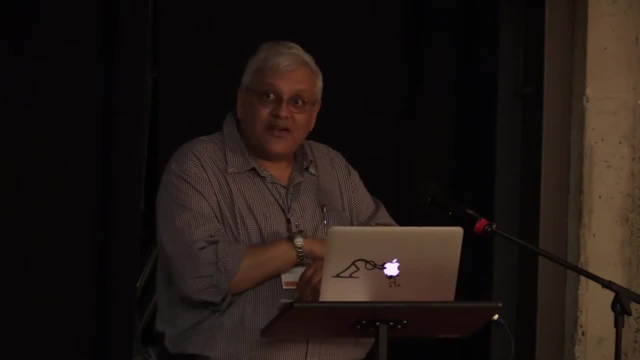 What you are getting. be very careful that what you are getting is a slice of the data, a snapshot of the data, right, And then you look at the data. So that is not the whole world, So be careful of that one. 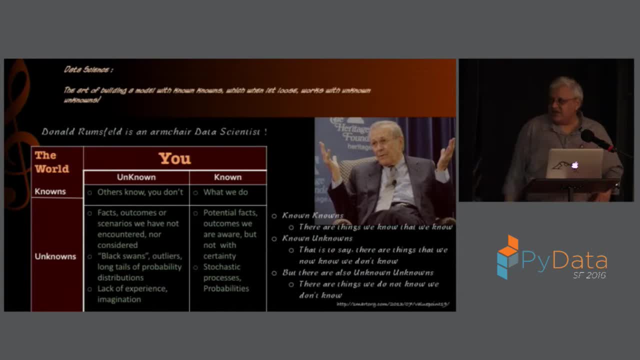 And so you might look at inference, for example. there is one thing that one of the data that we will look at- This is the. you know people click and buy pattern, right. So in that one it looks at it and says: we will give you like 33 million clicks, right. 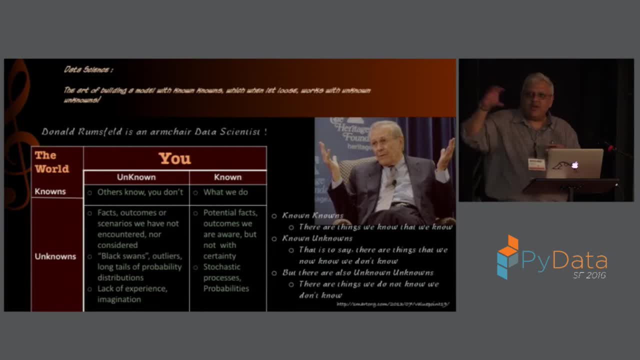 Tons of clicks. People click on all kinds of items And there is also a bias. And then they look at it and say, okay, now predict. Can you predict out of these clicks how many will buy Right When you look at it and say there might be, say like probably there might be, say 100,000. 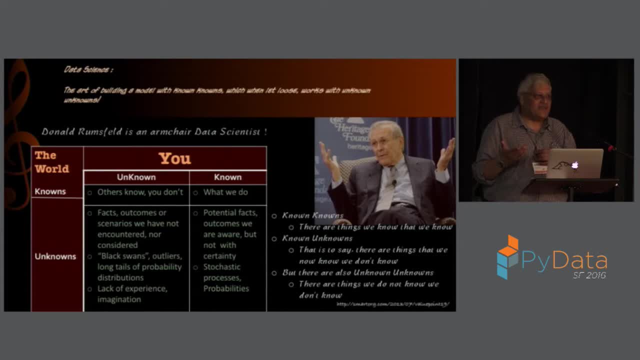 items And the bias might be only 20 or 30,000 items, Right. So from that one you can't assume that the rest of the 70,000 items nobody is going to buy. Remember, if you look at it and say if the data is from, say, March through September. 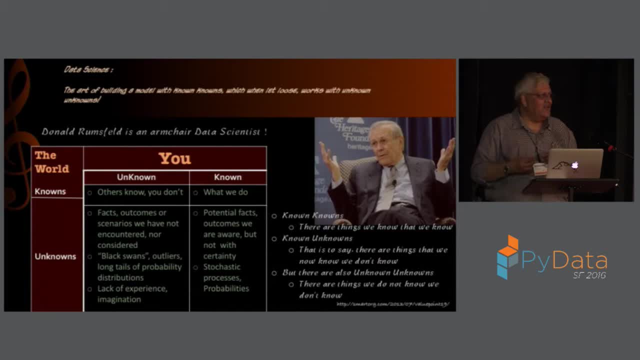 or something. and there might be items like Christmas ornaments right which people wouldn't buy unless and until you have the data from December. So the key is to make. so there are things that you know and there are things that you don't know. 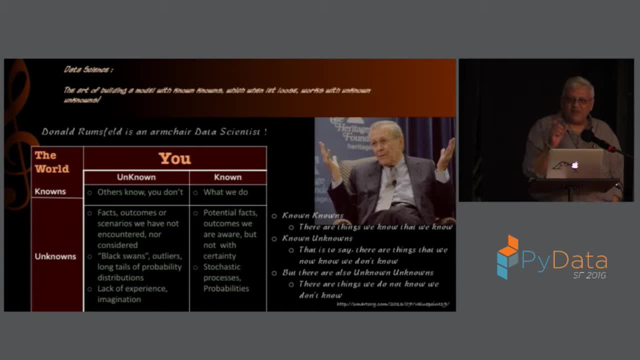 So keep, always keep that in mind when you look at the data, when you you know, especially when you're looking at averages, you're looking at various standard deviations, you're looking at various other things. you group by, et cetera, et cetera. 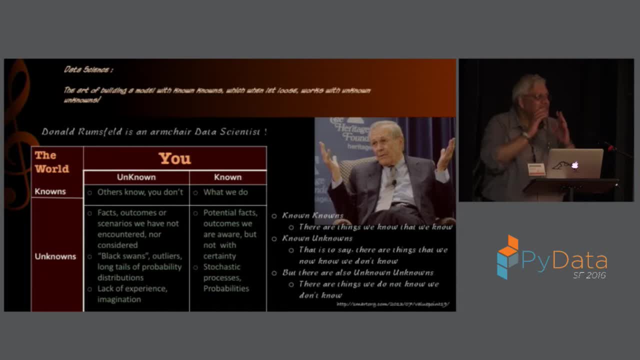 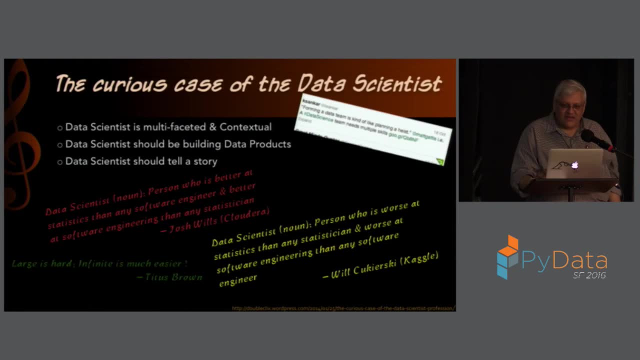 But make sure that the thing that- oh yeah, this is only a slice of the data there- is this huge world out there and things do change as well, So I just wanted to bring that up. I'll just pass on this one. 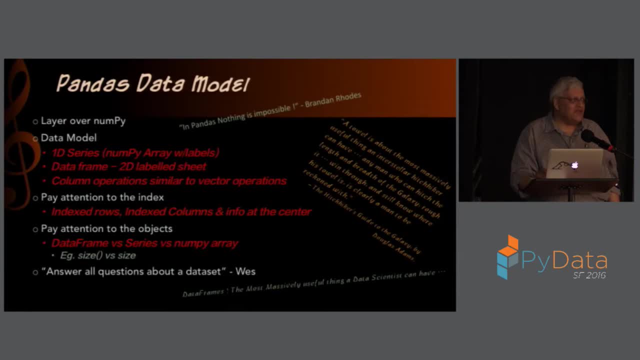 And let us quickly look at the APIs. right, the Pandas APIs. So the idea is probably you all know Pandas, but still, I just want to make sure that we have a. you know, everybody's familiar with Pandas. Okay, 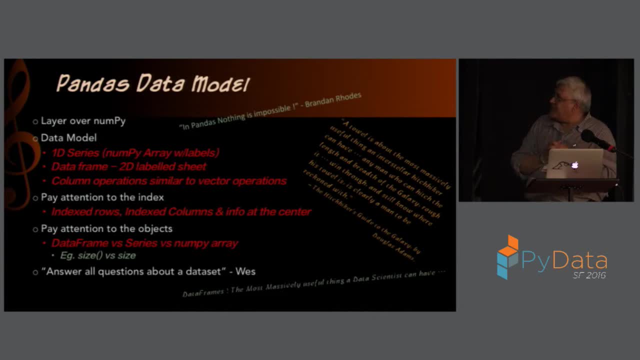 Pandas is on the same page. type of stuff, right, The Pandas first of all. the Pandas is a layer over NumPy, a very nice layer, but probably a slightly thicker layer with a lot of data. this thing right. 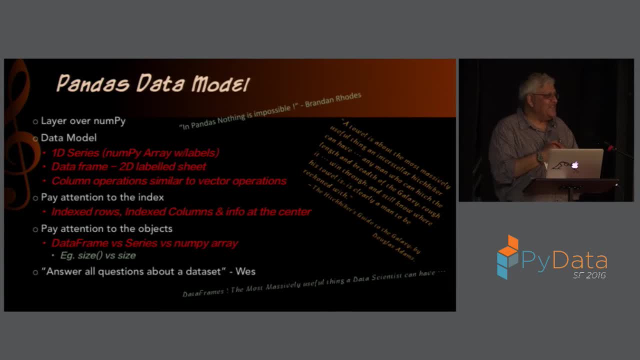 Brandon says. as Brandon says right, in Pandas nothing is impossible. So it's interesting this thing. right, You can do that, but you've got to figure out how to do it. There are two important data models, right. 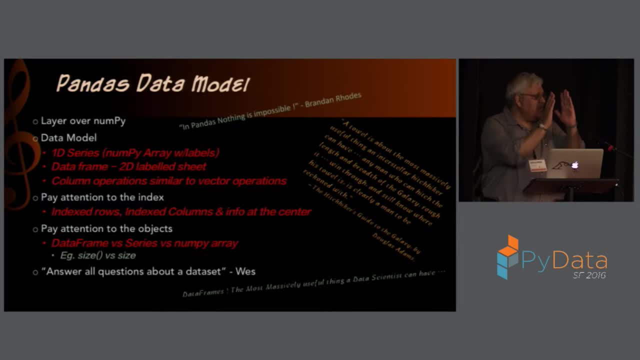 The series is a column. Series is a column and it is somewhat like a NumPy array. We will see that why, how it comes together. And the second data frame, Of course, data frame is the data scientist, you know the best tool. 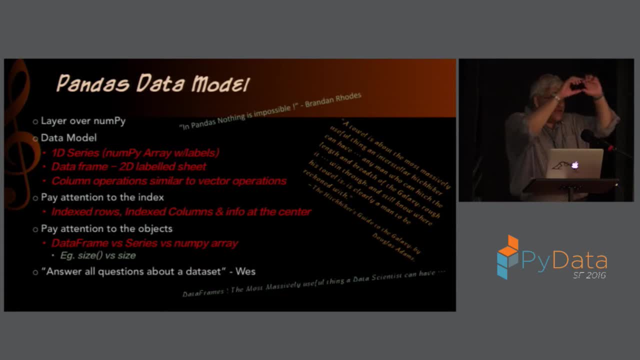 And data frame, of course, is a 2D. It is like a spreadsheet. It has columns and it has rows. The key one of the oh yeah. another interesting thing is you have operations like, for example, 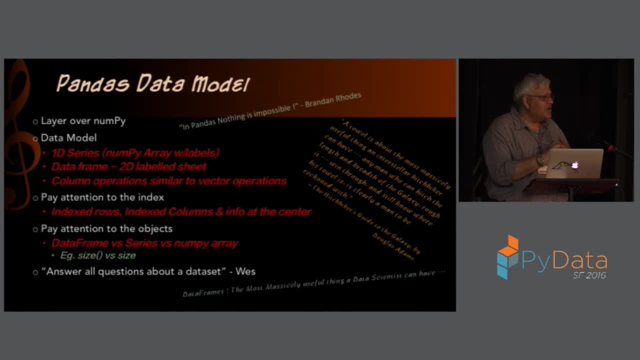 if you look at correlation, If you look at string, split various other things, right? Usually in Python these things act on one variable, right? If you give it a string and then say: split you, it split the string. 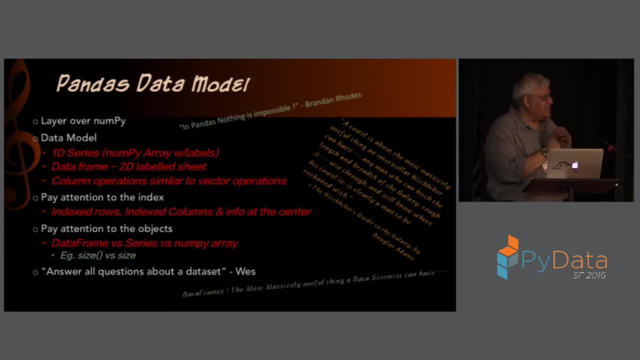 But they have extended it so that when you do a split on a data frame or a series, you get another huge column right. It splits each one of them. When you say correlation, it does the correlation. Or when you say covariance. 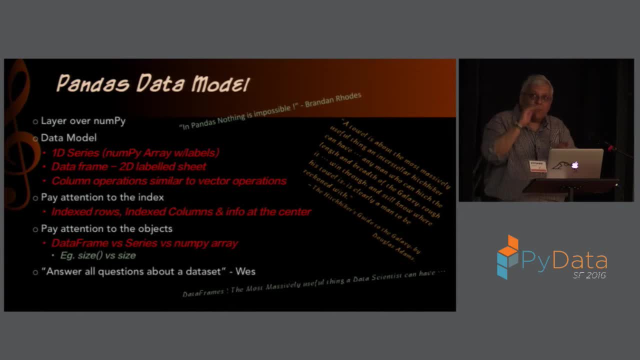 You'll see all those things. So when you say, right, So these functions act on a column or on a data frame, We will see how that comes together. Pay attention to the index: The way the pandas works. right. The pandas is not an array. 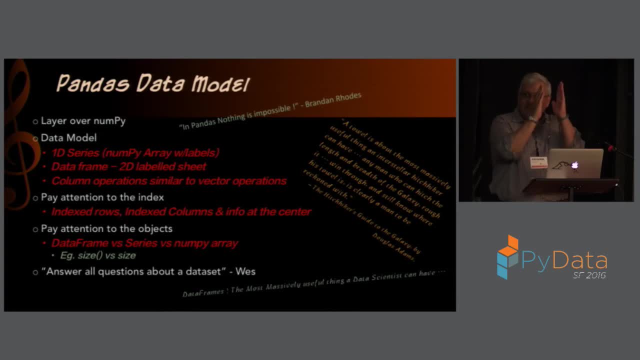 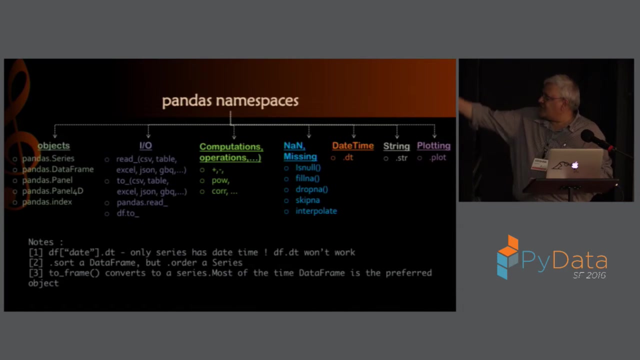 So you cannot just say: give me the zero, this thing. It is labeled rows and labeled columns. Keep that in mind. Again, we will see as we move forward. So that is. let me do one more slide, just to say the objects you have, the series objects. 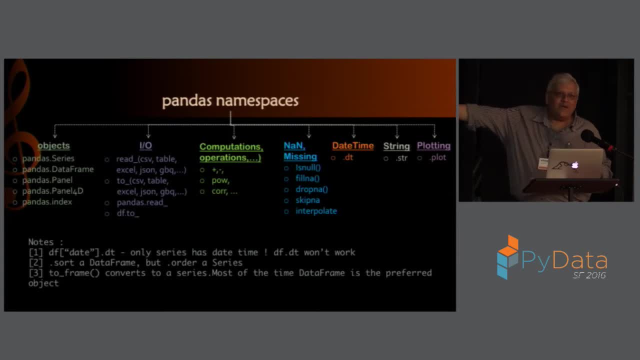 you have the data frame, the panel for the index. I'm using the index in one or a couple of places. Otherwise it is this: one IO is read, you know, you can. you know read CSV. you can read tables. you can read GBQ. 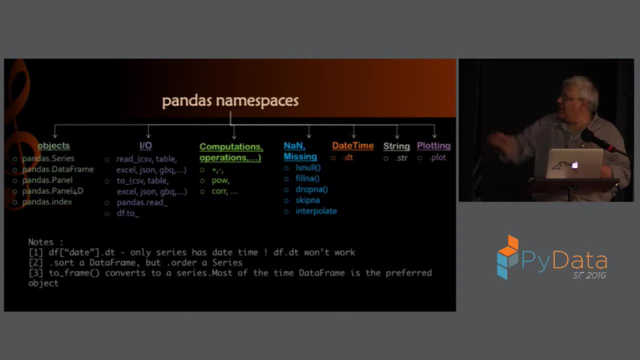 that is a Google BigQuery right GBQ. You can read any of those things You have. the computation NAN is interesting. Missing data: Again when we come to it, I will discuss more on the missing data, how that works out. 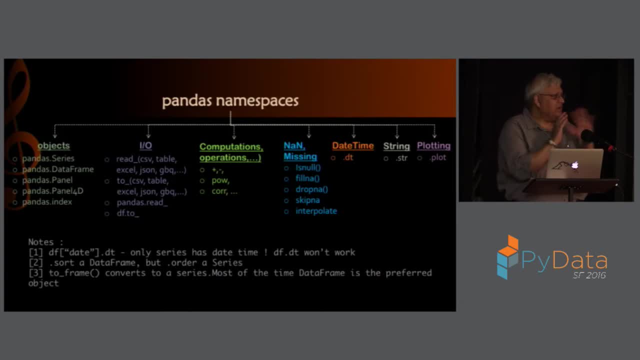 The whole date-time functions. a lot of date-time functions, right. You take the dates apart. All of these things are under the bt namespace, And then you have the str string operations and plot The reason this namespace is important, because when you are looking at something, you will. 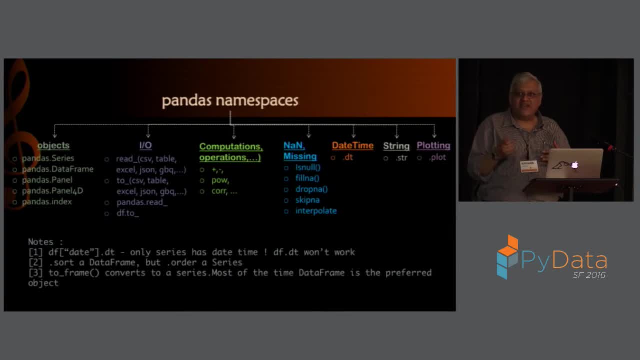 suddenly look at it and say maybe you will look at it and say data framesplit, But it won't work right? Then you look at it and say, mm-mm, what's going on? Then you look at it and say, oh yeah, split is you have the str namespace? 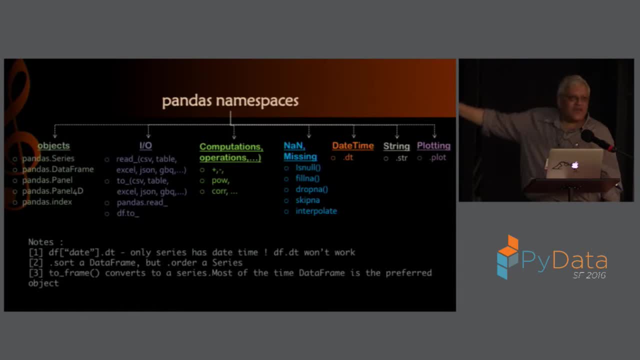 You look at it and say str, so dataframestrsplit. immediately it works. So it's easy to the namespace and how the APIs are organized. it's important to understand So that way you know where to find what This is. just a data site. 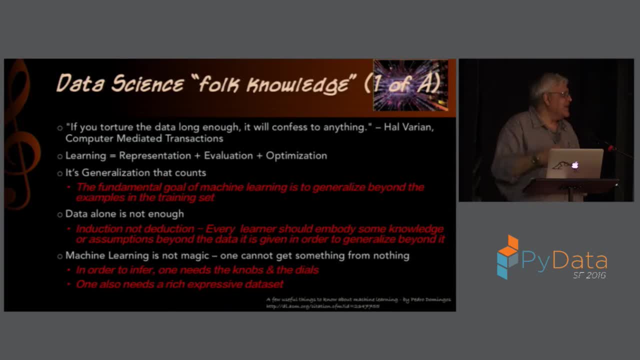 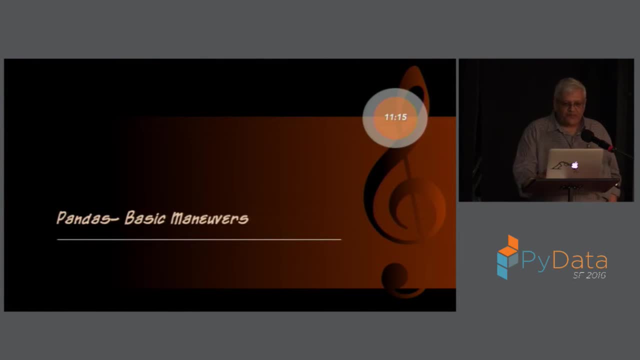 I have it in the slide so that you know when you know you can take a look at the slides. You will see some interesting things. You can think about it, that kind of stuff. So, without further ado, let us look at the basic maneuvers, right? 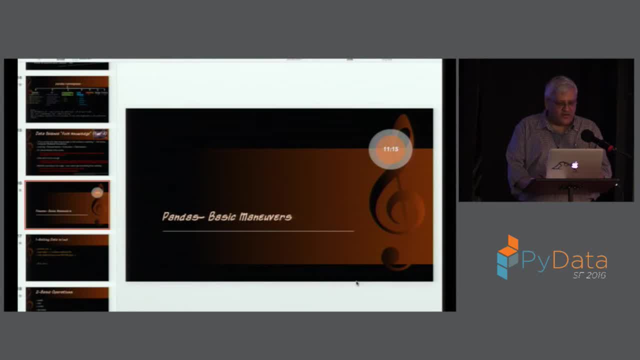 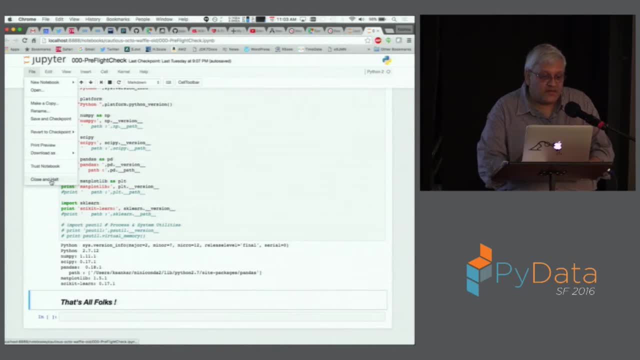 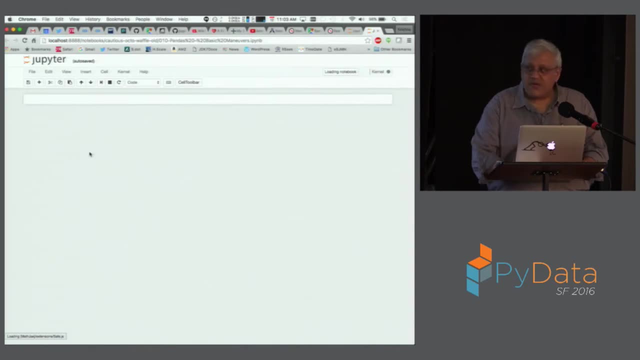 Basic maneuvers. We go back into the first. let us get rid of this person. We have the basic maneuvers, which is 0, 1, 0.. So now we have the basic maneuvers. We have the basic maneuvers. We have the basic maneuvers. 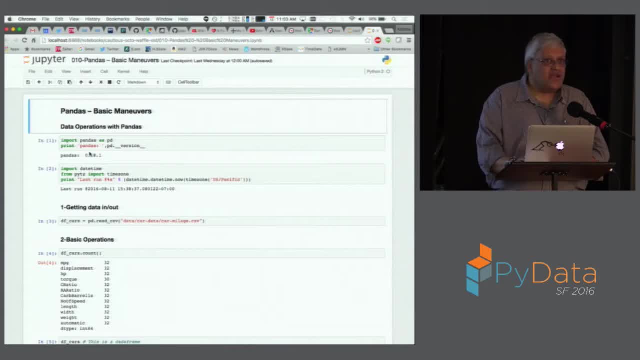 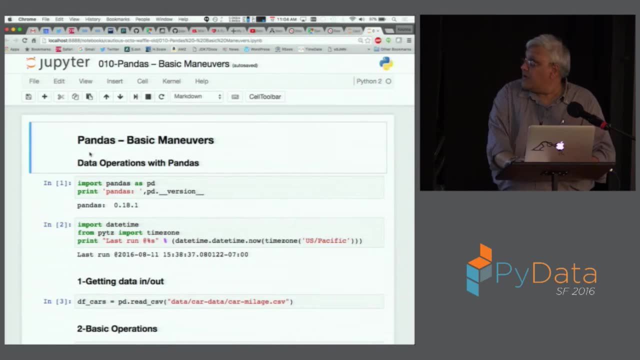 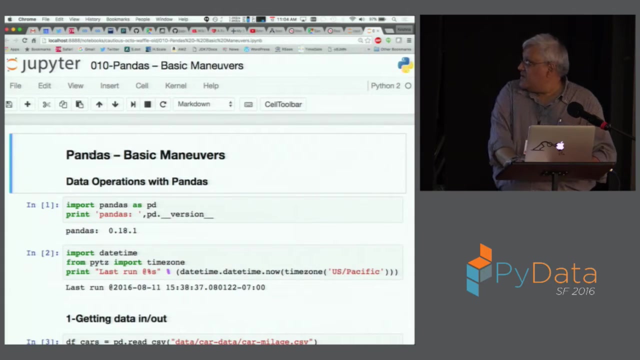 Let me see. I'm going to try command plus and if that works, it makes it easy for all of us to see How does it look. Is it good enough? Because if I do a more, ah okay, I'm going to hold it there. 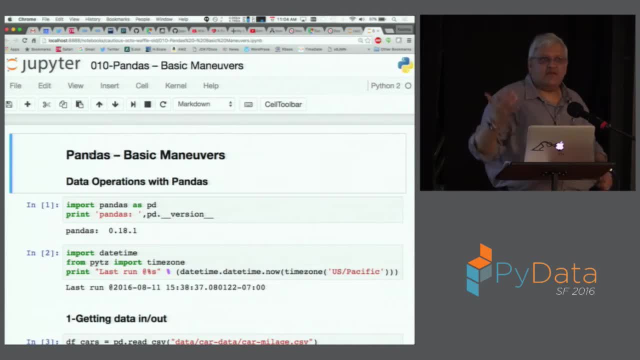 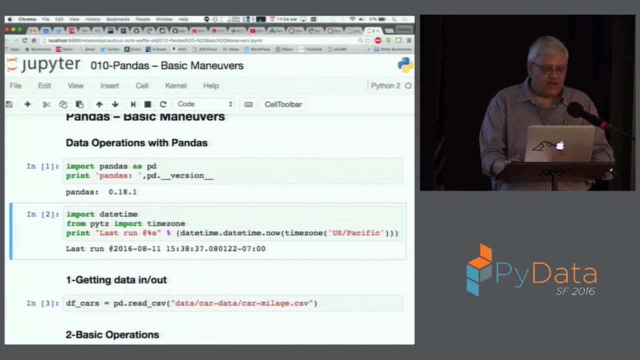 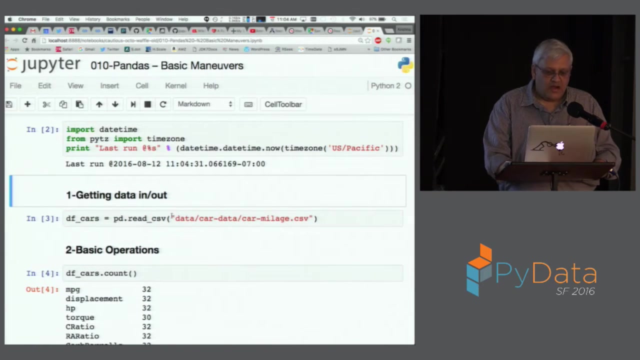 So you might see something cut off from the other sides, but still you can see that one, right, You can see from the back end here. okay, Yeah, fine, right, That's good. So first one, it's always, you know, you know, just to have a couple of this thing, datetime. 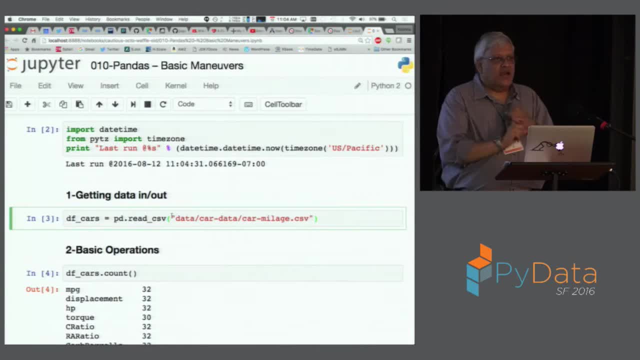 Item number one: right: Data in and out. Data in and out. it reads CSV, it reads delimited text files, all of these things. We have our data in a CSV file. So really, what we're going to do is we're going to, we're going to, we're going to. 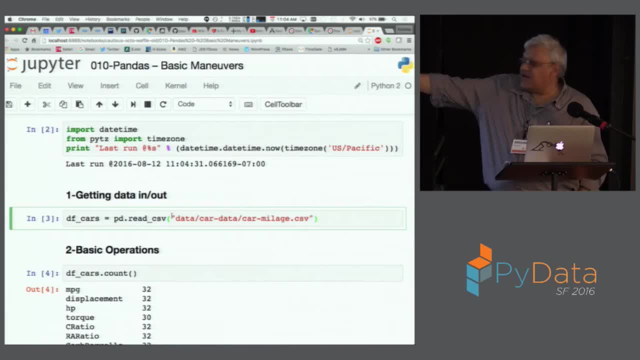 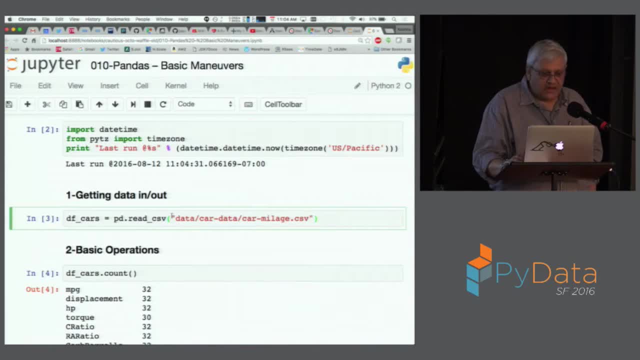 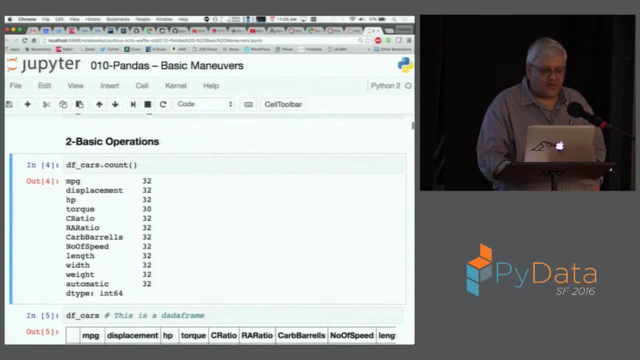 This is the car mileage data that we have. Let us look at what exactly is there. You read the data, the basic operations, right. The first thing you want to do when you get a data set, you want to look at it and say: 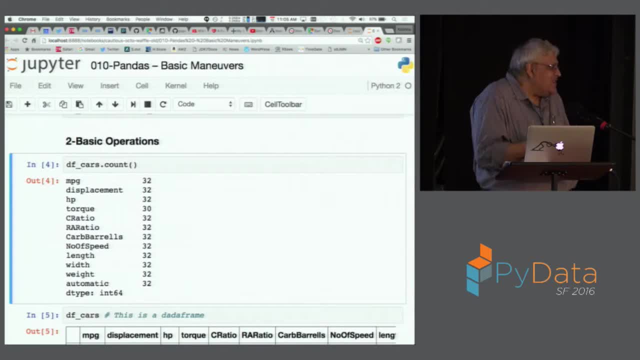 what? how many rows right, What, what? what is this data all about? You look at it and say yep, this is. there are 32 records in this one. Miles per gallon displacement torque, you know. RA ratio, rear axle ratio, carburetor balance. 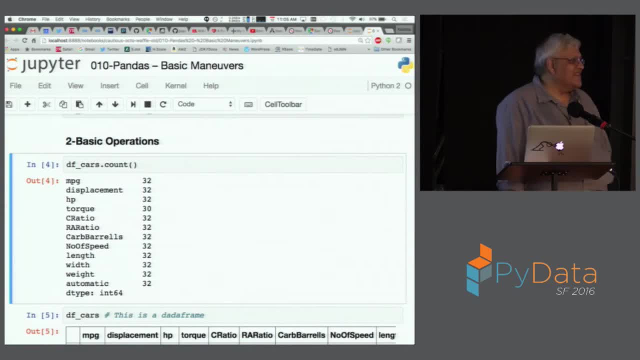 number, of speed, width, weight. You realize that. oh yeah, this is the car data set, which has a few attributes. right, Look at this guy. right, You see the torque somewhere there. Torque is 30 instead of 32.. You know why? 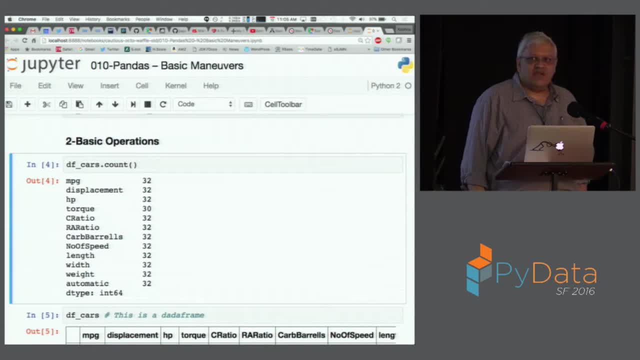 it is 30 instead of 32?? It is because NAN, right, Because for two items there is no torque in there. So we will see now. we will see how to handle these things And what do we do about it. So the other basic operation. 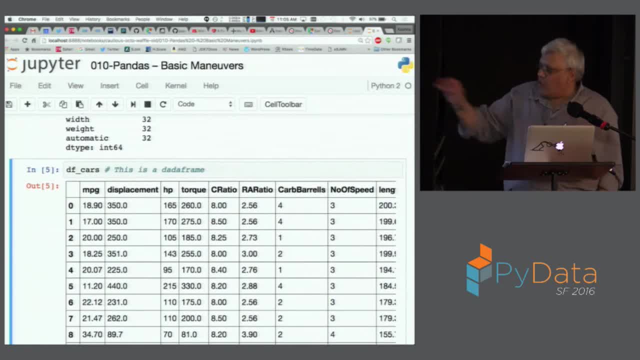 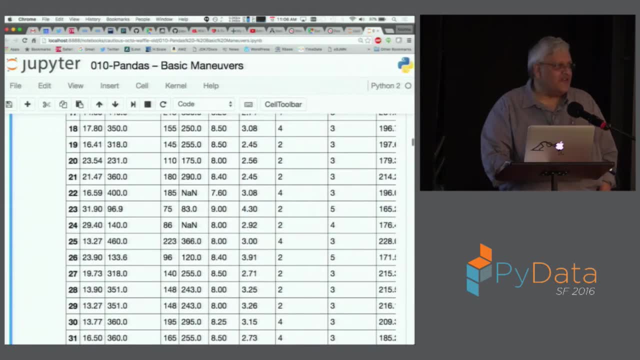 is you? just, if you type DF cars, it won't show the whole thing, It will show some part of it, right? Because this is only smaller data. otherwise, what it you know pandas- is enough. otherwise, if you have a record, 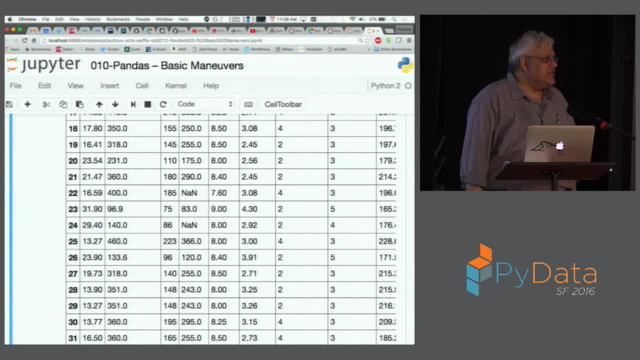 for example, by the time we get to the Rexes, it has like 33 million records. It's not going to display 33 million records here by that time. You know what it will do is it will show the first 20 and the last. 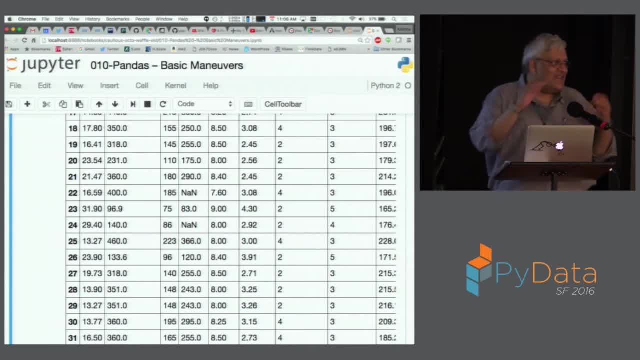 20 or something. Of course I'm not going to do this on that one, but still, that's what it will do. It knows enough and it looks at it and says, okay, let me show some. but you know, 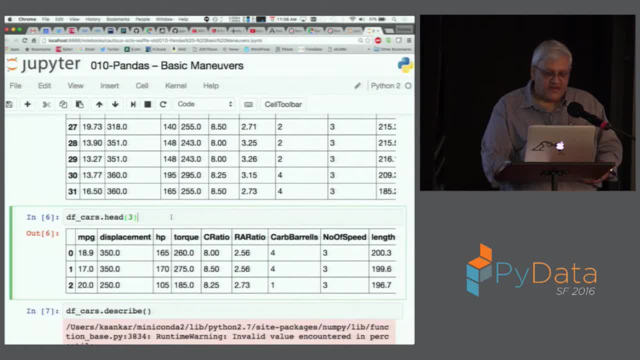 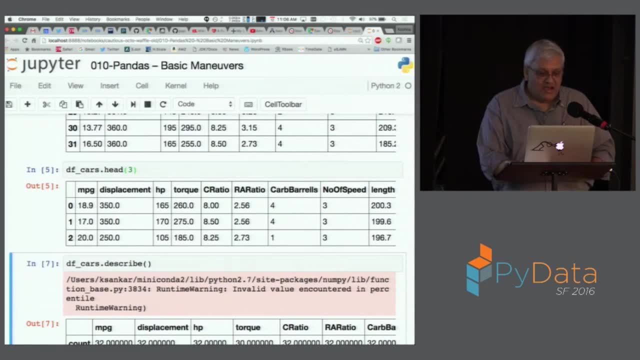 anyway, keep in mind. so it's okay, This is a, this is, this is a good one, right? You look at it and say: give me the head three, give me the top three, and let me take a look at it. There is another one. 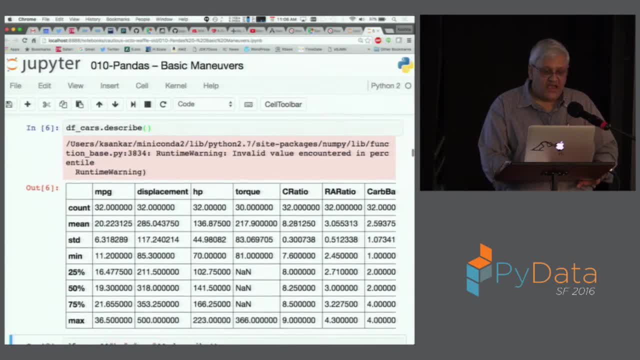 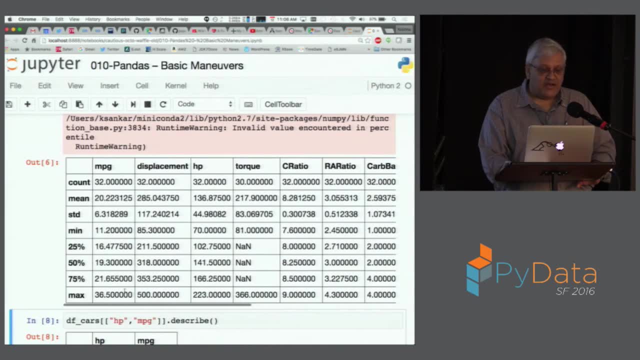 is describe, Describe, gives you the count, mean, standard, deviation, the quartiles, maximum right. So so now you can look at it, you get a feel for it. Oh yeah, there is this. miles per gallon, these are. 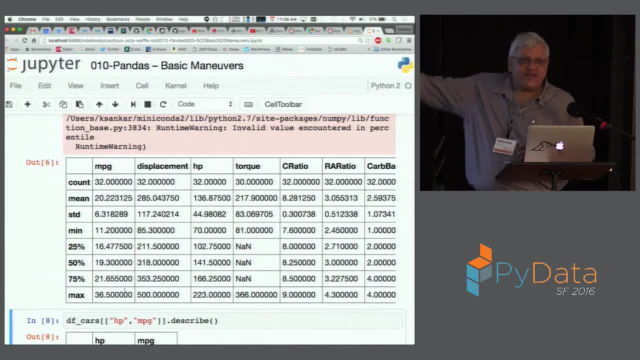 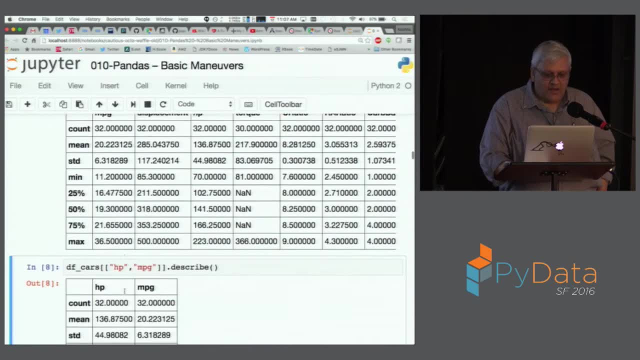 you know, these are the kind of things that is in there, et cetera, et cetera. So describe: gives you a quick snapshot, a nice snapshot that you can figure things out. By the way, if you, if you give, this is an interesting one, right. 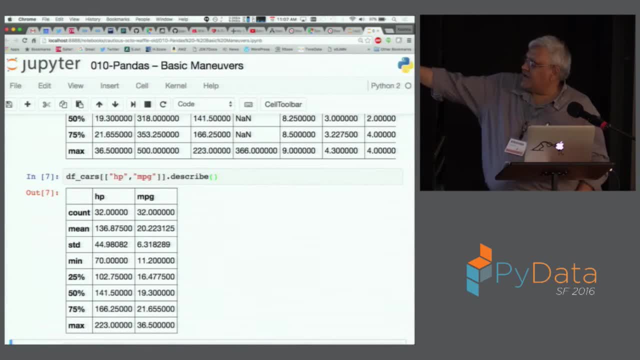 So when you do this right, when you you square bracket and you put those things in, you are giving a column label. When you give a column label, wherever it takes a column label, you can also give a list. So keep that in mind, right, So that? 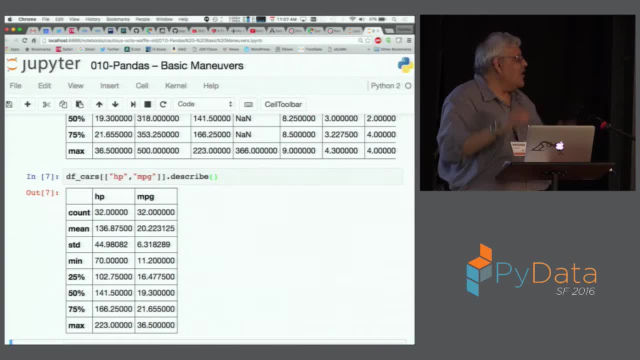 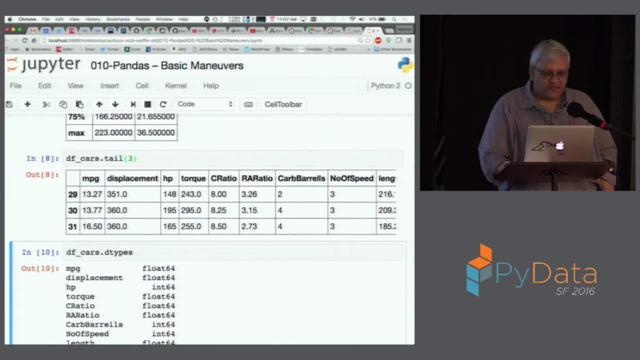 you can. you get multiple columns, you get a subset of the columns, you don't get all the columns. So you can do that: one, You have the. if you have the head, you have the tail, of course, Another. 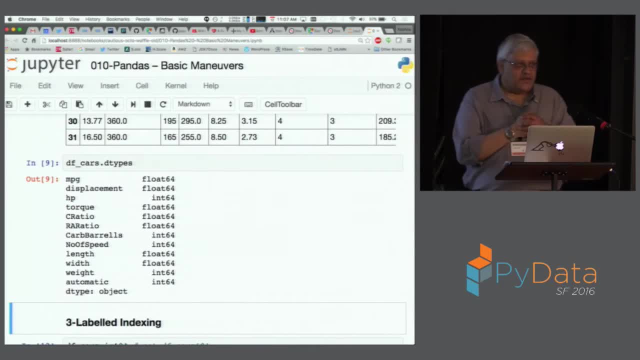 important one: dtypes right. Once you read some data, you also want to know what types they are right, Whether they are integers, date, et cetera, et cetera. So dtypes are important. So these are the. so if you look at dtypes, 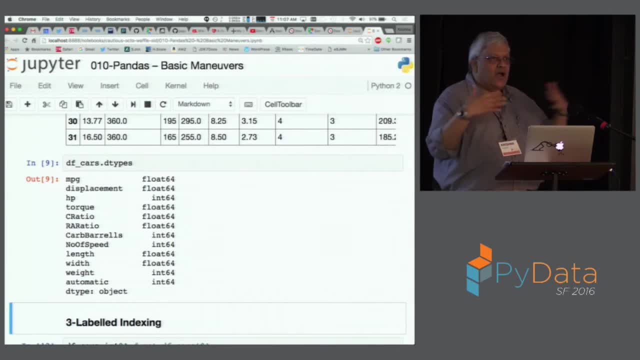 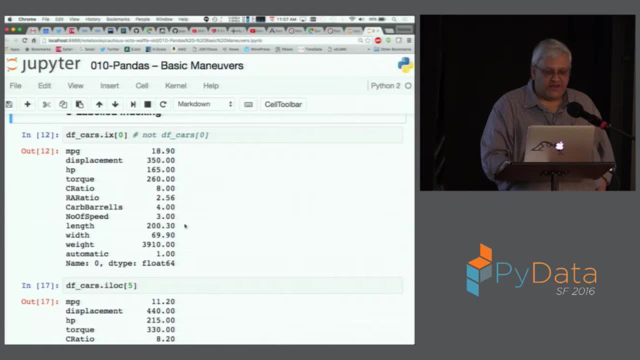 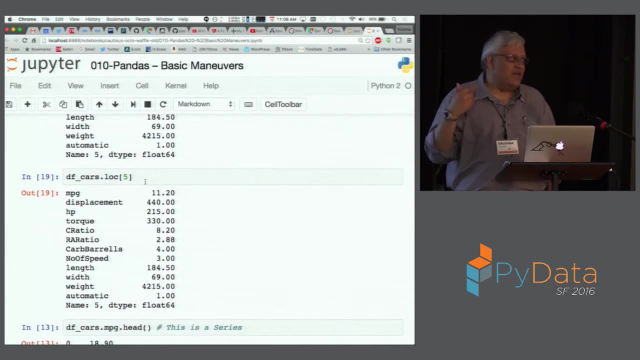 tail head describe. that gives you a feel for how these things are. The indexing: is the labeled indexing right? If you index zero, you get this one. We will. you know once we start indexing. we'll come back to the indexing, But the key is you can index. 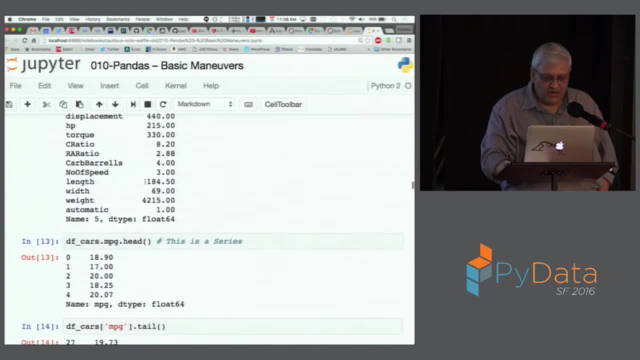 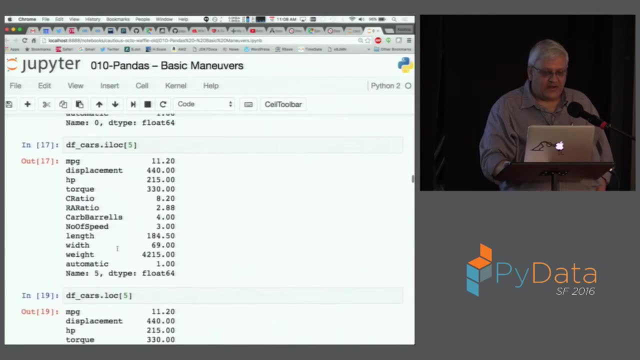 any row and say: give me that This guy Right. See, this one right. This is like this It is. you know, it doesn't look as interesting as this one Right When you do just the. give me the. 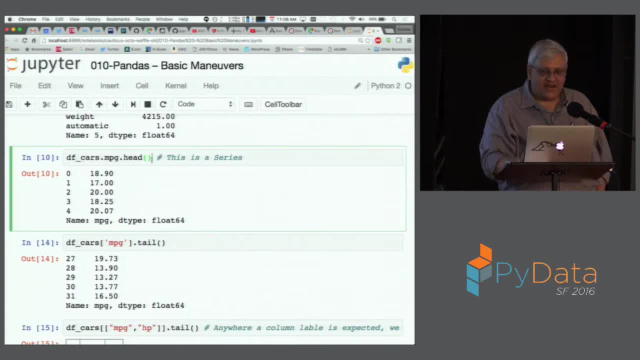 give me the. remember, carsmpghead, that we are taking one column. You know what this object is? right, That's a series object because it's a column. So this is what I was talking about. When you look at things, some things might be series, some things might be data frames. 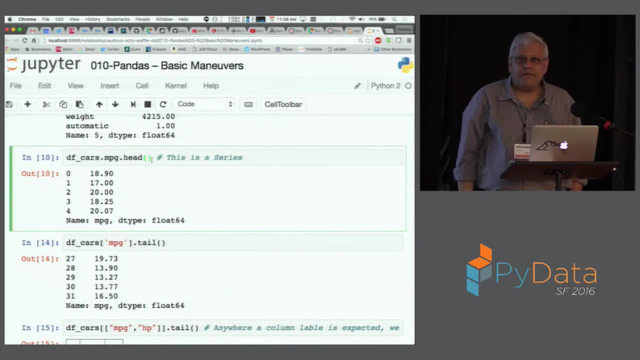 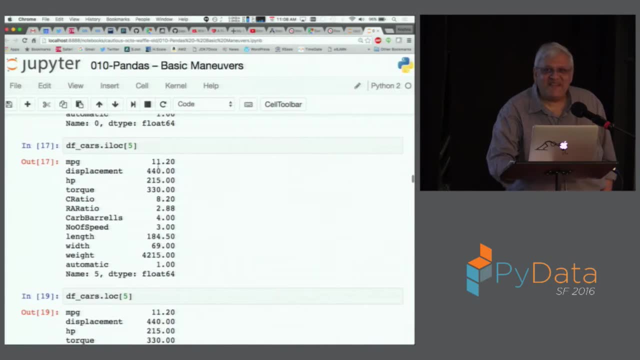 you have to keep an eye on both of them. Excellent, Excellent question. Excellent question, Thank you, I was skipping it. Yeah, yeah, So the question is: what is the difference between ILOC and LOC? Excellent question, Thank you. 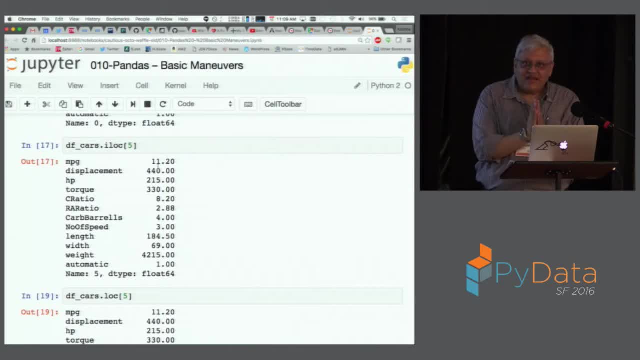 First of all, pandas is not an array Right. Pandas is not an array Right, So that you cannot just say zero It has. it has row. it is indexed by row row. it has row labels. it has column labels. Labels can be anything Right. 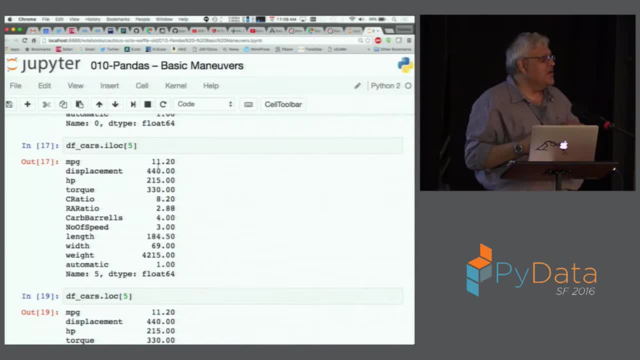 So in one of the things what Brandon was talking about, the label could be the. if you are taking the movie data set right, The label could be the movie name, So you can actually index it by the movie name. That is all fine. Now somebody says 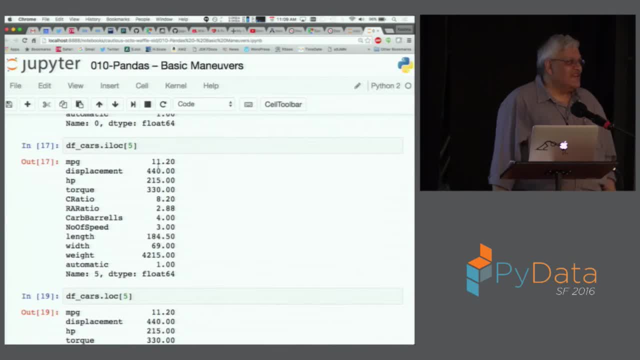 give me the fifth record. How would you do that? one ILOC, if I am correct, is it will give you the fifth record. But if you say LOC, it so happens that in our data, right in our data, in our data- 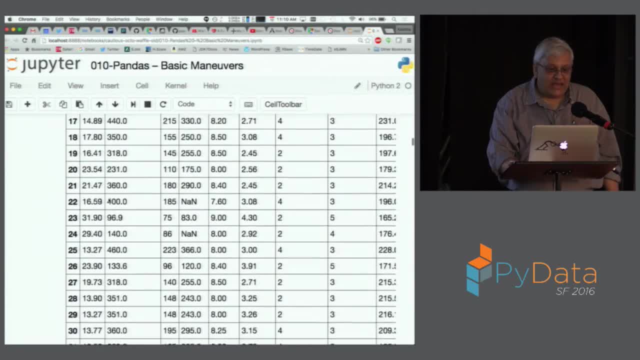 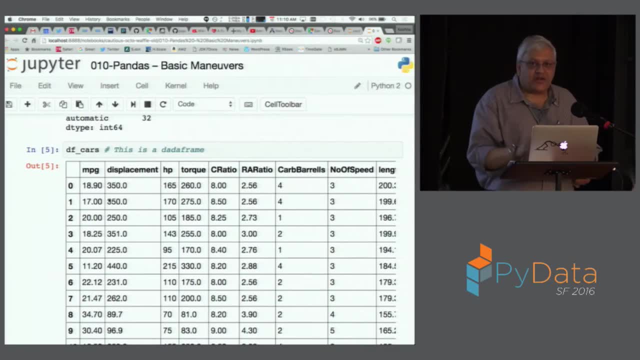 that is why see in our data, the index is the index and the number of the row is the same. But it need not be Tomorrow. you could move it and you can say: put the name of the car or something in there and then. 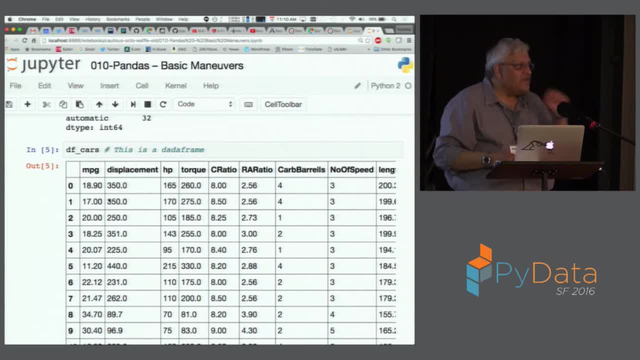 then when you do the fifth one in the, so ILOC gives you the fifth element, fifth row, But LOC gives you the row with the label it. it so happens that it is five, but it could be anything. 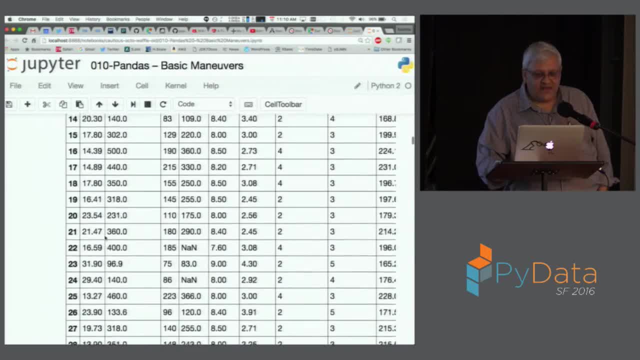 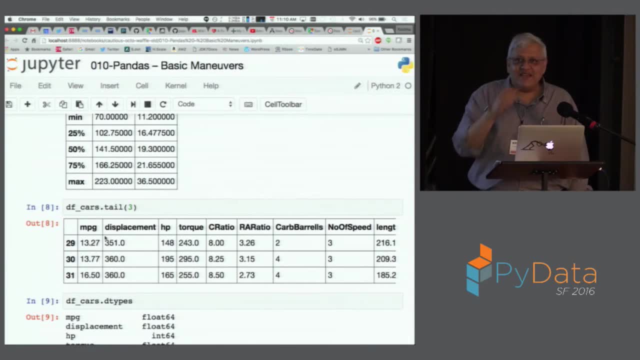 Does that make sense? So, anyway, that was the question. The question was: what difference? what is the difference between ILOC and LOC? Thank you, and this is exactly the reason I put that one in, so that you know it doesn't. 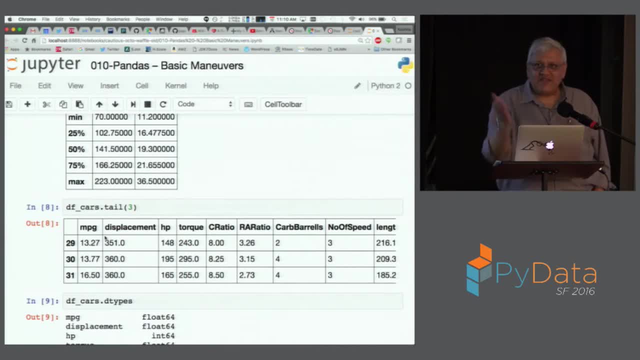 I said, oh yeah, So let me make sure that at least you get this thing out. This is the reason I was saying earlier, Two things are important. probably three things are important. right, I'll take the third one later, But the first one is the objects series versus. 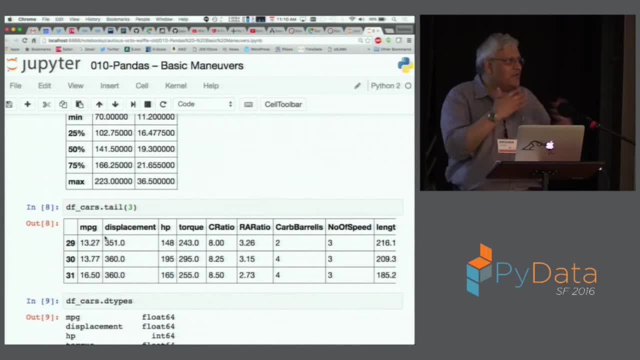 data frame. We will see that when we start looking at more data, we'll look at why is this thing happening. That's one, And the second is this indexing right. You want to make sure that you are able to index it. It is not. You can just go in and willy-nilly. 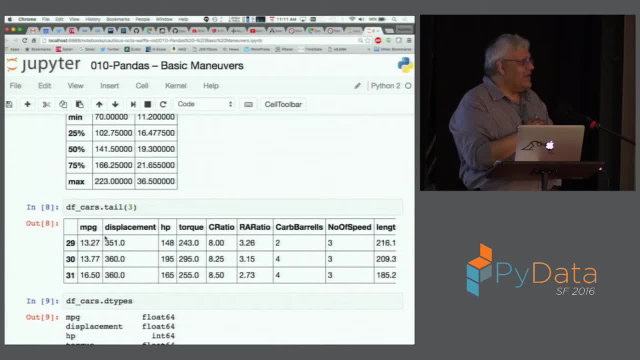 take something out And you don't want to right, Because if you have 33 million records sitting there, you can't handle one, two, three and you can't put it in here. You have to deal with it in aggregate. You want to deal all the columns and the data in aggregate. 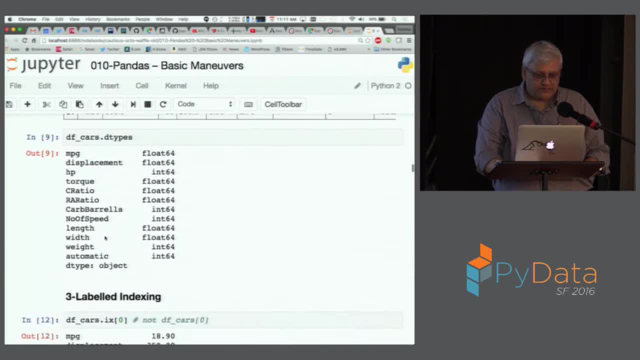 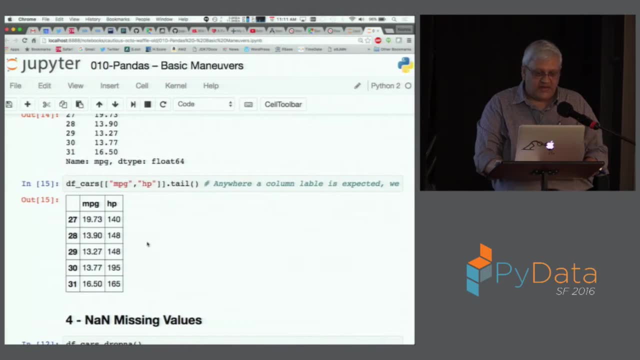 and you need to do things with it. So we went to the labeled indexing. Good, So then see this one. right, This is what I was talking about. right, You can index it by label. You can index it by column name, Wherever it takes column name. you can give a list of. 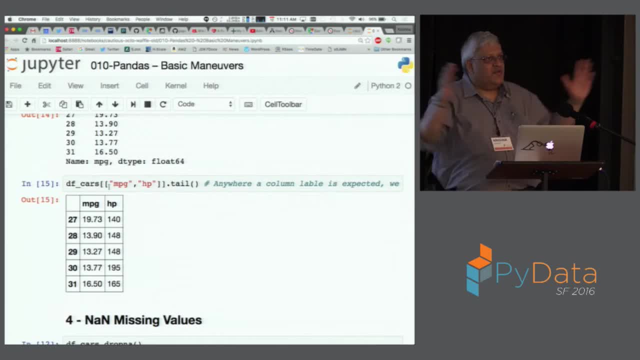 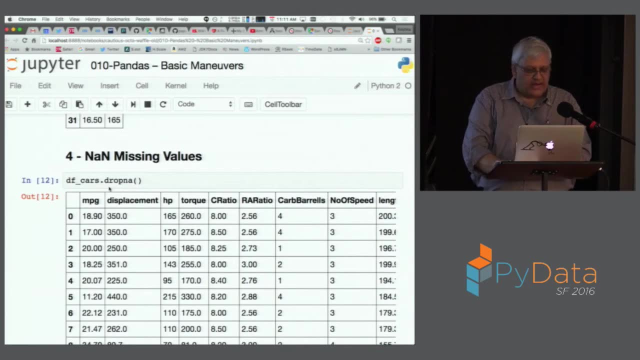 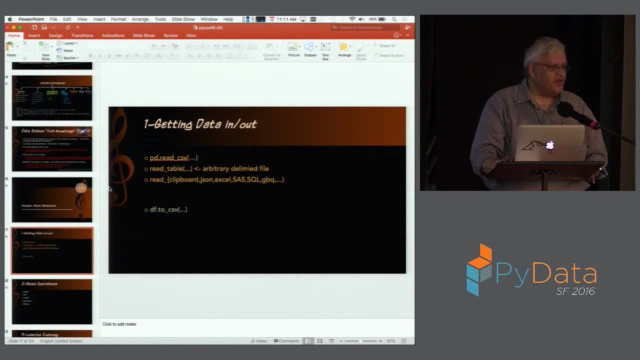 columns, so that then what happens is you get more than one column, So you get a subset of the columns. So now let us go into the one of the. so we went through this one right, Read in and out. You know that what you can read, what you can, you know This one: basic operations. 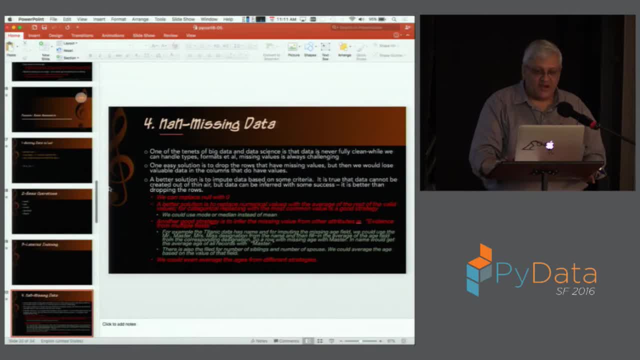 head, tail, We saw these things labeled indexing. That's what we were talking about just now. And then, remember, we were talking about the torque. for example, right When we did the count, we saw only 30 torque. 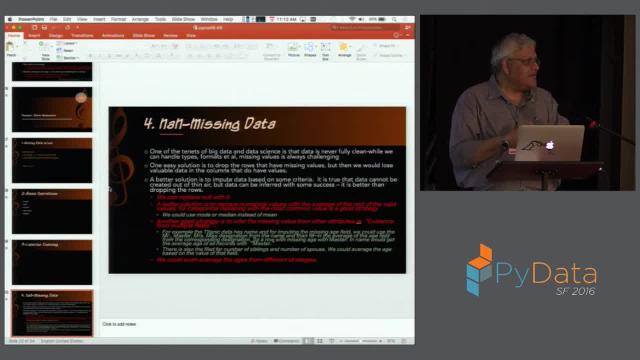 When you, as a data scientist, you know that they all data right. Data is not going to be clean, right You have. you are dealing with a lot of data. There might be data might be missing, Data format might be wrong, Somebody might not have entered the data. It's not. 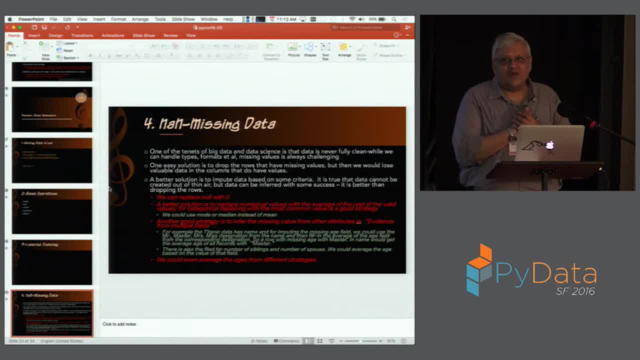 somebody entered the data. when you do the, you know, when you do the ETL, some pieces might not be there, that kind of stuff, right? So now suppose you want to model a you know dying habits of people, How do you handle it? right, You have, you have some pieces. 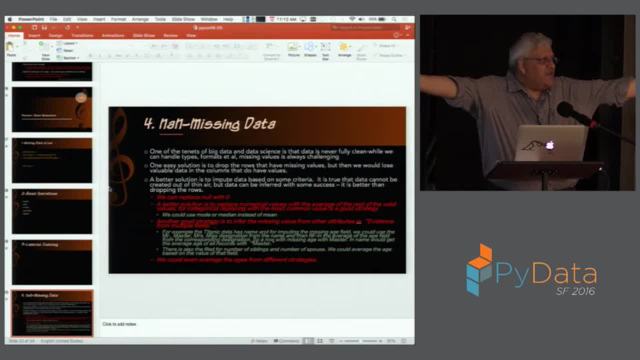 or you have, you have like 30 attributes or 50 attributes and some pieces are missing in various other places. What do you do with it? right? What is the most obvious way of doing missing data? Drop it, right, You right, That's what it is. Drop it, It's good You. 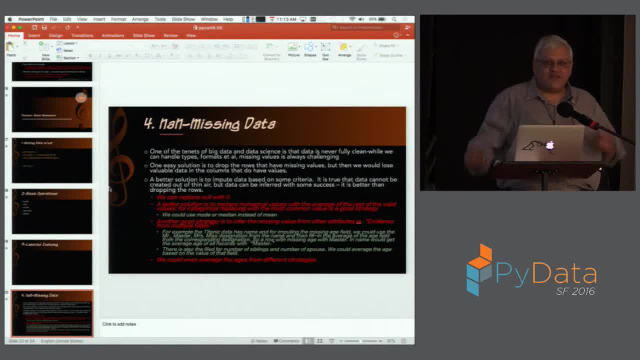 can drop it, but what is the problem That means? so suppose you have 30 attributes. one or two are missing here. one or two are missing here. one or two are missing here. When you start dropping, what happens? By the time you start dropping it, a lot of your 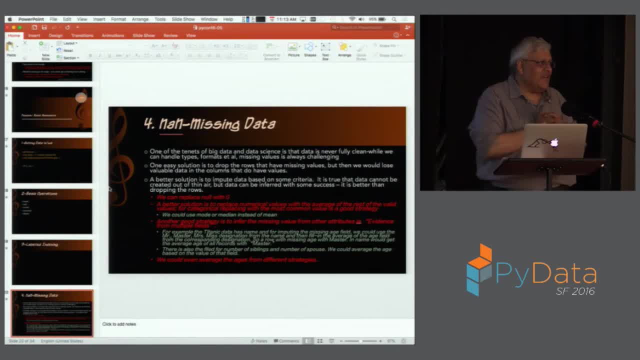 data is gone, right, Because it it kind of fine. So then what is the next best alternative? Impute- Thank you right- And impute data right Now. the question is: that's fine, So what you are going to do is, for the pieces of data that you have, you want to put things. 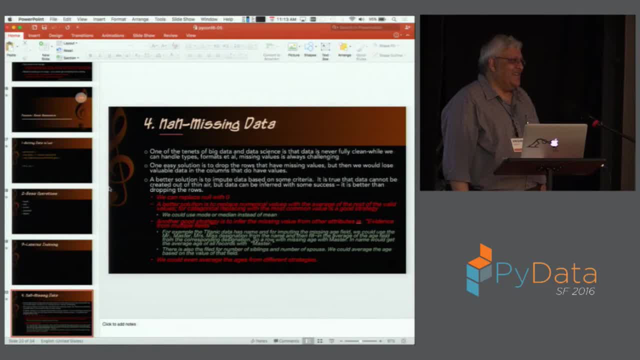 in it. It is good, Excellent. So then, what do you put in there? Yes, Thank you, No, no, no, go ahead, go ahead. I was just thinking about imputation. Yeah, yeah, Excellent, excellent, Thank you. Thank you, Because imputation itself is bigger. 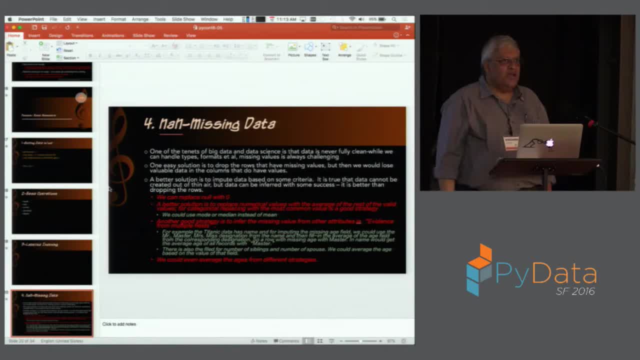 You can do mean, right, You can do mean Mean is fine. but then it might not be right If the the mean almost assumes a normal distribution of the data. right, That's why you are putting in mean. But your data might not be normal distributed, Just for example, right, You might have say: 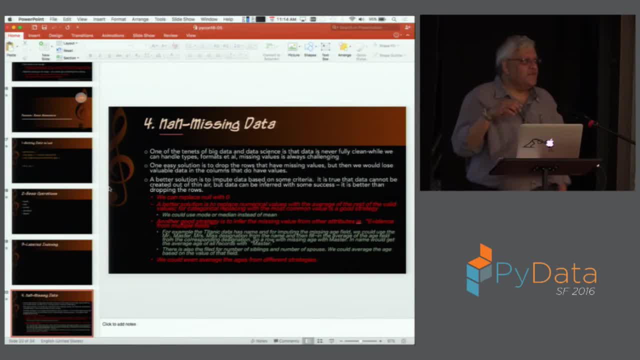 for example, you are looking at some readings for, say, health reasons, right. So if, for sick patients, what might happen is the readings are high, right. And if, for example, you know very rare diseases, 99% of the data will be, you know, won't be, won't be high. 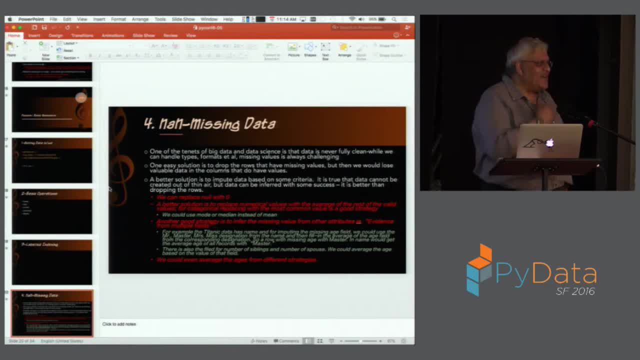 and only a few of them will be right. So now, if you put the mean, what happens? All of them. you are putting all of them in. You are putting all of them as healthy people. That's not right. So what you have to look. 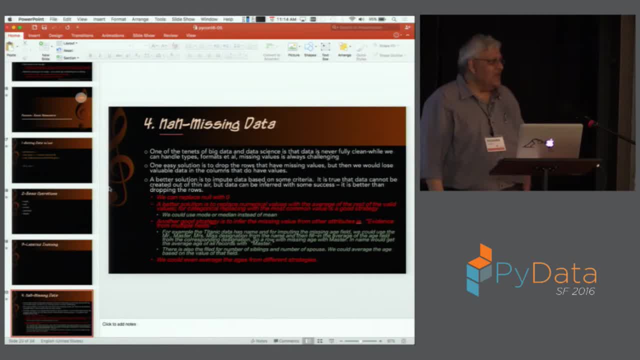 at actually is look at and say: I have this data 99.95% of the time. this value is between 10 and 30. And probably come on in guys, Come on in, Sit down, Let's go. So 99% of. 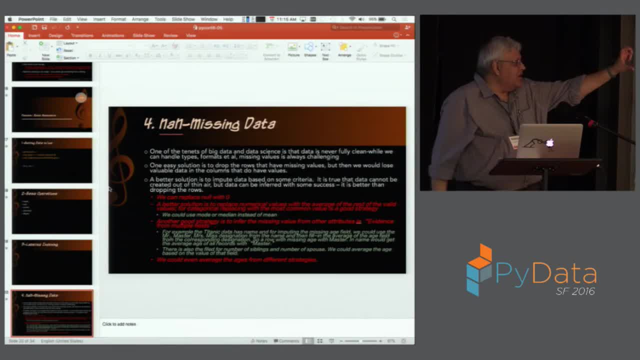 the time. you know, 99.5% of the time it is between 10 and 30. But 0.5% of the time it is 120, right? So now this particular field- you have about 500, say 100- data is. 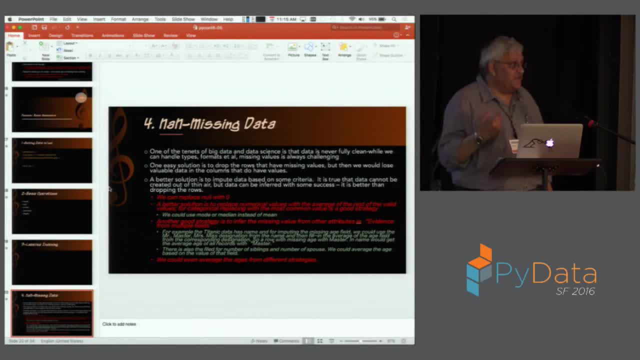 missing. So if 100 data is missing, you are not going to put everything as 15.. You have to look at it and say 95 of them are, say, between 10 and 30. So you have to do some. 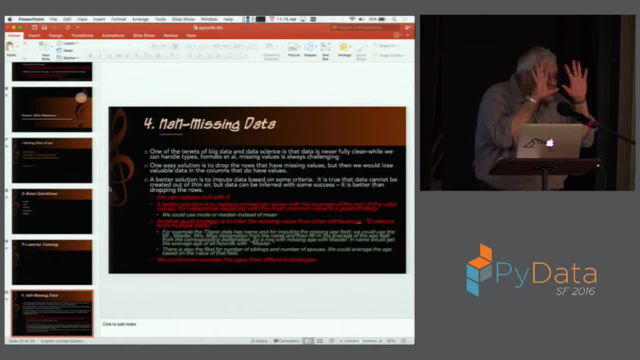 random this thing and say 10,, 20,, 22,, 23,, 50. And then 5% of it you do have to put like 100,, 110,, 120, et cetera. So you know, so there are. it gets more and more interesting. 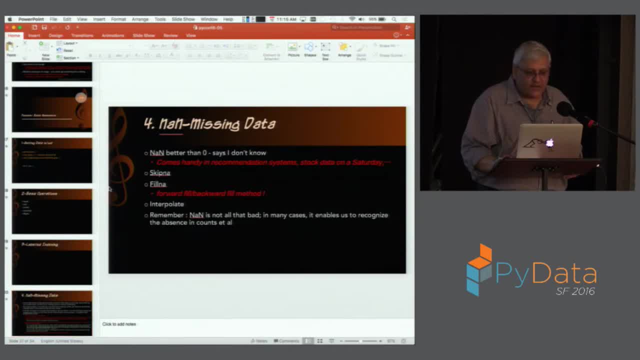 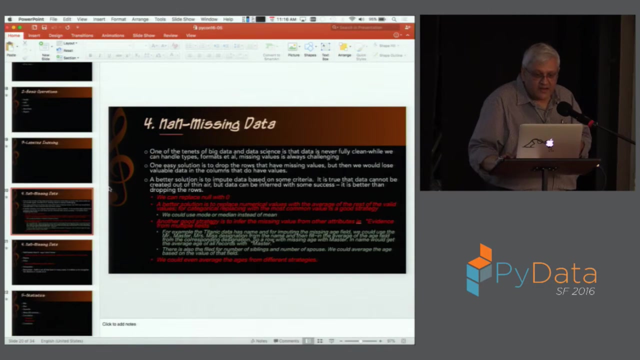 We'll go deep into it. There is also another story, NAN, right? Yes, sir, Yeah, yeah, yeah, It's a. so we have the East Null. So the the excellent question. let me go back, And I had it somewhere here. Anyway, the East Null is the one to figure out. We. 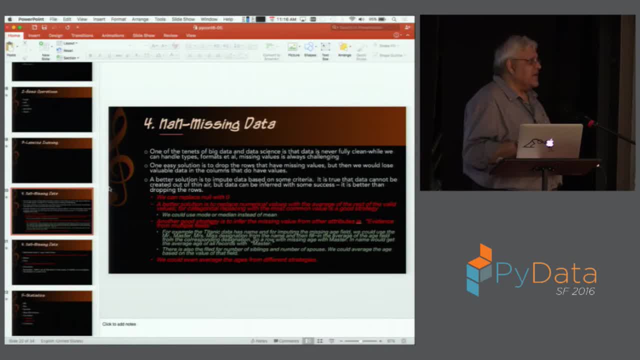 will, we will, we will do it. We will do that one here as well, Right? So because, remember, you have to look at it and say, East Null, I'll show it. We have this one, East Null, in this column And you. 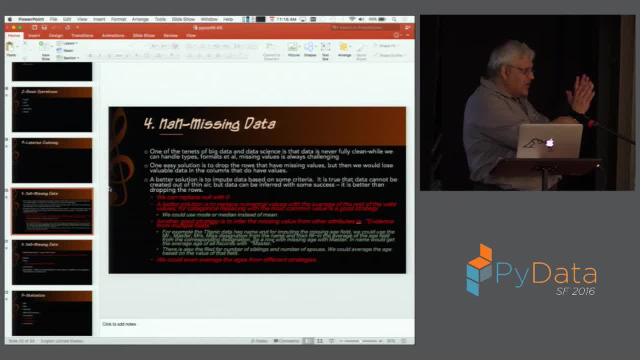 can do many things. You can say East Null, You can pull the, you can pull actually the rows out. You can do many things with that one. No, no, But remember each column is: this is a heterogeneous thing, right? So you cannot. 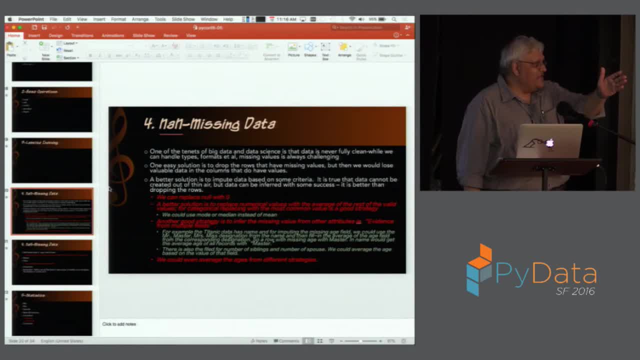 you know the average of age. you can't do that, You can't do that, You can't do that. The average of age is not the same as average of fare or something else. So, yes, you can do East Null and it will give you the whole thing, But you have to treat it, you know. 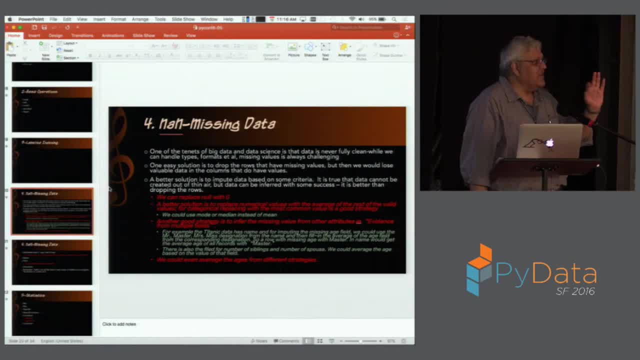 column by column, And and if you want to do it, you have to go surgically and say this column is age. So I'm going to take an average age. This column is something else. I'm going to look at it And there might be categorical columns for that matter, So that 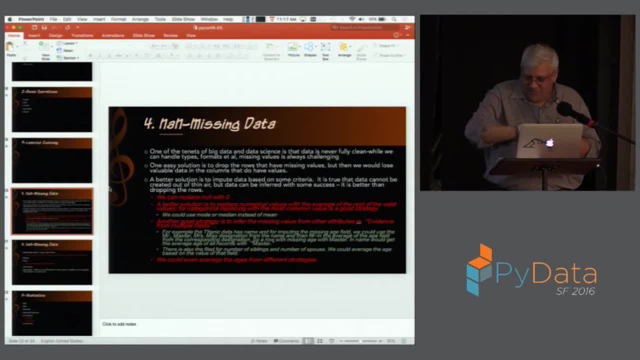 is why you know, thank you. It's an interesting discussion. I hope you know we'll sit through the lunch and maybe the dinner as well, But you know it's, it's, it's, it's, it's, it's. 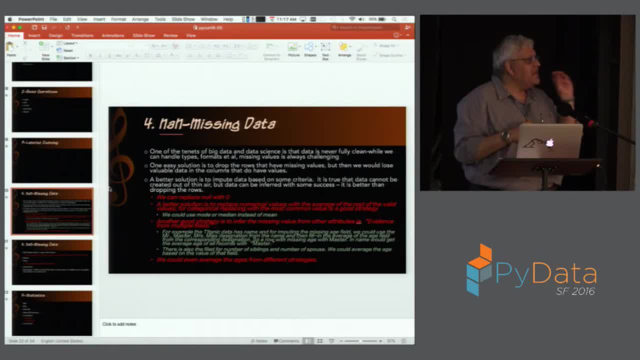 you know, which is fine, Because the NA is an important one. This is one of the, this is one of the interesting ones, and and PANDAS helps a lot on that. What I mean- it helps a lot- means it has six. 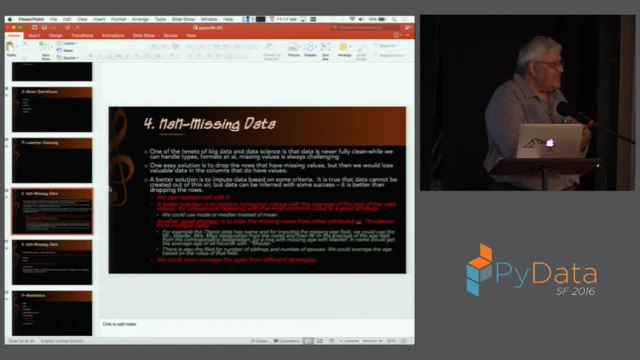 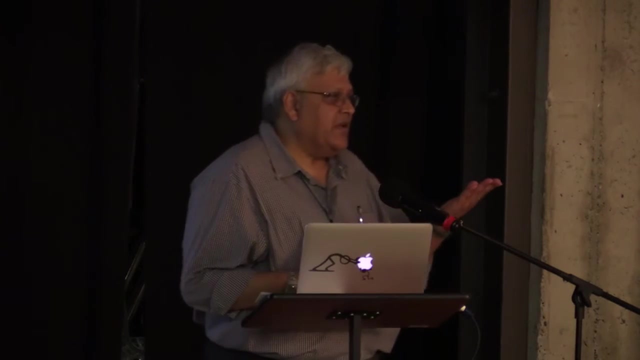 or seven functions. that's the best it can do. Does that make sense? Female Speaker 7. Hmm, Female Speaker 8. Absolutely, absolutely, Yeah, yeah, yeah. So even though Pandas gives you only six primitives, Panda doesn't give you all those things. 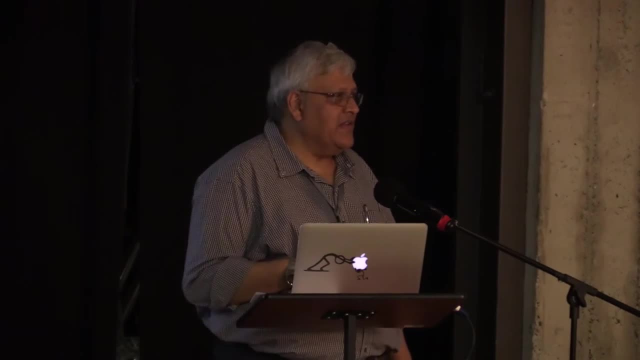 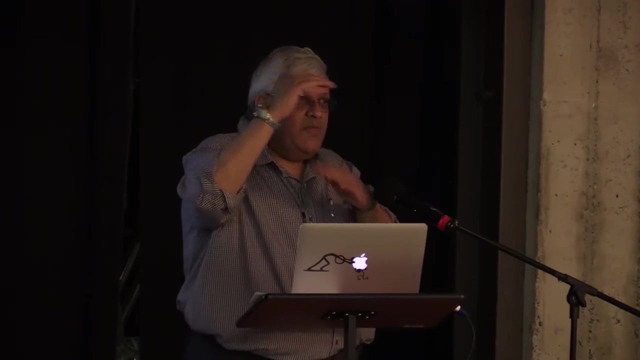 So, for example, the Titanic data that we will see a lot of age is missing. So either you can put the age as average age or you can look at it and say Mrs, Miss Junior, et cetera, and then say what is the average age of Mrs? 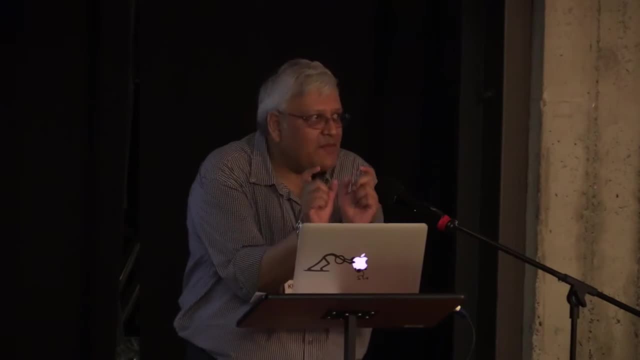 which is a name in there, right? So I look at Mrs and Miss and Miss and Master and that kind of stuff and look at what is the average age and then, based on that one, I can actually impute ages there. 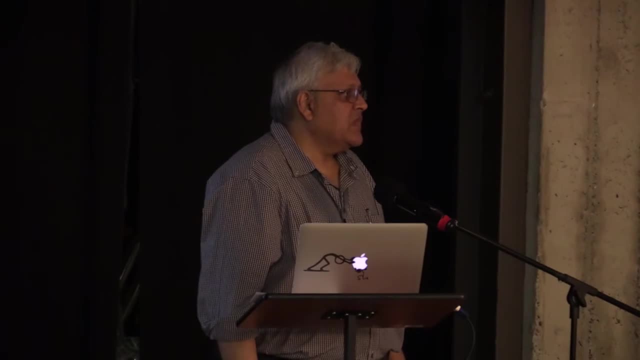 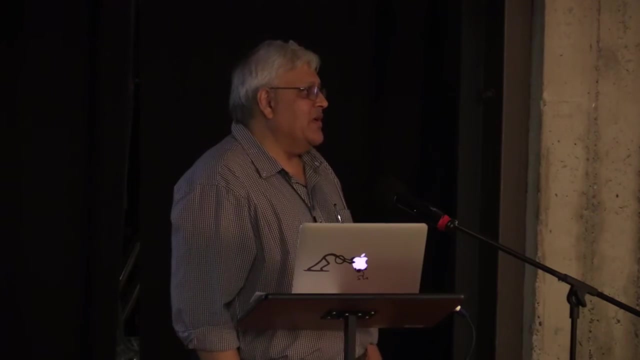 Yeah, Something like property and the other. is that an in-place modification or is the property returning a new? So you have an in-place equal to true. You have an in-place equal to true. If you do in-place equal to true. 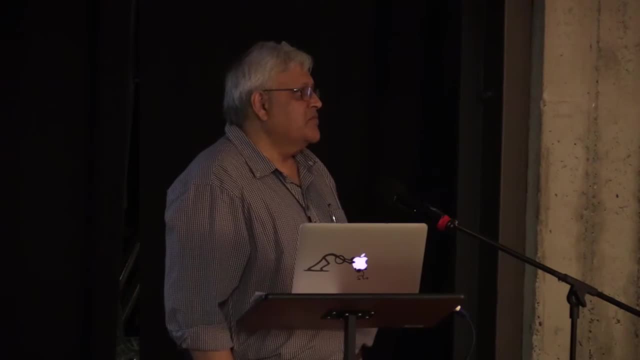 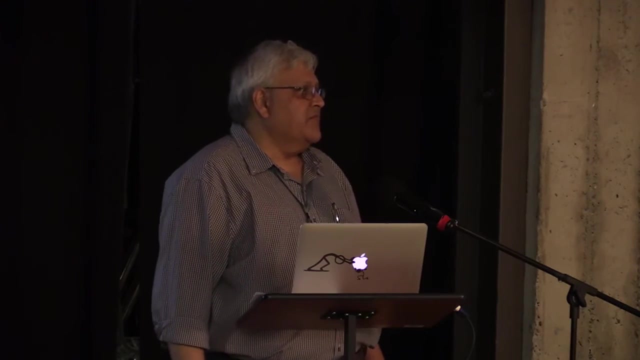 it will go and change that one, Otherwise it will return a different one. Yeah, in fact, in-place equal to true is there in many of the other transformations as well. By the way, just to give you this thing. I also you know I'm writing a book on Spark. 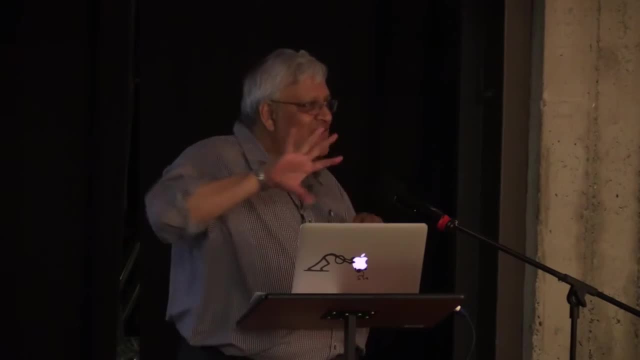 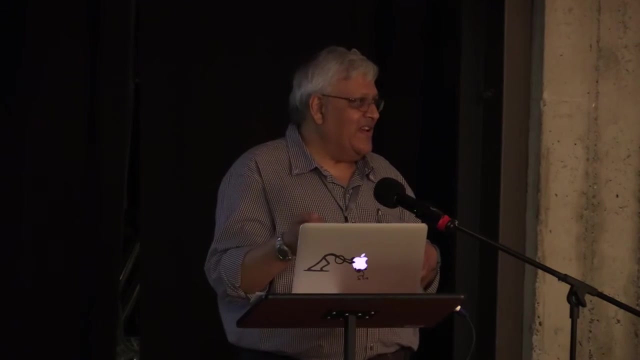 Apache Spark and that kind of stuff, right. So there are like that's an interesting. So if you use Apache Spark, for example, the APIs are very similar. So the data wrangling that I do here I have also on the Apache Spark as well. 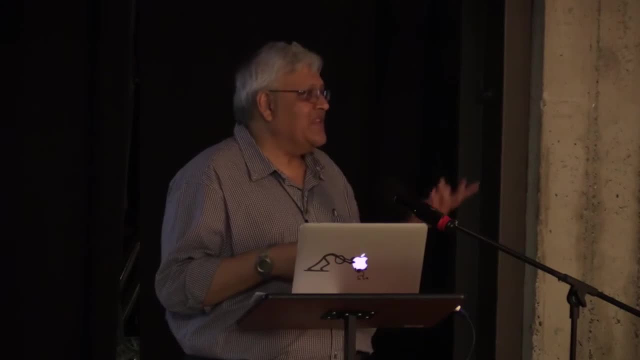 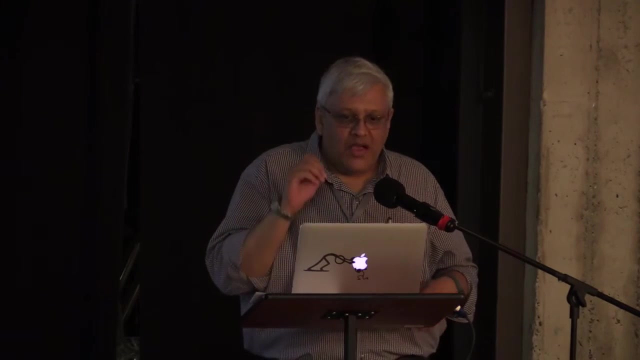 So it's an interesting one, but there it always gives you a new one. There is no in-place. in Spark It always gives you a new RDD. Okay, One more point on NAN, and then I will go. NAN is always. you can't look at it and say it's bad. 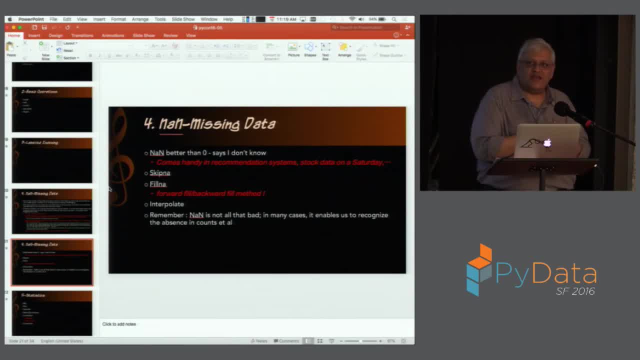 It's not So, for example, the recommender. that's happening on the other side of the room, right When you do collaborative filtering right. What happens is: you suppose you know that you have rated two movies, somebody else have rated five movies? 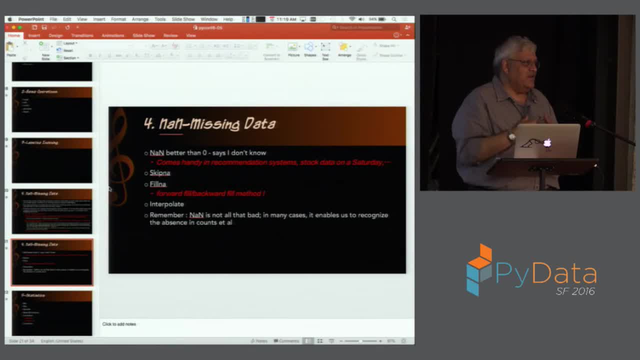 and if there are common ones, based on that one, you can say whether you like this movie or not, which is all fine. But if you get somebody right who hasn't rated any movies and then say: okay, give me a recommendation. 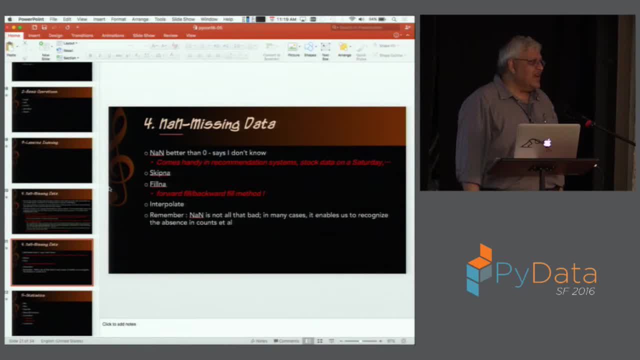 for this person. what would you do? You can't do anything, right? So you have to return an NAN. NAN which says I don't know. So NAN is good, And if that is there, maybe you can do when you do count. 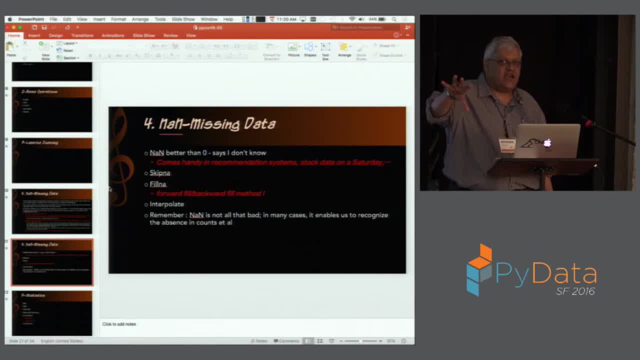 and various other things. it will give you NAN and you can look at it and say, oh yeah, in this data there are this many things that we have no clue about. Okay, So that's it. So one way, NAN is good, because if you put zero in there, 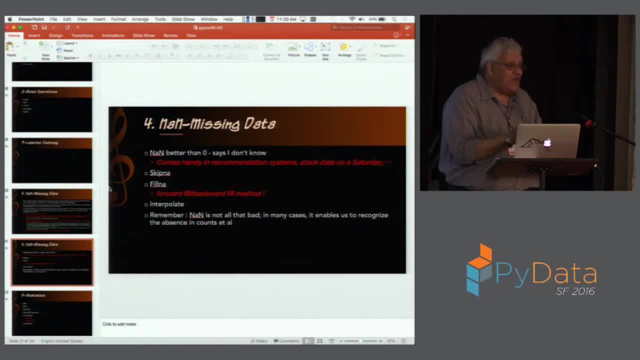 there's no difference between zero- and if you have a zero rating, you don't know How do you say I don't know- versus actual zero. So NAN is good, but you have to treat it, you know. And Pandas has a skip. NAN fill, NAN, interpolate. 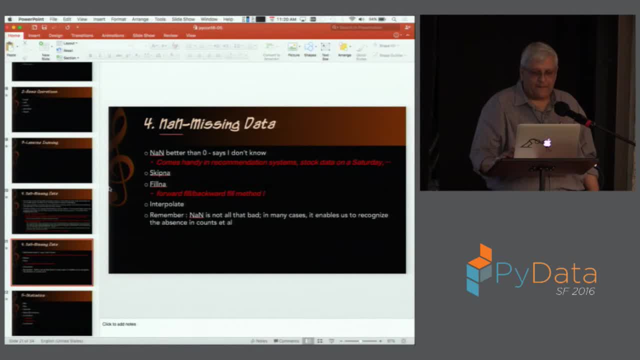 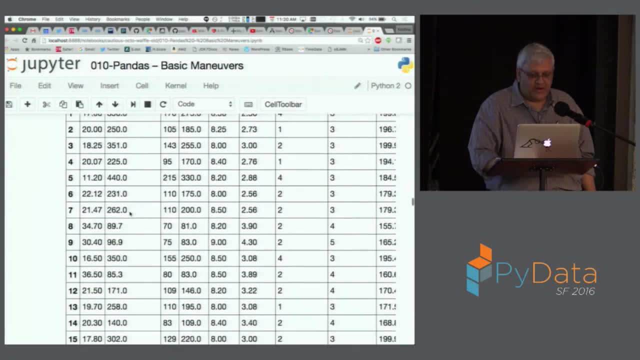 Interpolate is the one where you can do interpolate all kinds of stuff. There's interesting ones in there Moving on, So you know, drop NAN NA is one you can do. drop NA. so, for example, you know. 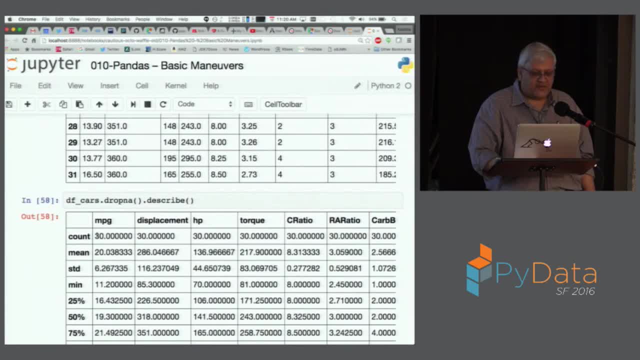 remember earlier when we did this one it had. so now when you do this one, see 30, right, Because earlier we had 32 records. Drop NA took out those two records which had this torque to be NA. 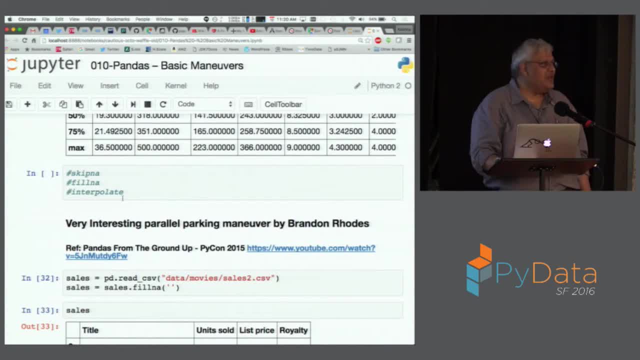 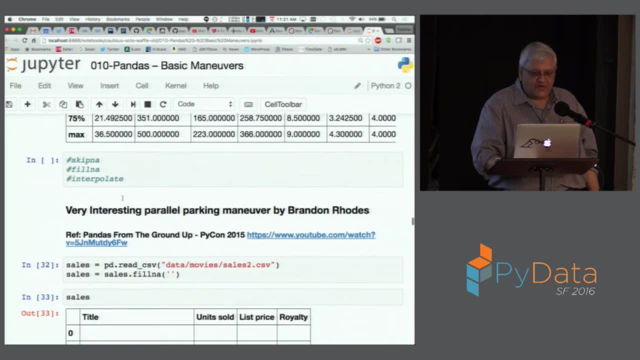 There is a skip NA, fill NA and interpolate- right, These are some interpolate is. you have got interesting functions where you can do. you can interpolate this one, So this is an interesting one, Interesting. okay, See this data right. 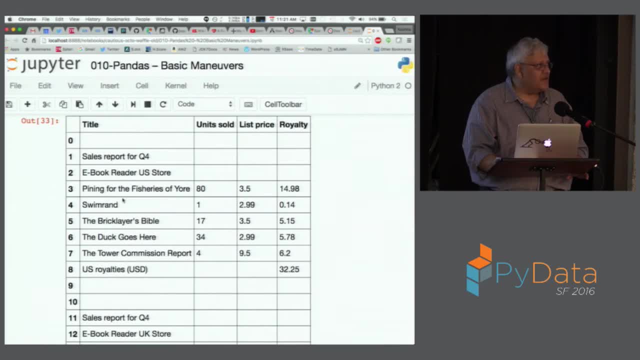 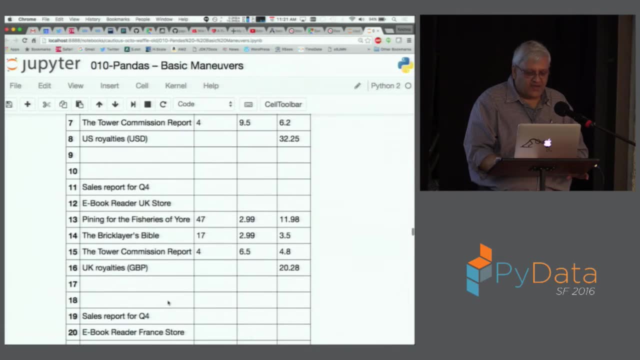 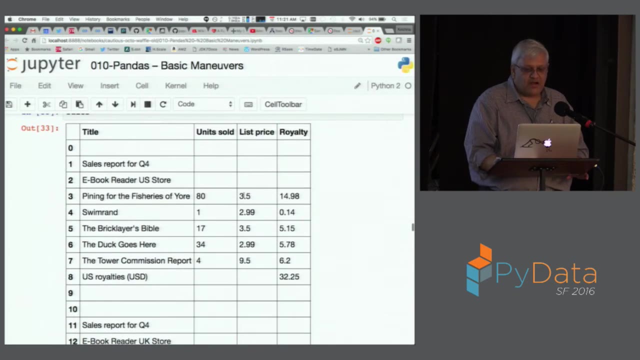 This is from Brandon's this thing. He gets this report. It says sales, sales, sales. You know you have the royalty. This is USD, This is GBP And this is euros. right? So he says: I want a column which says how much. 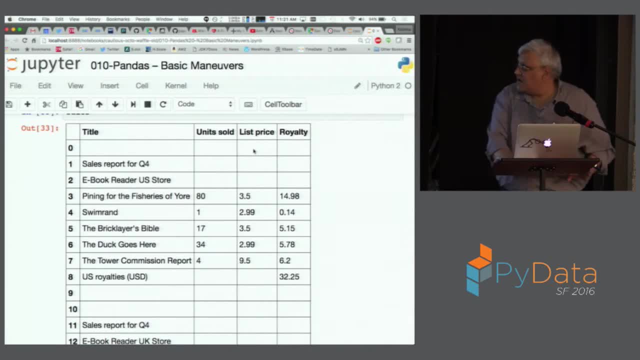 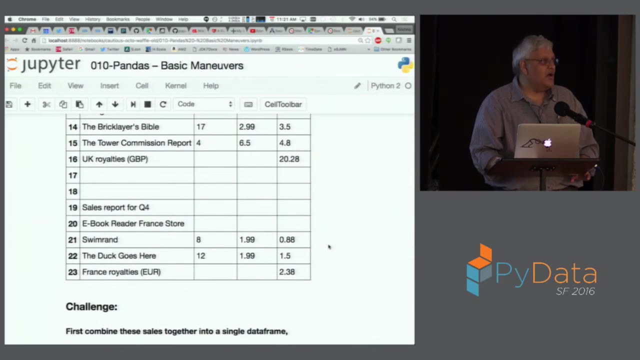 how many, how much amount the customer spent? right, Which is units sold by list price, Which is fine. But then the problem is, the currency is different at different, different rows right. Here you have USD, here you have GBP, here you have EUR. 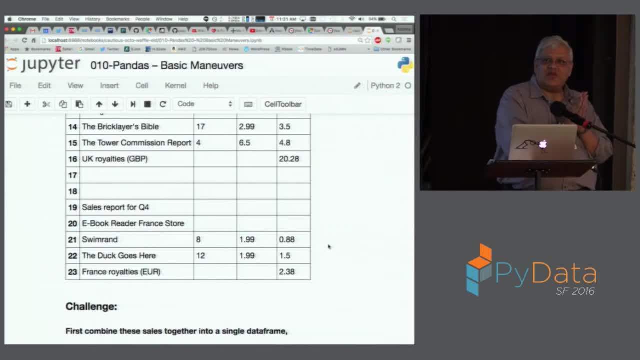 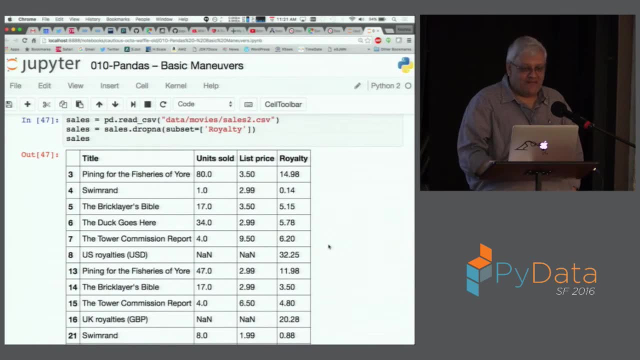 So how would you, how would you fill that in right? So this might be a good thing to look at- fill NA, and how do you do that? So what you do is- I'm just quickly going through because I think first of all you do the drop NA to get rid. 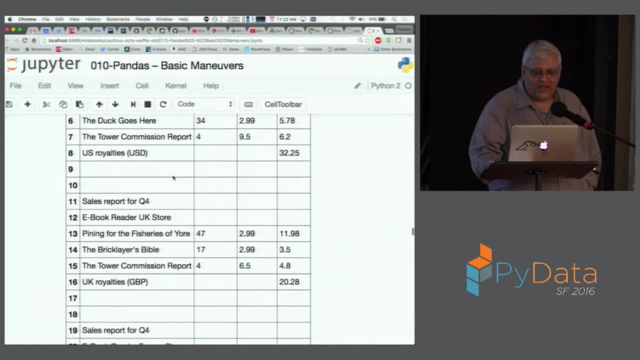 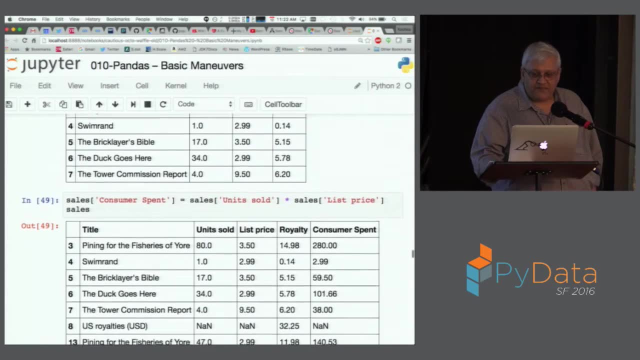 of all these spaces right. First, you do the drop NA, You get the drop NA, you get this like this, which is good. Then what do you do? You go in and amount spent, which is a new column sales. 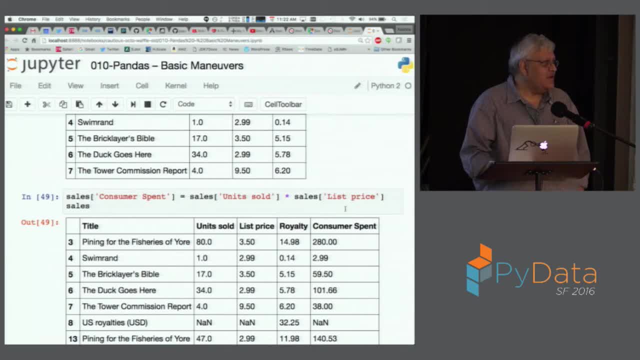 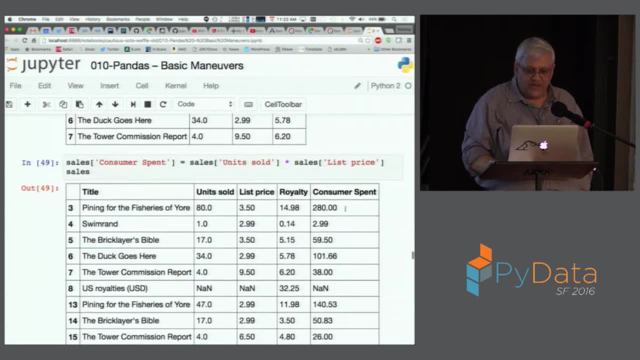 star. you know, units sold star list price. right, Which is fine, Which is straightforward. You add a column which multiplies the units sold versus list price. you are in good shape. That is good. Now how do you put the currency in? 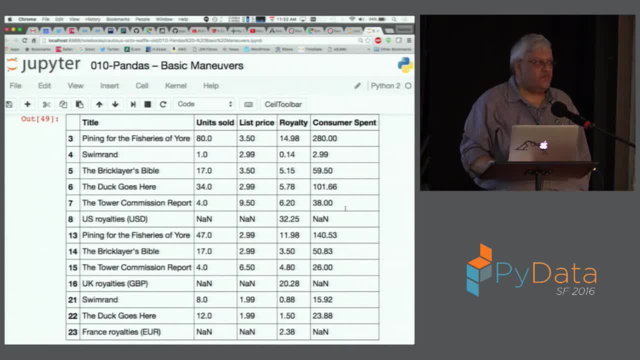 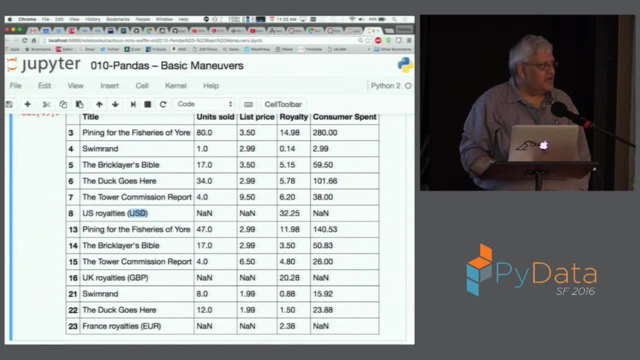 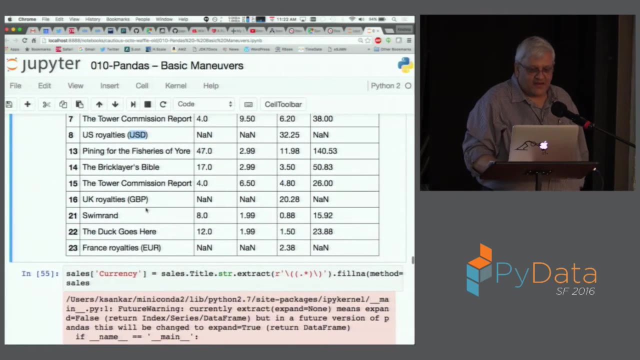 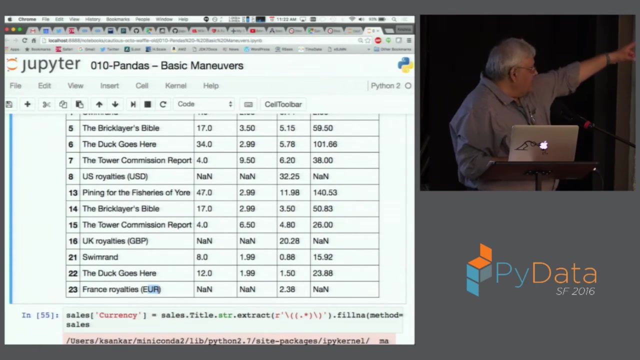 Any thoughts? Where do you have the currency? You have the currency sitting here, right? Yeah, So thank you. So the first is what you have the this thing here, right? So the first thing you can do is search. 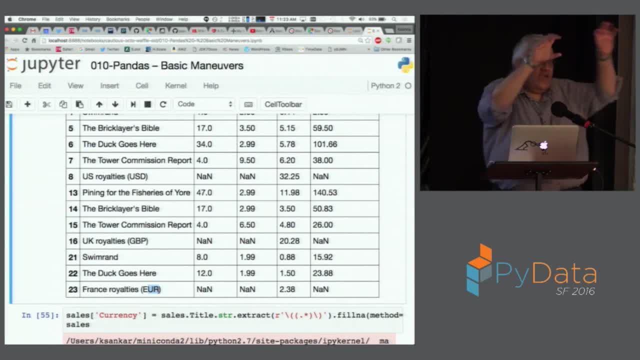 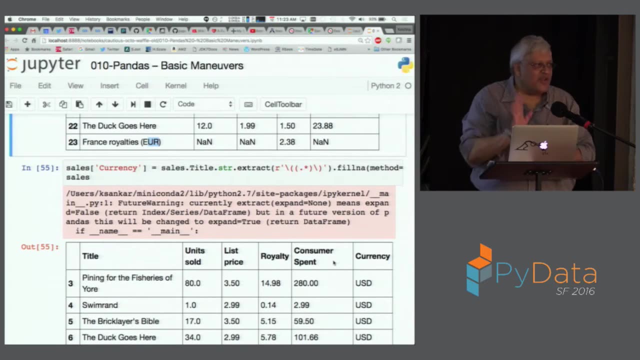 for things in between brackets, right. So you get USD, EUR, Right And most of the things will be NA right. And then what do you do? You put it in this column, So X? Okay, I'm going to. you have to bear with me in the sense. 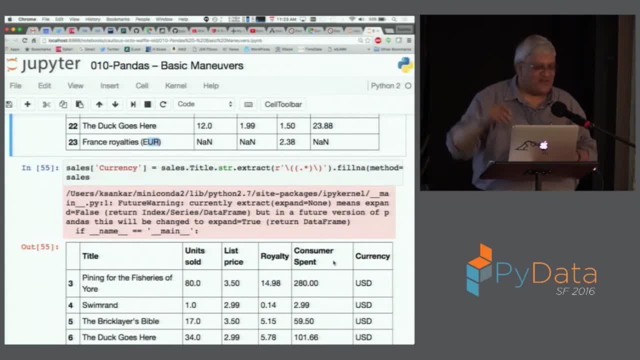 that because I have the whole thing in one column. I need to split it so that I can show you how this happens, right? So I'm going to. what they say is: you should never try these things when you're doing with the audience. 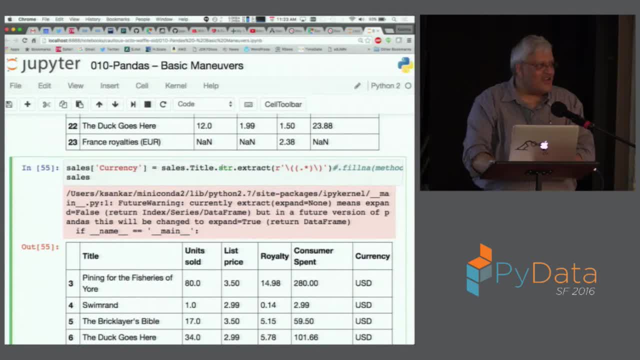 So this is what You're Remember, this STR. So this is where remember that we talk about this string functions on this STR namespace, right, STR, SUBSTR, and you have this regex thing, right. What you are looking for is you are looking for things. 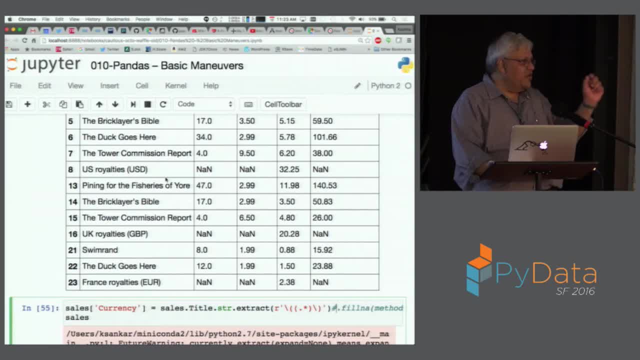 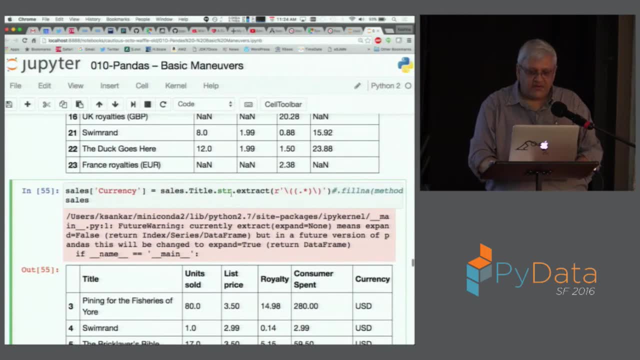 in between brackets, And when you find that things in between bracket, you're going to create a column and put it in there, right, Which is good. So this is Rumber. The STR functions act on the column Right, So this is Rumber. 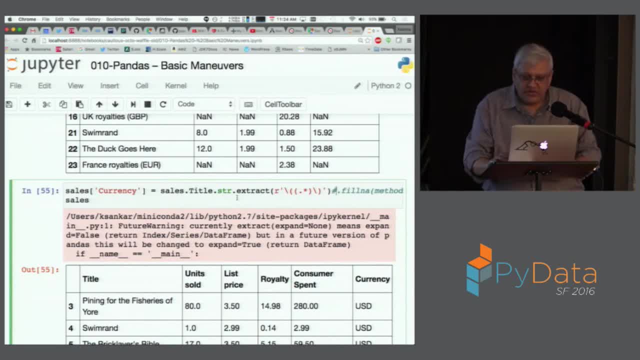 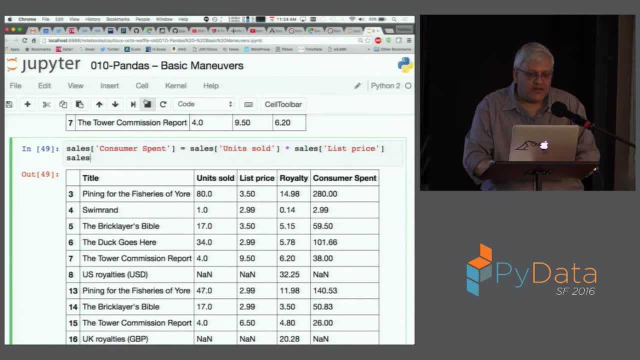 On a column right, It is not on this thing. So when you do this, I have to, okay. So the first thing I have to do is to run all above right. It has to run because I haven't been running these things right. 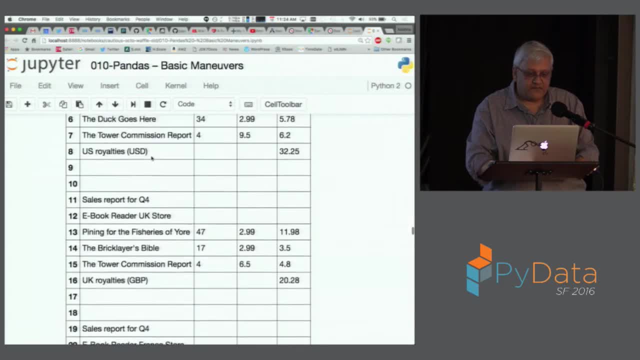 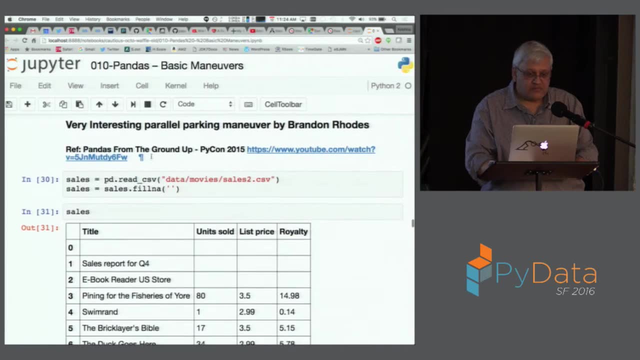 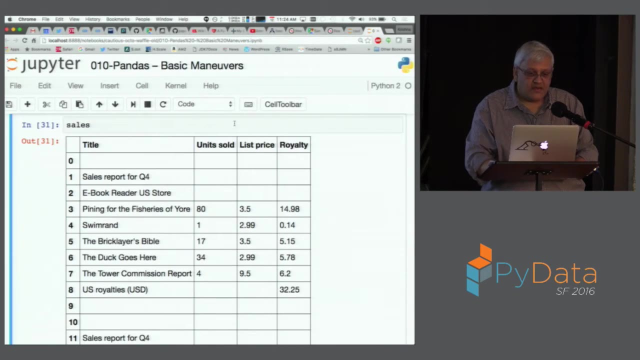 So let me run these things. So let me run these things. So maybe I didn't have to run this one, So let me do this guy, Let me do this guy. Yep, Sales is there, So let us go down. 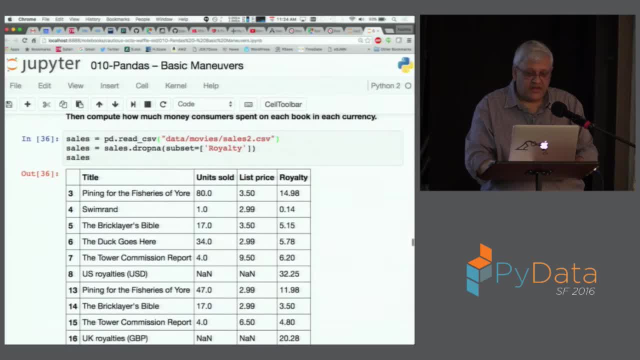 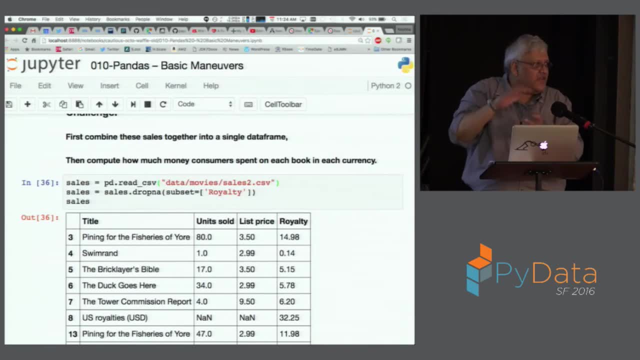 And these things are there. So first thing we did was drop in there. right, You drop all the frivolous columns. So now you have got at least everything is in pack, this thing, Now let us go down and you know, just get the head one more time. 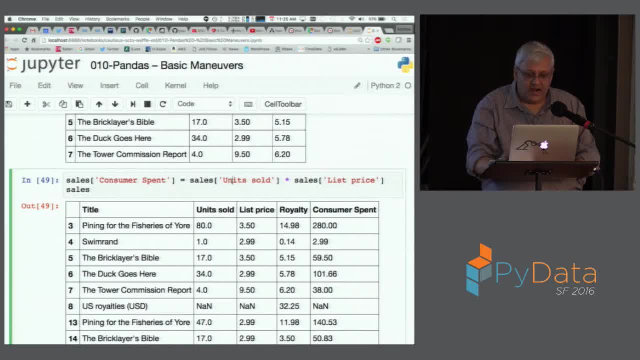 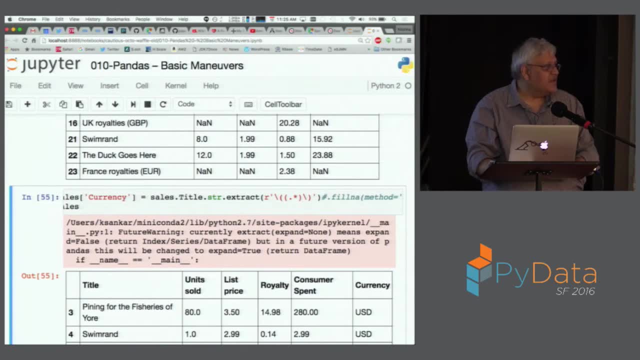 So that you know. so you know. you add the. you add a new column, which is very simple. After adding the column, what is our next thing? We search for the currency. We search for the currency. Actually, I should say we hunt for the currency. 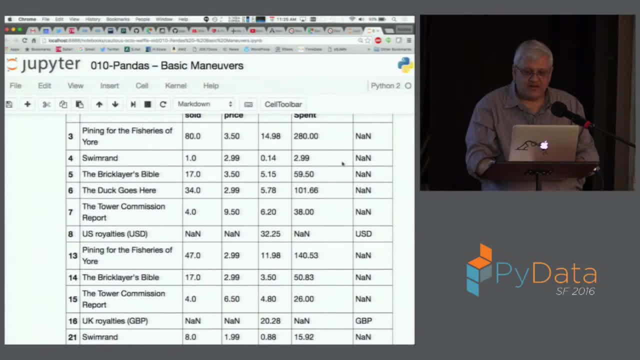 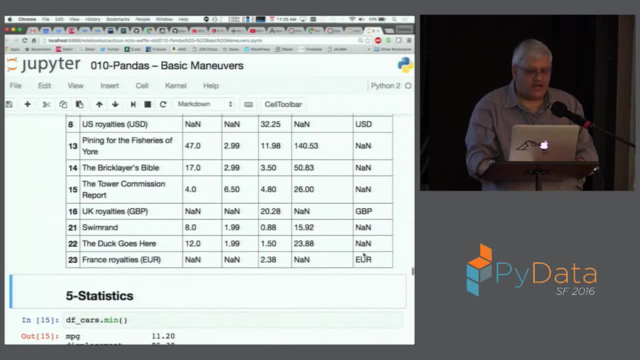 We do, We got it right. See, tons of NAN one USD, tons of NAN one GBP, tons of NAN one EUR. right, Because because the bracket, The brackets were only here, They were not here. 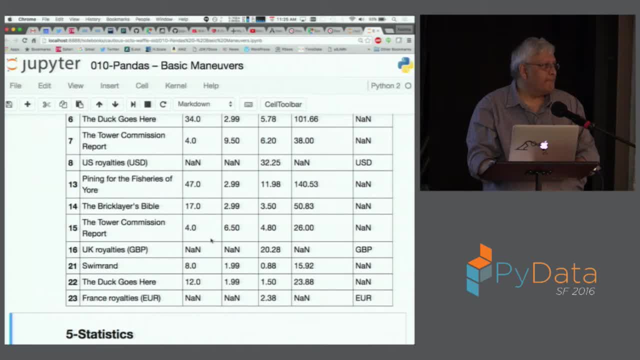 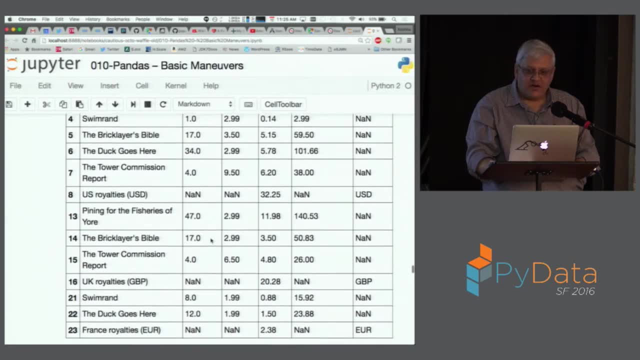 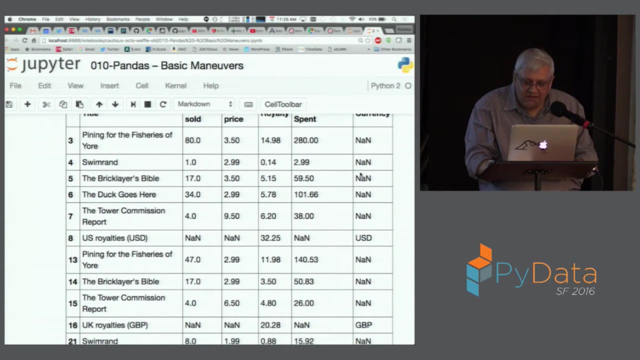 Now, what do we do? We have a fill NA, right? What we want to do? we want to fill NA. You want to go up to USD and then fill the guys up with USD, right, Not down right. 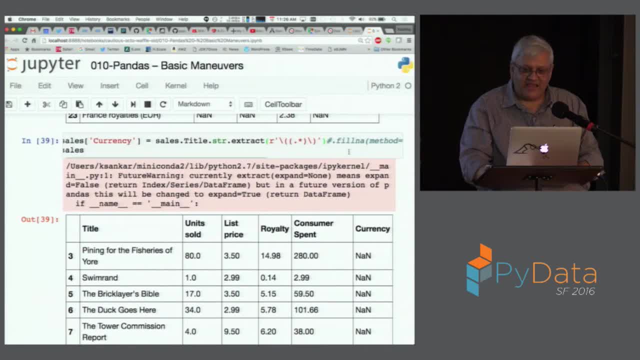 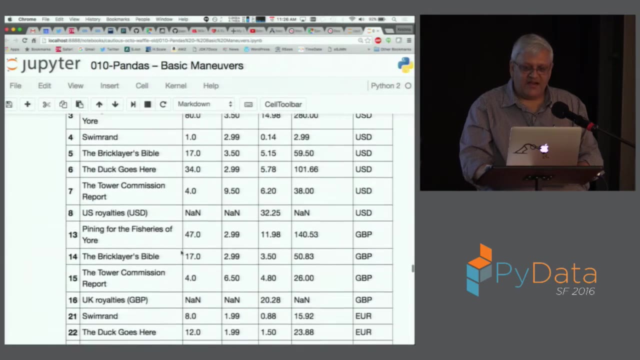 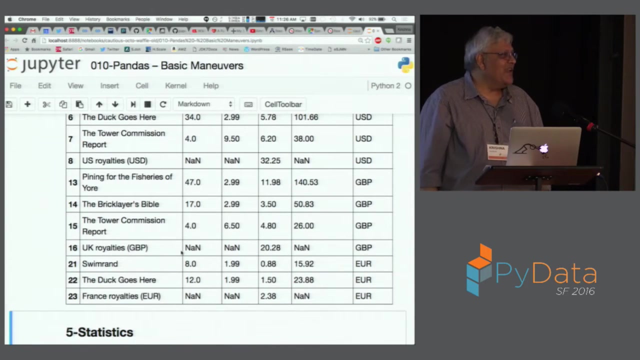 So there is a thing in: fill NA Method is backfill. So you go in fill NA backfill. See what happened. It went in and we got nice currency thing on the top right. So I thought that it was an interesting, very interesting. you know, parallel parking. 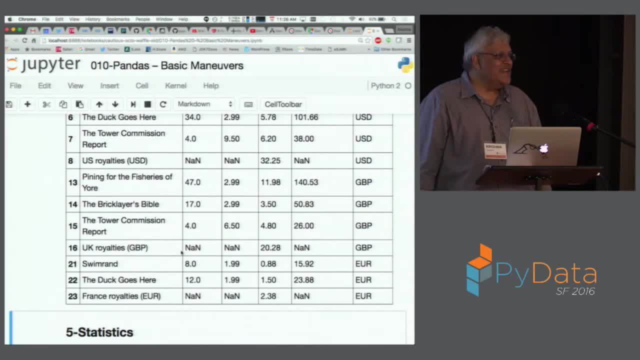 because you know I come from Volvo so I do autonomous driving and that kind of stuff, right. So parallel parking and maneuvers and all kinds of stuff, autonomous driving and all this, right. So anyway, see how, see how we were able to use here NAN was good, right. 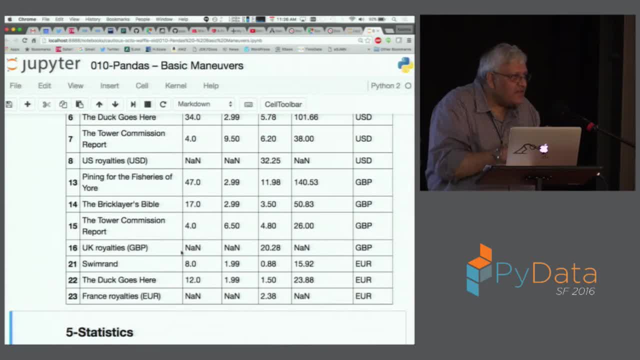 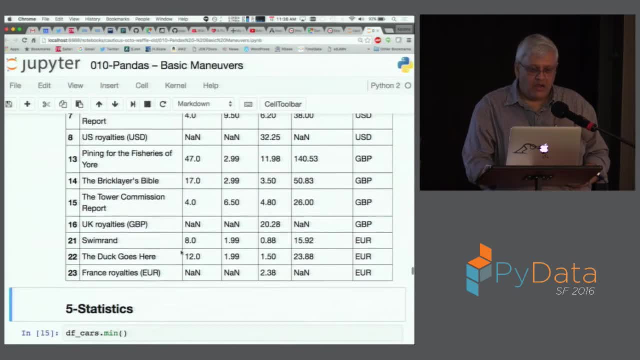 Because you had NAN and you were able to say: some of these had USD and various other things you go in. you looked at it and said: give me, backfill back, and you were able to fill it. This has statistics. So, going back, switching back into this one, 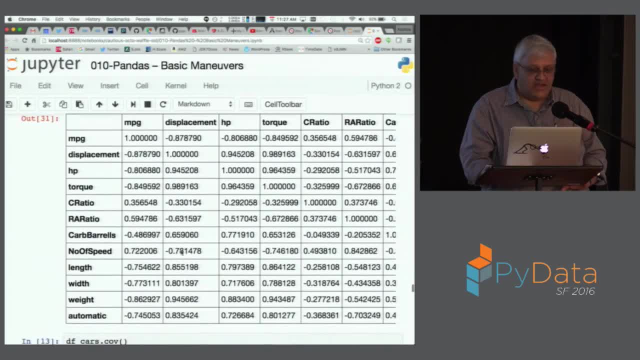 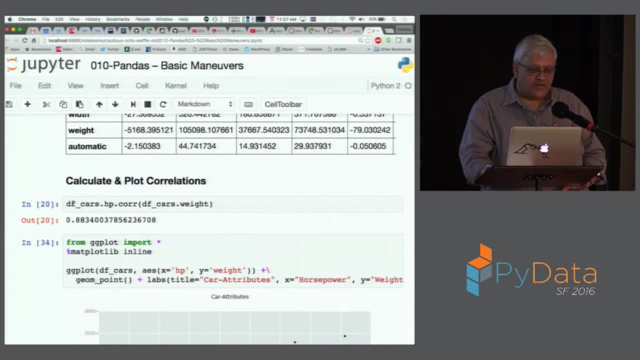 Min, you know quantile correlation, it gives you the whole correlation. Or if you covariance, all kinds of stuff is there. So you can see that, If you want, you know. so this guy right, this one, this returns one number, right. 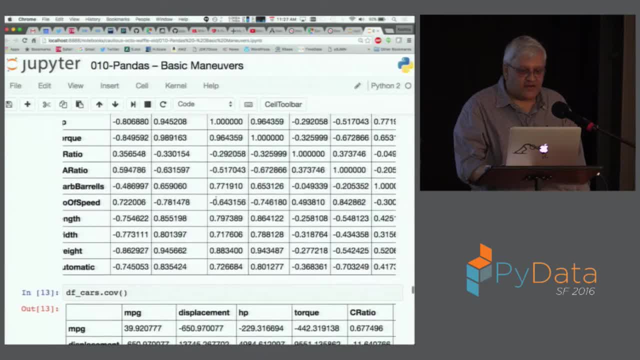 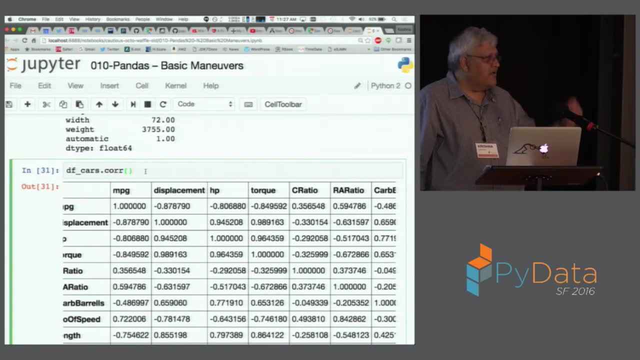 What is the difference between this and this correlation? This correlation acts on a data frame which returns another data frame with right. It is a cross correlation between all the variables. Here we went in and we said: give me the correlation. 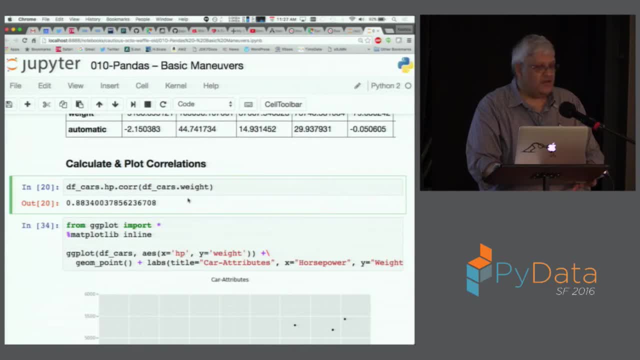 Of horsepower versus weight, So this gives. so now we are doing a correlation on a series and that gives a number, Because you have one series and say: okay, give me a correlation between two series. it's nothing but a number, right. 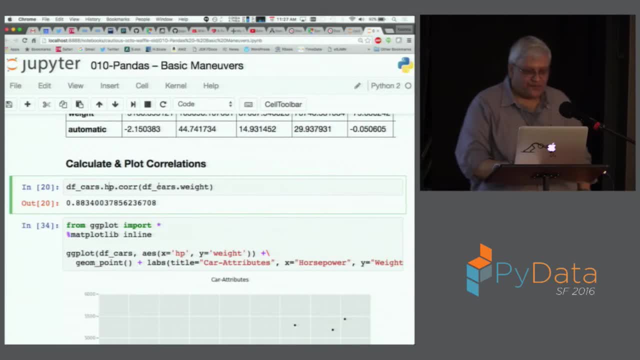 Because it looks at the correlation and gives you a number. So this is where you keep an eye on what type of objects you have, what type of operations you do. So then there is a plot, You can do the plotting, Et cetera, et cetera. 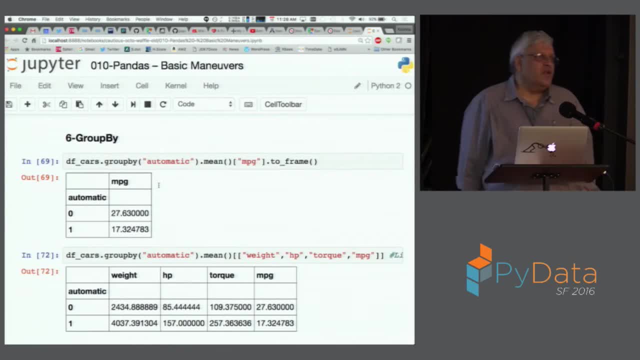 So I'm going to you know. oh yeah, So this is one. The group by probably is one of the most powerful ones. right, You want to look at. you have this car, HP and weight and all kinds of stuff and miles per gallon. 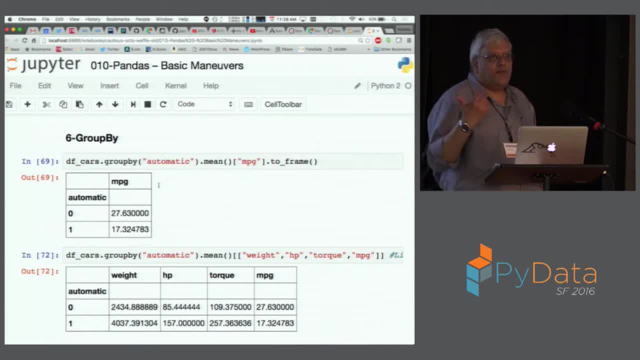 And you want to look at it and say: automatic and transmission, What is the? you know which one has better mileage right? So what do you do? You group by automatic And then you find, You find a mean right. 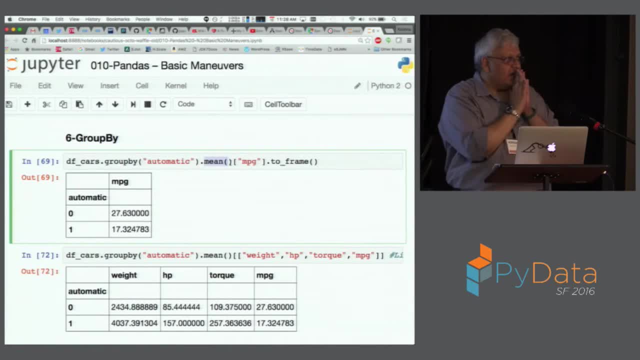 So you say: take all the automatic. So this is the thing they call split, apply and combine. You take the data, split it by automatic. So all automatic equal to zero goes in one, or automatic equal to one goes in another. of these things right? 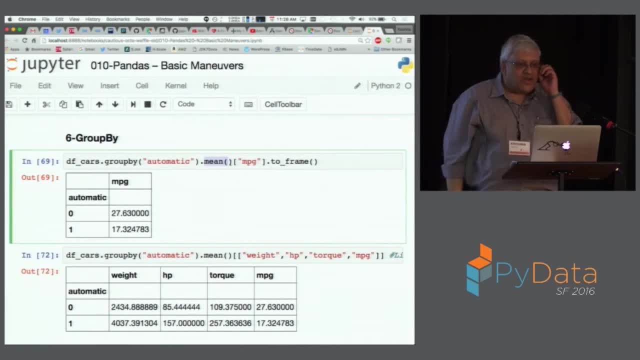 And then what you do? You apply a function which is basically mean: In other places we will do sum, et cetera. We will see how that happens. And then you combine, So you get a tiny, you get an interesting data set, right. 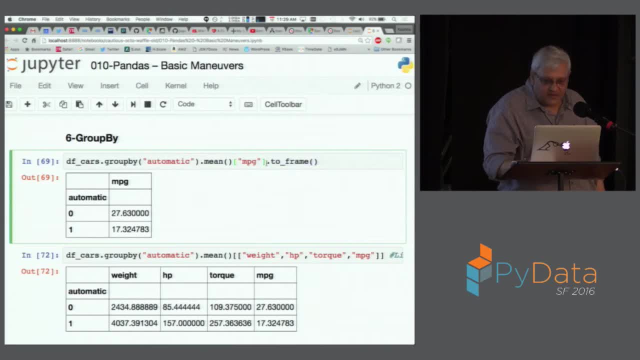 So this two frame is: if you do this right, I'm going to try this. If it doesn't work, don't hold me to it. It's because we haven't done other things, but probably it will work Right. 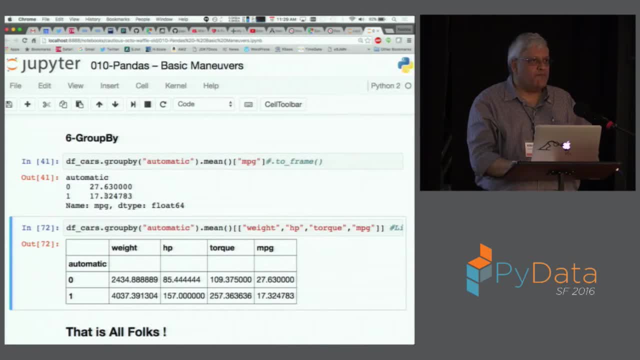 If you don't have this two frame, we got what is this guy? It's a series, right, Because it's a column. So when it's a column It gives you a series. Of course, you know we all want to work with the data frame. 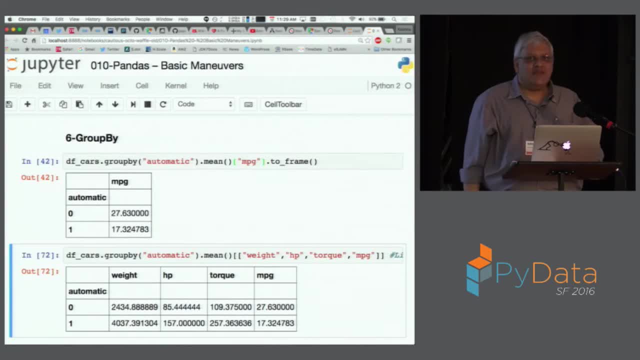 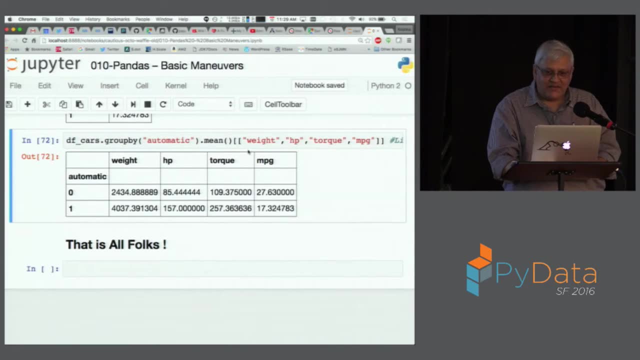 So you do the frame. You get a nice data frame out of it. We will see more when we go into it. Anyway, so this is a group by. Keep this in your mind, right, You can do group by various other things. 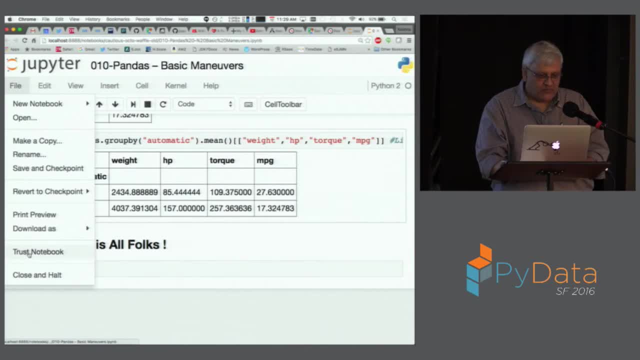 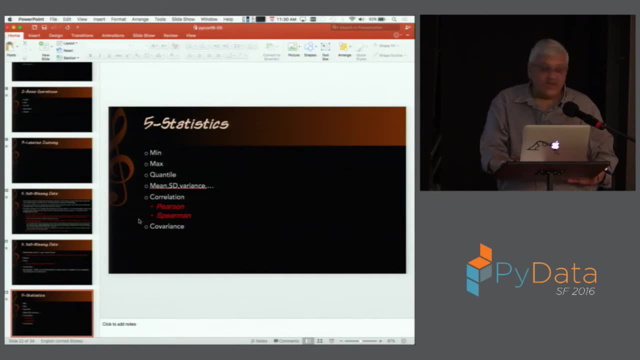 So we are in good shape. So we saw the statistics. You have Pearson correlation, various other things, Spearman correlation, et cetera, et cetera. We saw the group by as well. So this is a good time. 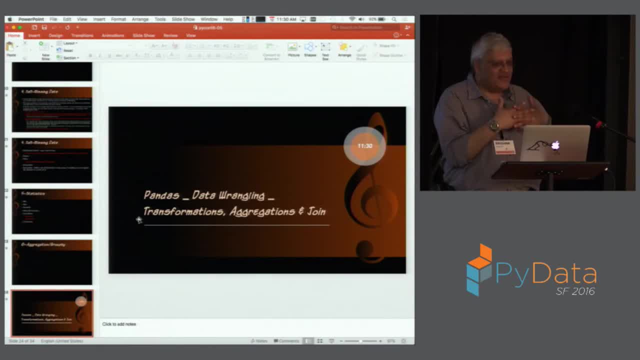 So now that we understand the basic maneuvers, Now exactly 11.30.. See, guys, I had that 11.30 marked there Because I had always this thing on there which says: this is where I should get to this thing. 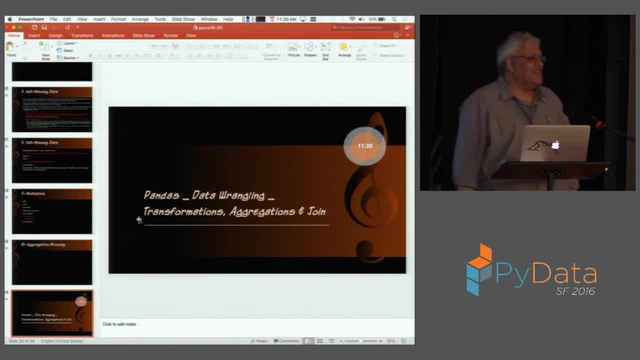 And we exactly go to that. Thank you, You have been a good audience, Anyway, because we have only 90 minutes, So I need to cover the whole thing right. Even then, I have more than what I could cover. 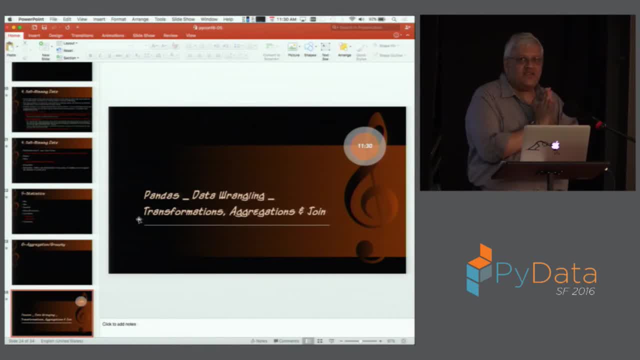 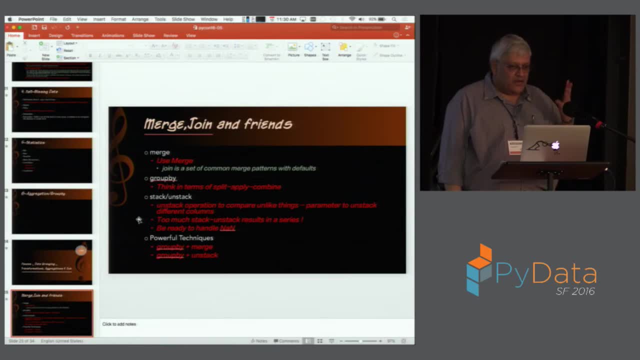 So, anyway, Now let us look at data sets. right Now, this is a time to look at data sets. Let us look at some data sets. We know what the basic things are Before we go into data set. there is another one, merge. 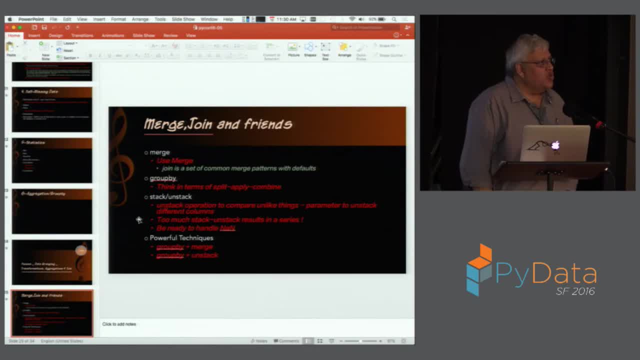 Right. Merge is like the join You merge to, you know, to data frames. We will see how the merge works. Join is, you know they also have join, which is a subset of merge. So always use merge. 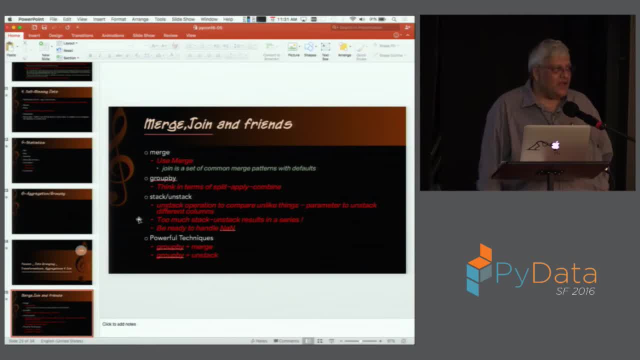 We saw the group by. We also talked about split, apply, combine. Another thing is stack and unstack, So what happens is we will. so this is, these are the things where you will know more when you run it rather than looking at it from this person, right? 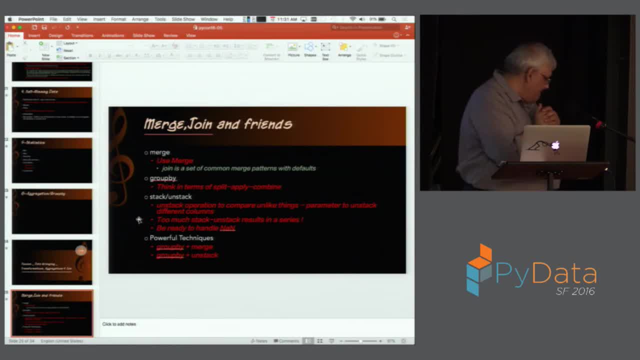 Anyway, just keep in mind, okay. So let me take from my ad tech experience: right, You have, you have the TV data set, right, People who watch that kind of stuff, right, Okay, Then the, the, the, the one of the column is the type of the genre, for example. right, 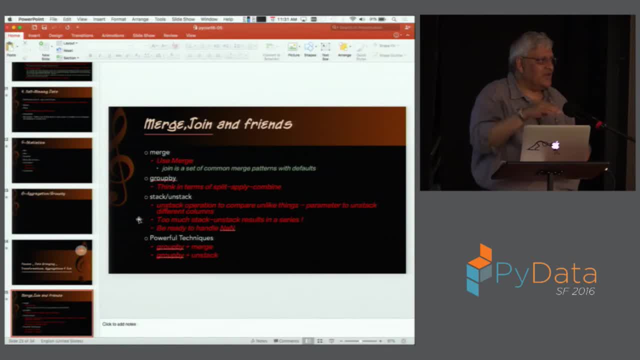 You have horror, child adventure, et cetera, et cetera, right Now, and then you have all these things people watch and they're going to. so now you want to look at it and say: no, I, I, I need to take this thing and make it a column. 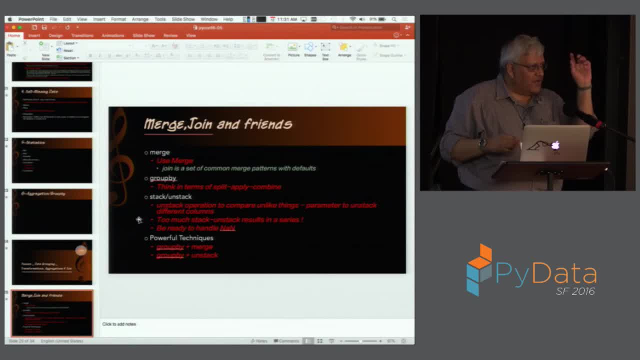 So it's a transformation, right? You take a, a, a column and turn it into a, A column, heading and on, based on the rows. We will see that one. I I'll show it to you, But anyway. so what happens is it turns this thing around. 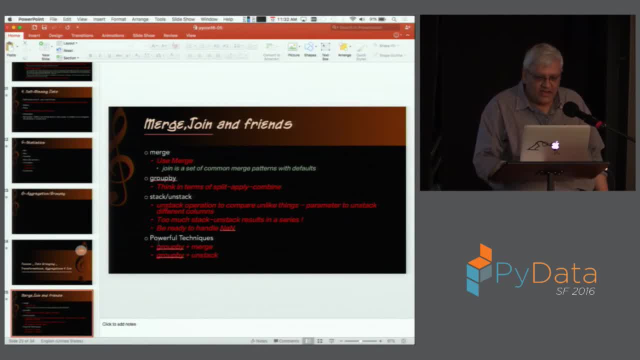 It turns based on one column around: We, we will see that one. So the, the group by and merge, and group by and unstack. These are the two powerful ones. We will see that one right, Because so this is our next, this thing, you know so. 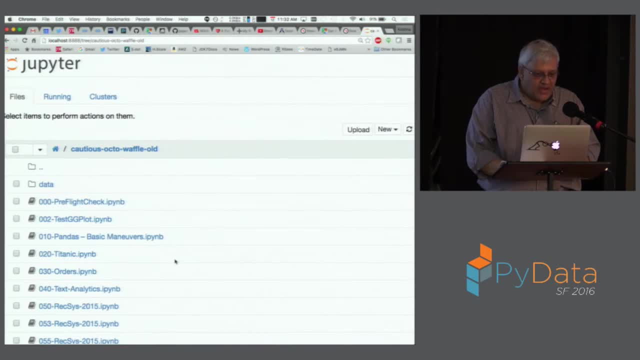 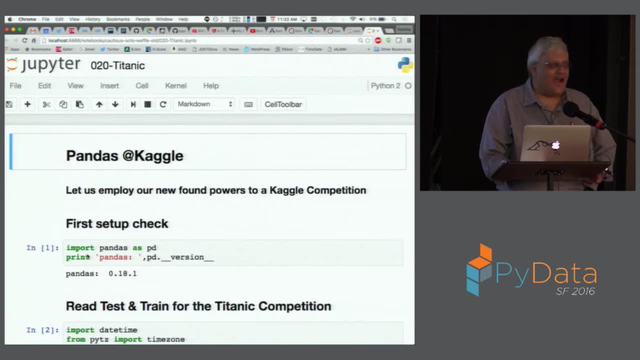 So how many of you have heard of the Kaggle competition? Right Yeah, Good, Excellent, Excellent, Excellent. Ah-ah, We have a whole Kaggle. So that means you have done the most. probably you have done the, the, the Titanic. 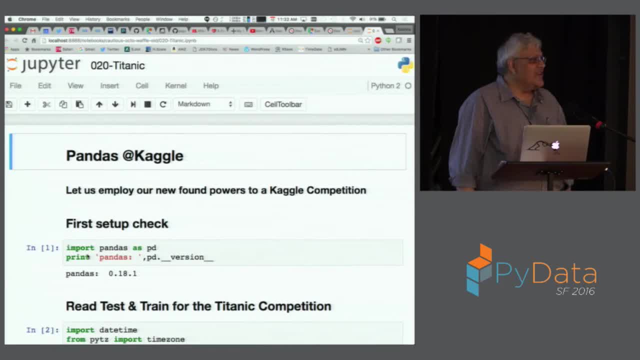 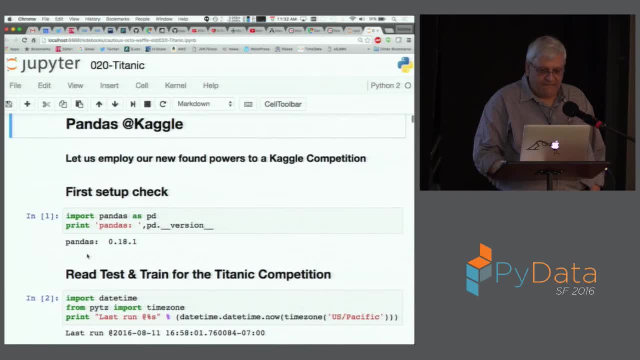 That is one of the classic ones. right, And probably you have done the Titanic using pandas. You know the the Titanic data set. So let us look at, look it up, So let us employ our newfound, you know, powers. right, 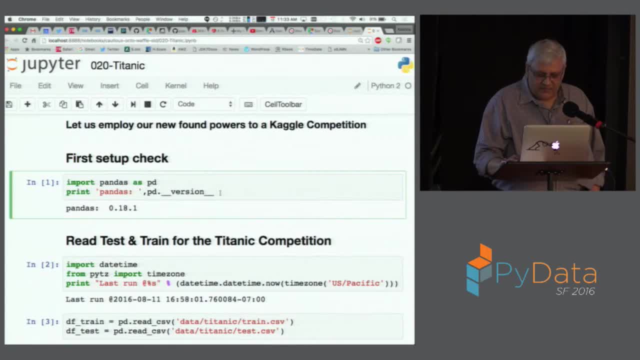 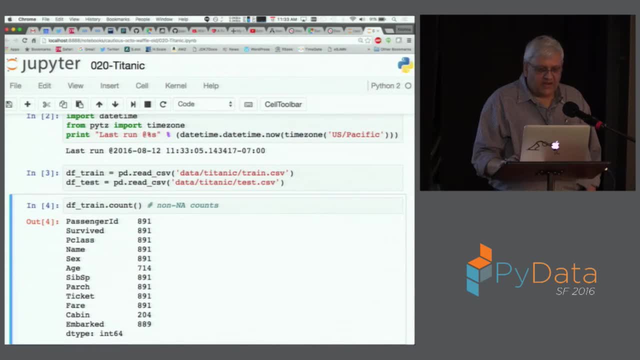 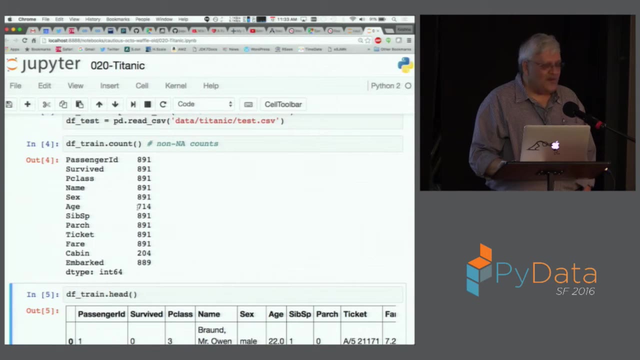 The ability to manage this one. Let us go in So you have the train data set. First is count. This should bring tears to our eyes. You know what happened: right 714, right, Only 714 has age. 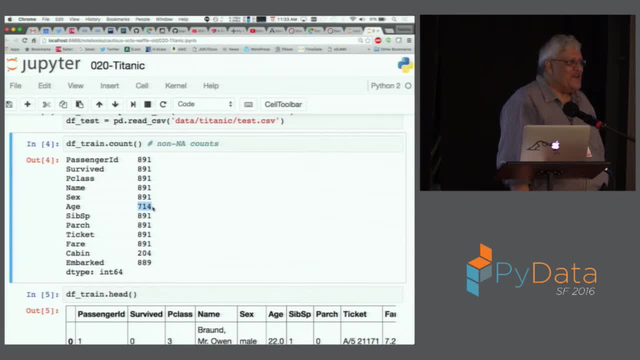 And the rest of them don't have Right. So that means we have to drop all of them And remember what we are predicting. we have a passenger ID, a class name, age, et cetera, et cetera. So what we are predicting is that we have a passenger ID, a class name, age, et cetera, et cetera. So what we are predicting is that we have a passenger ID, a class name, age, et cetera, et cetera. 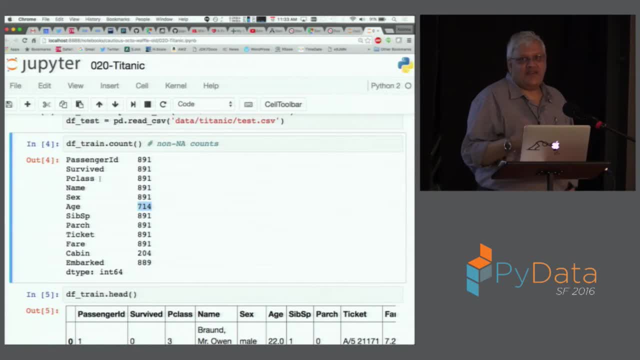 So what we are predicting is whether they survive or not, right? So age is an important factor, right. There will be. maybe age is an important factor, right, But probably age is. So now we need to figure something out. 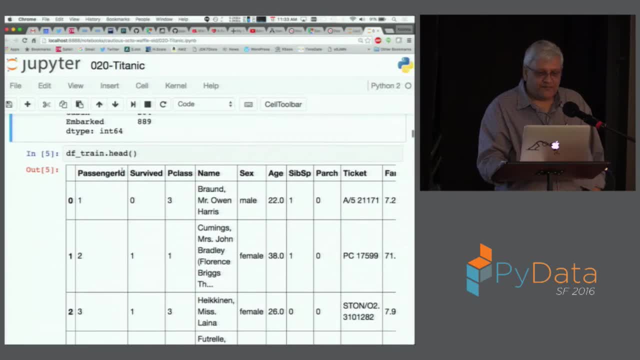 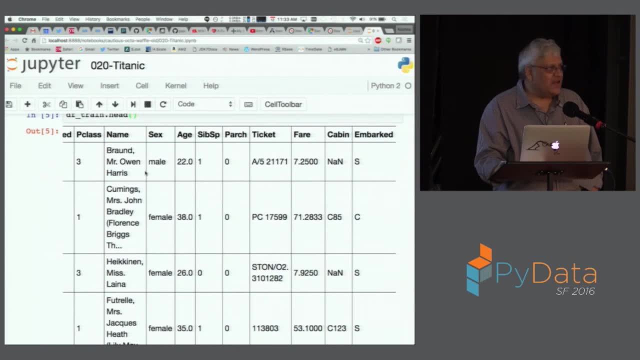 So this is where one of the interesting things comes in. You have the head. We look at it. Yes, we have the. you know, we see a cabin number ticket. you know this, which says parent, children sibling. you know, spouse, right. 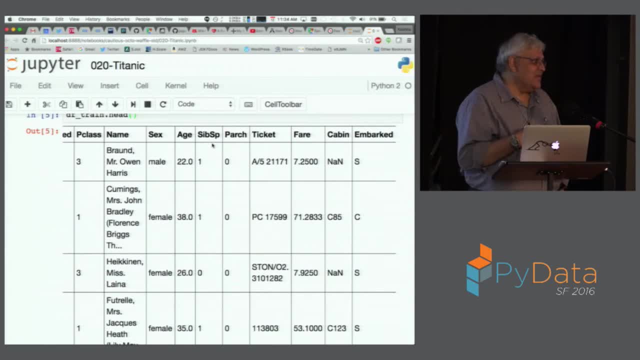 So what it shows is whether this person has a sibling, Because the idea is that maybe if you have somebody with you, you have a better chance of survival than if you have nobody right, Nobody who gets fine, right. So no, no, no, no. we need to get this person out of this one. 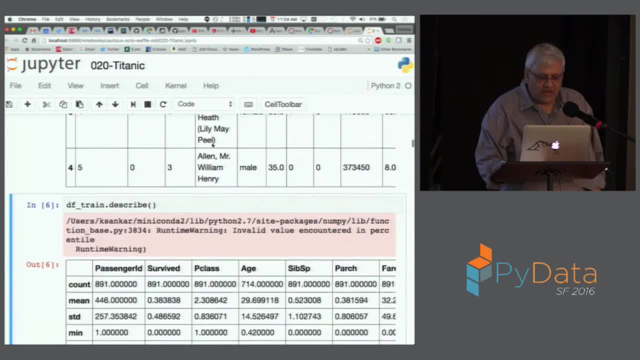 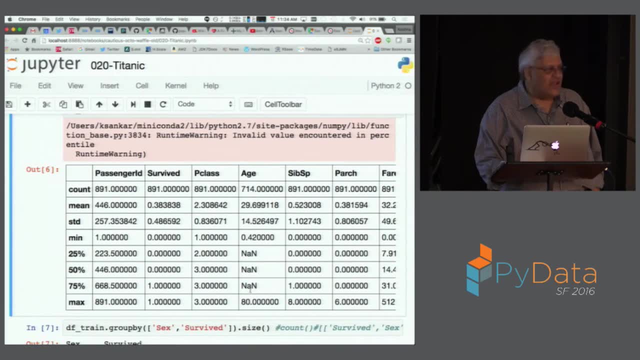 Maybe, maybe not. Anyway, describe gives you a description And you know we do the describe And here you can see that age gives you this NAN Because it can't do these things, because there are NAN in the age right. 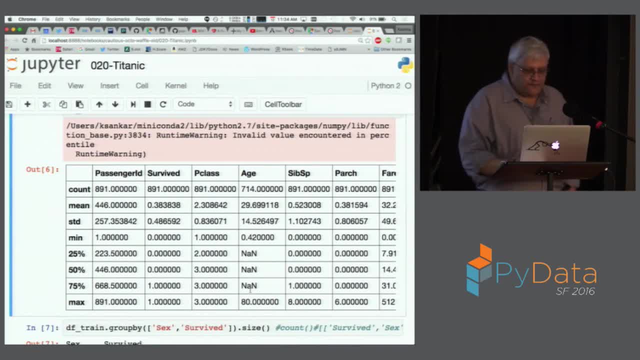 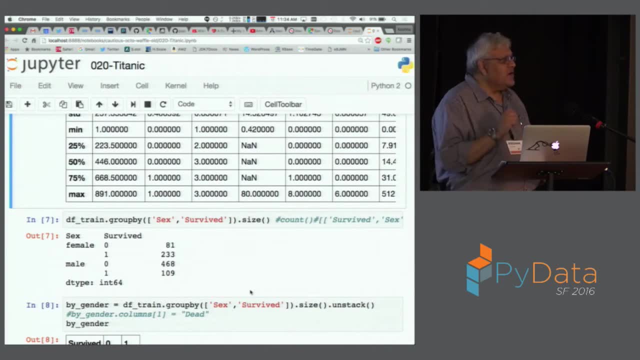 The major is missing. and it is missing. It says no, I can't do this one. So the first one right. Let us look at and say whether gender made any difference on the survivor right. So what do you do? 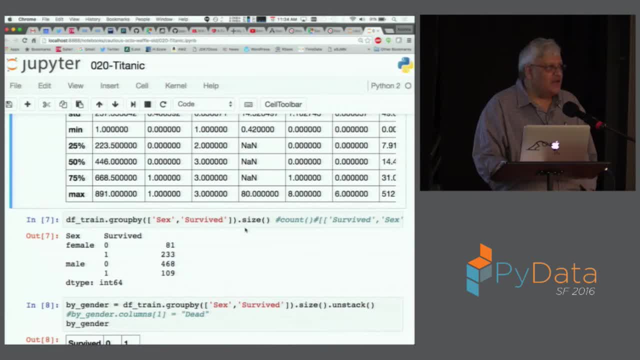 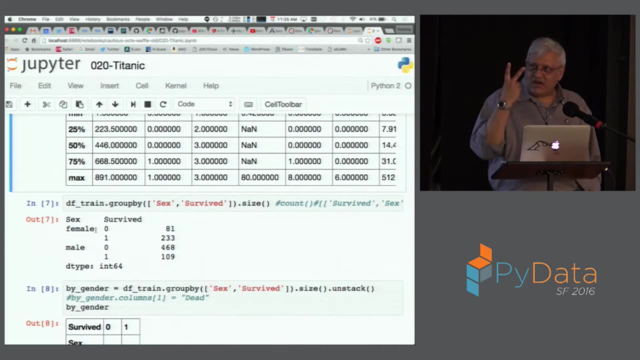 Group by sex and survived. and then the operation that you do is size. Naturally you get the, you get a series right. You see this one, This has got double series right. So this is a multi-indexed. There are two indices on it. 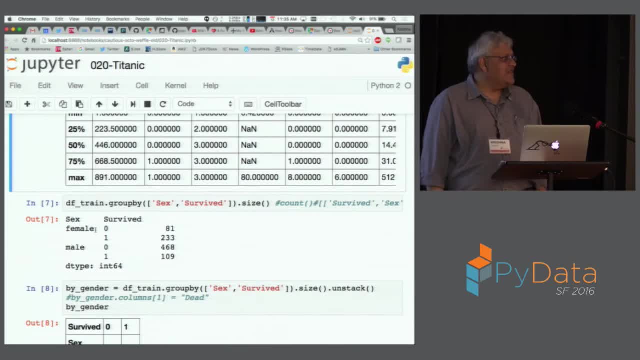 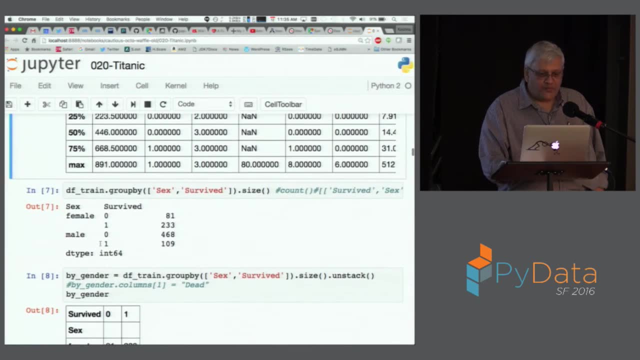 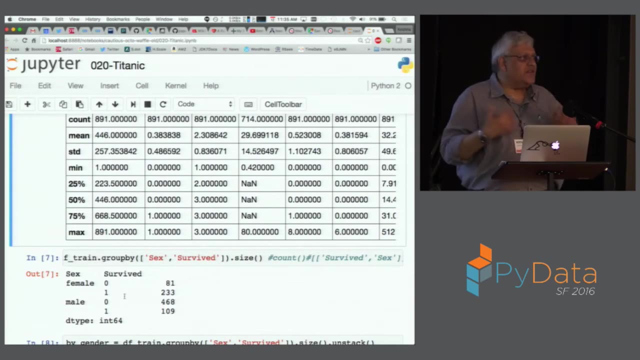 The first index is the gender and the second index is the survive. right, So this is the data and this is the index. right So now. but if you look at it here, right, How do you, how do you total them up and how do you take percentages? right? 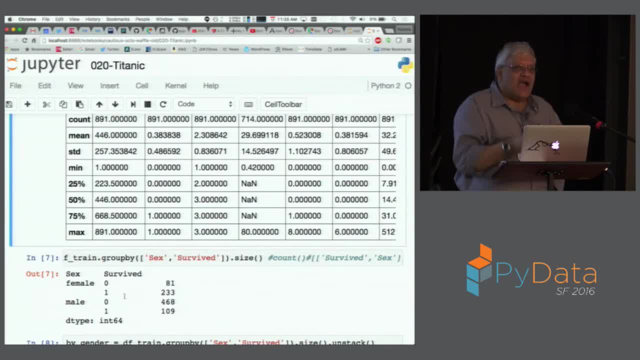 You don't want to go in and take rows and start multiplying? oh yeah, add row one and row two, and then you know, and then you know Row one by row one plus row two and row four by row four, et cetera, et cetera. right, 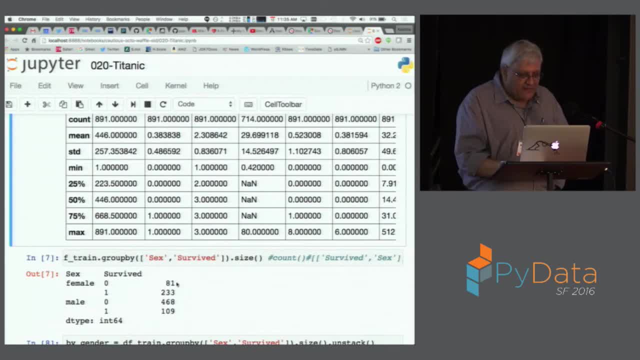 What do you want to do? You want to take this: survived on the top right, So you want to take that column and bring it to the top. What do we use? Unstack, Thank you, And we use unstack. 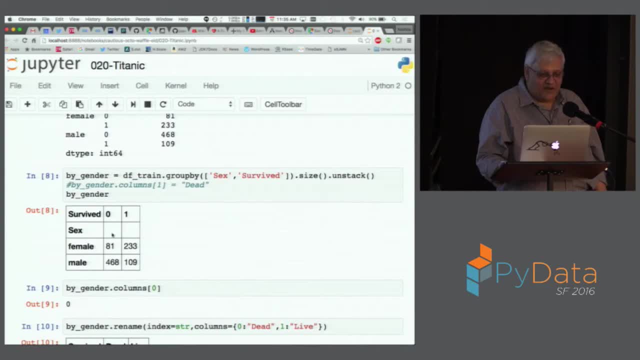 Now we are in good shape, right? What happened is you get zero and one and then you get the rest. So this is what. that's what I was saying. The unstack by explaining won't work, But when you look at it, it naturally looks at it and says, oh yeah, if I, so this is. 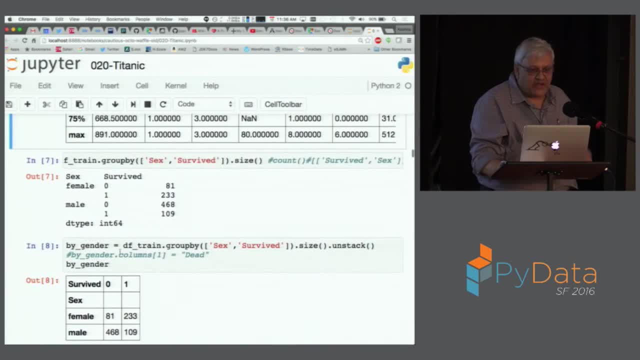 where, when you do group by, usually, when you do group by and when you have group by multiple columns, you get into a structure like this. right, Remember, these are the labels. They are not. you know they are part of the data, but they are. Pandas, considers some. 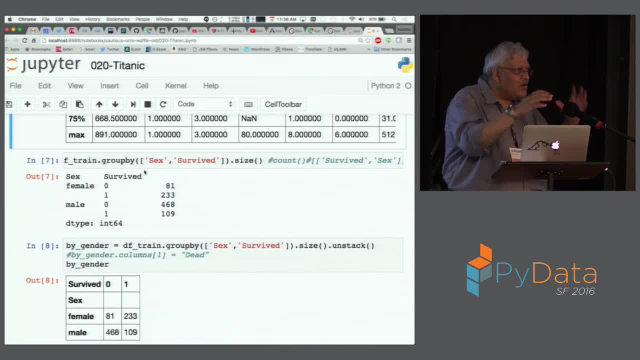 as labels, right? So, and then now you want to turn them around and say: I want to get a nice, you know, data frame. So you get the data out of it, You do the unstack and when you unstack it you get this one. 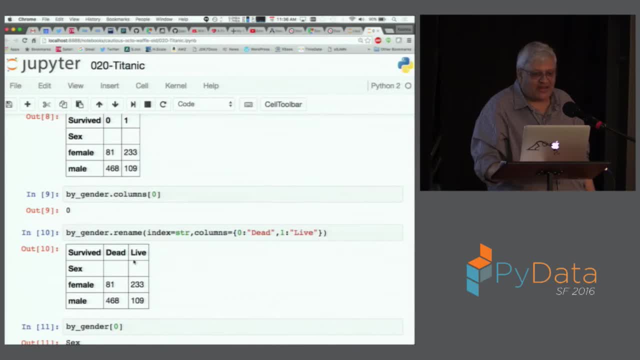 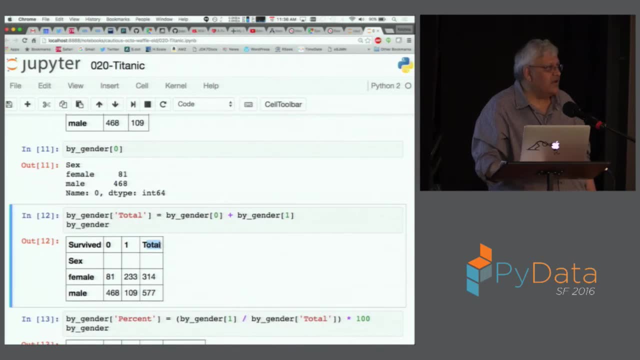 Now, when you get unstack, then you can also rename the columns like dead and alive. You rename the columns and then you add another column. It says total right, You do want the total number of males and the total number of females. 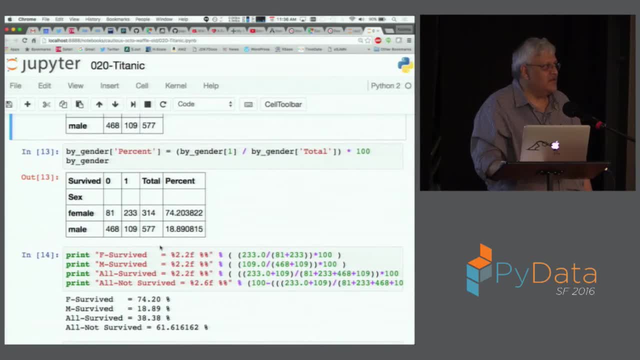 You get the total and you get the percentage. Does that make sense, guys? See how we, you know we were able to. We were able to apply the group by, We were able to apply the unstack, We were able to add columns and then we were able to, you know, do the column operation. 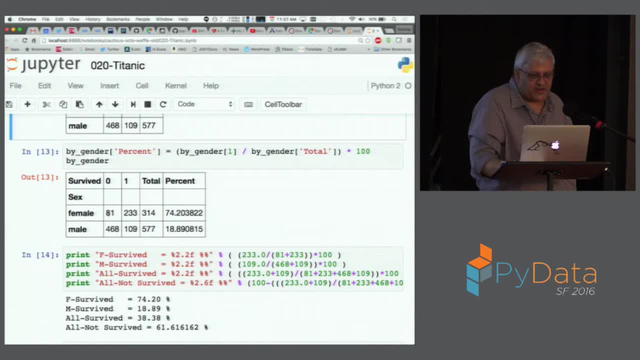 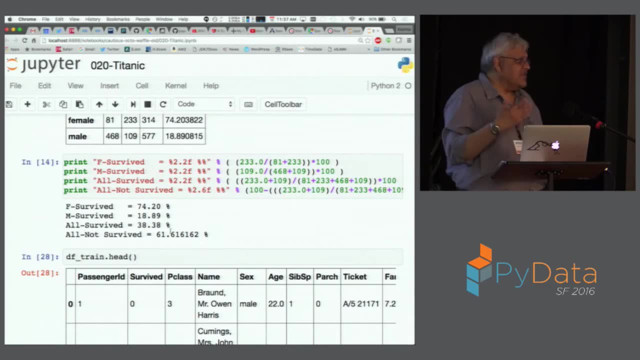 and now you can see that you know, 74% of the females survived and only 18% of the males survived. So anyway, so just to want to show that. So see how the manipulations come and you know how these things work out. 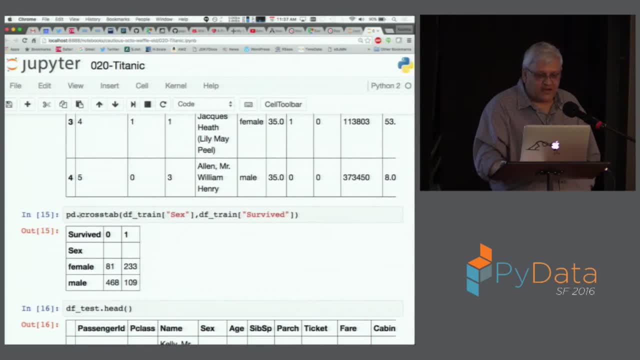 We could have done There is. There is another thing called crosstab, the crosstabulation, So the crosstab also will give you the same thing. So, interestingly, you know, without all these things we could have used crosstab. 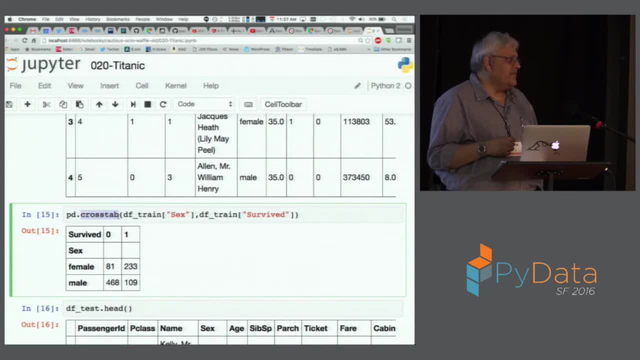 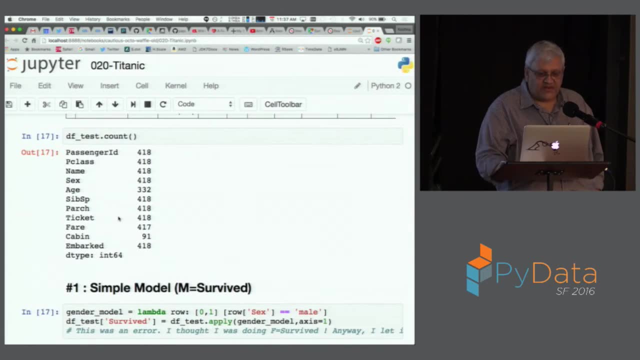 and we could have gotten the, gotten the similar structure. Then the rest of the stuff is: you know- yeah, I have to show one of these things, So fine. So let us get a simple model right, Very simple model. 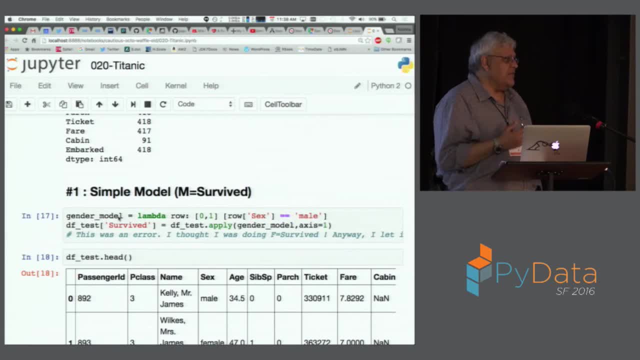 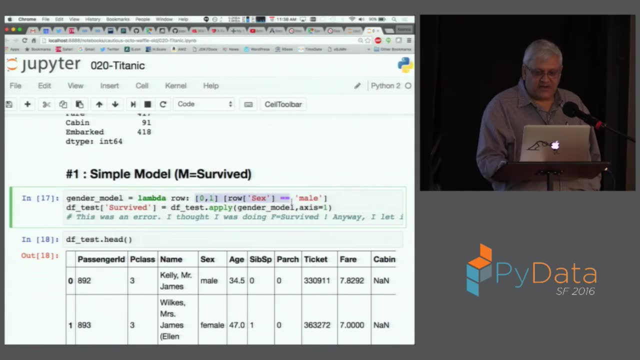 You know, let us say that all males survived, Right? Just to see what happens. So we make a simple model. Again, Pandas helps us, right? You have a lambda which says: you understand this maneuver, right? This is just a double indexing right. 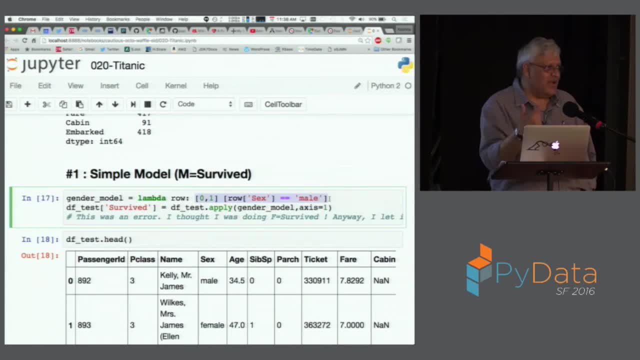 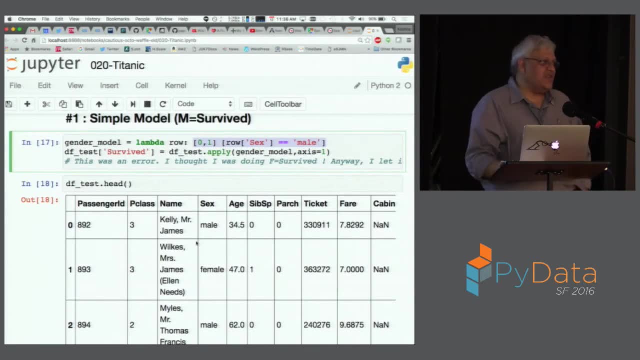 You have zero and one, And if it is male you get one. So you get the first one out of it And then you apply that one. So you apply. So this is the test data, right? You have the test data. 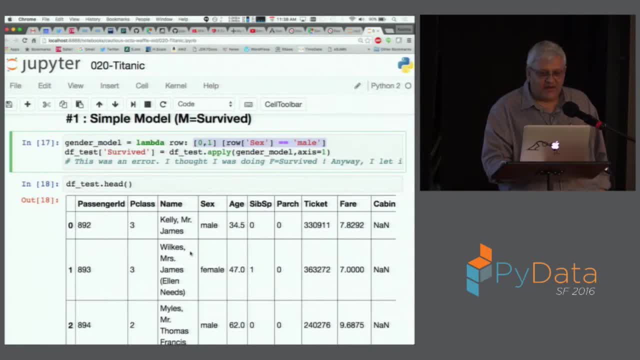 So you apply this model and you get a survived survived equal to all males survived. So don't go into, Don't go into the semantics, because we are not doing machine learning, We are just looking at how we can do the thing. 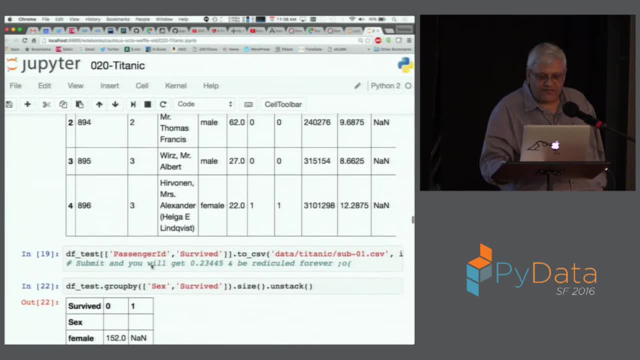 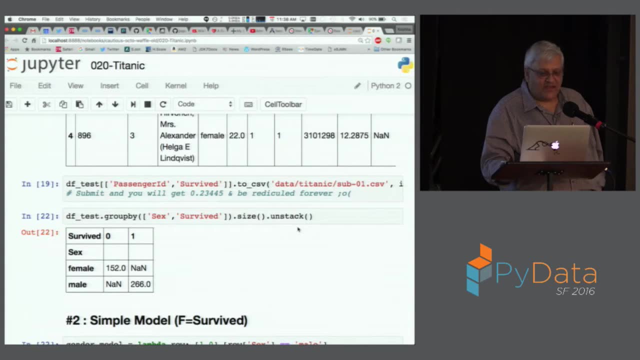 I wanted to point out one interesting thing on that one. So this is good, So let us do this guy right, Let us do the group by survived and size and unstack right. So what happens? You get this NAN. 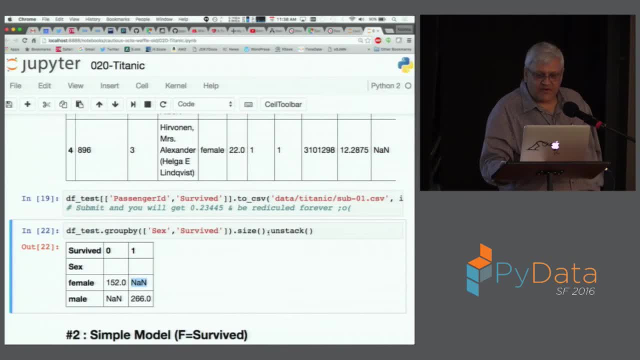 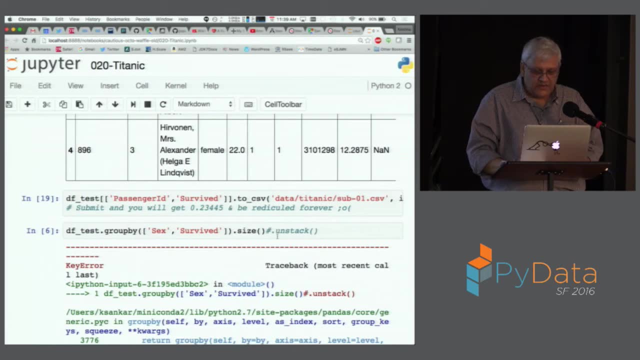 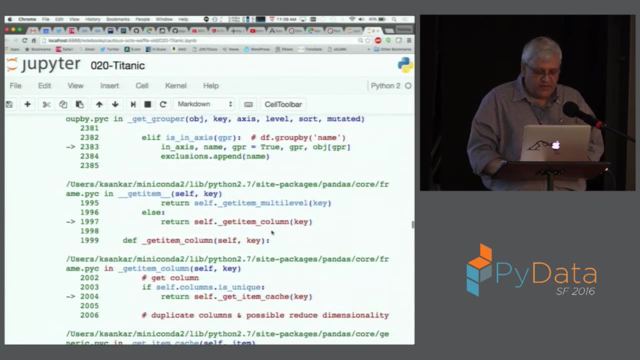 You know why? right, Because I'll show you why. right. If you do this Well, we are going to solve this problem. Let me show you what it takes. This is a good one, Probably. I hope that it is the error that I'm looking for. 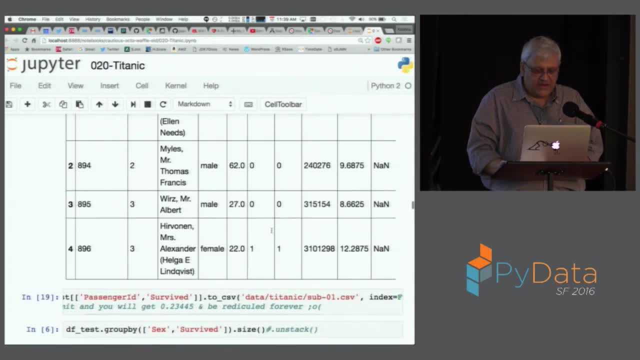 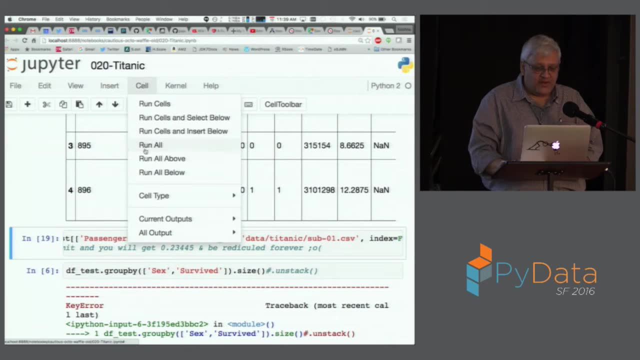 Here I'll survive, because I don't think I did this one that way, Because what I have to do is I have to go here and say, Because I haven't ran the thing, So what you do is run all about. This is an easier one. 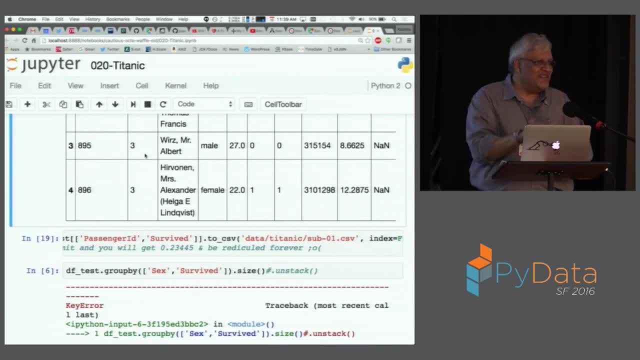 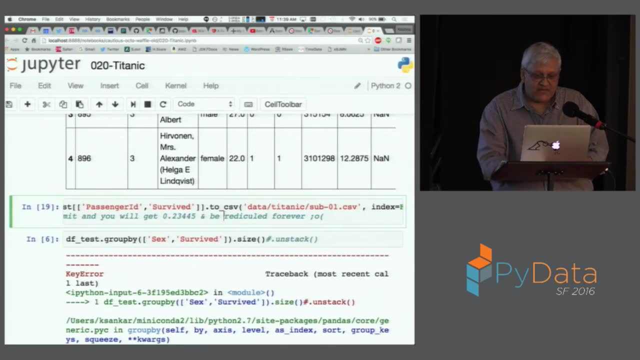 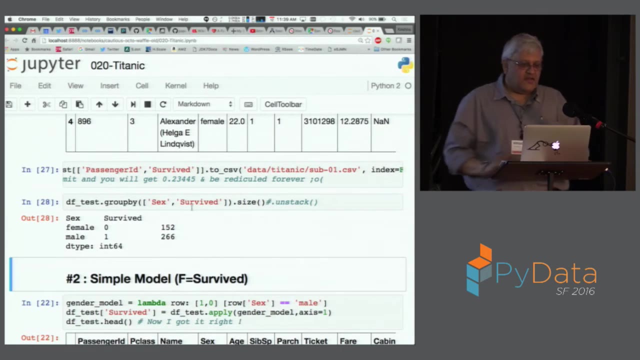 If you're running the 33 million one, That would take some time, So I would not run it, but this one we can run. So then, what we wanted to do was we wanted to do this one and size. So, because our model is that all males survive. 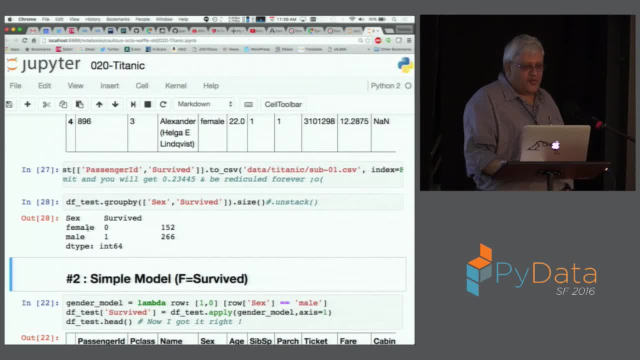 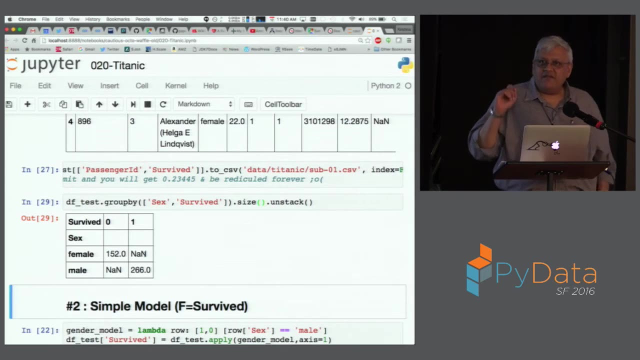 So you see this one. There is no female 1 or male 0.. So when you do unstack, what happens? You get NAN. The reason I want to point out is, when you do unstack, be careful. You will suddenly get these NANs. 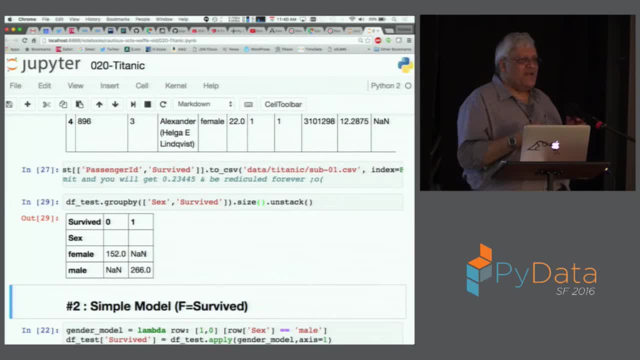 which were not there before, Because what happens is, when you are unstacking, you are taking all these things and putting it there. So when you do that one, there might be rows that are not there. You would not have seen it or you wouldn't have noticed it. 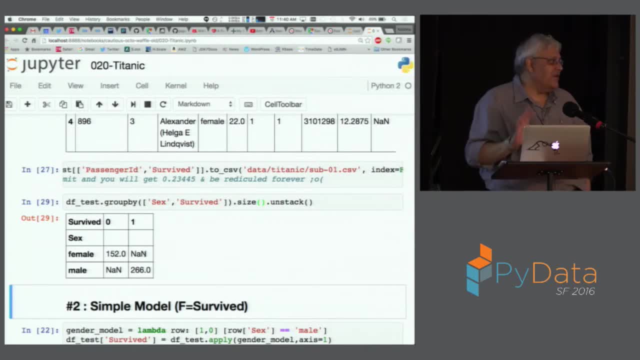 when you just Just use the earlier one, But when you do this one. so be careful. When you do unstack, NANs can appear. So once you do the unstack or things like that, you should check for NAN and you need to account for it. 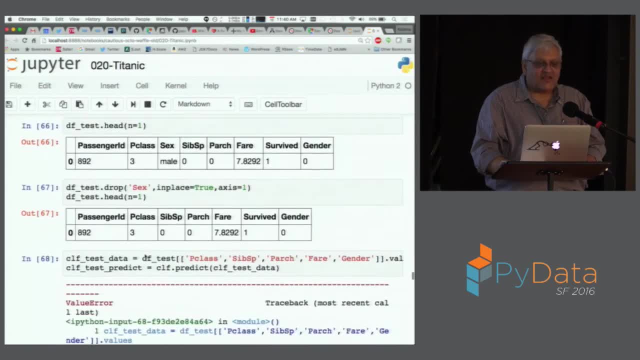 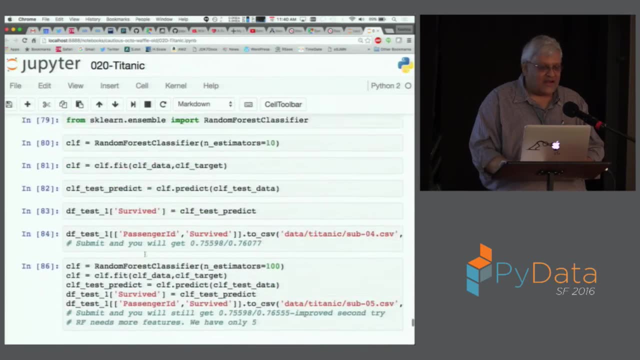 So that's all what I'm going to do on this data. There is more in here. I actually have done some machine learning and a tree and regression trees and random forest model and that kind of stuff. These are more on the machine learning side. 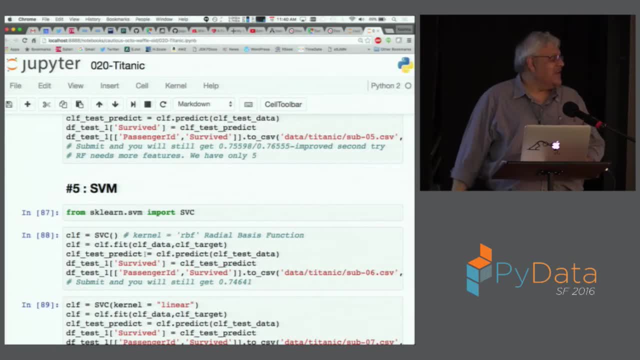 I'm not going to go through that one, But we have them here. You can take a look at it And if you have any questions, ping me I'll go through it. So this is good. So now we have gone through one data set. 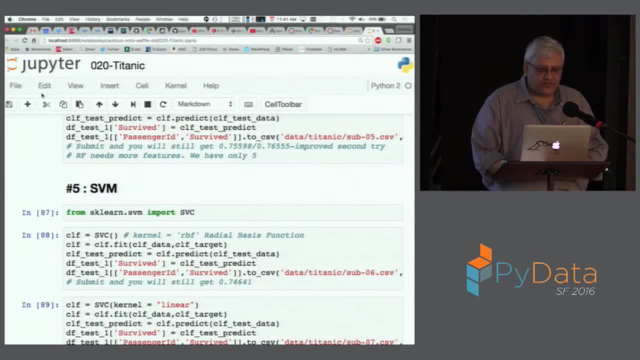 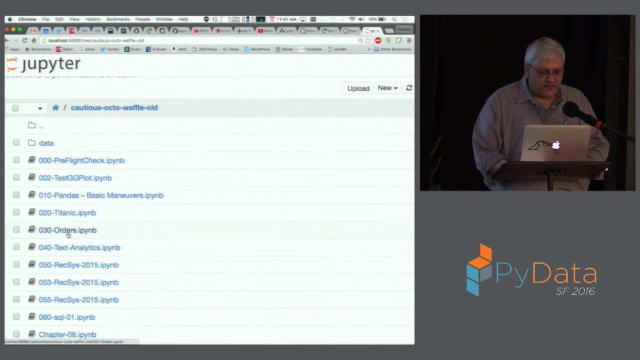 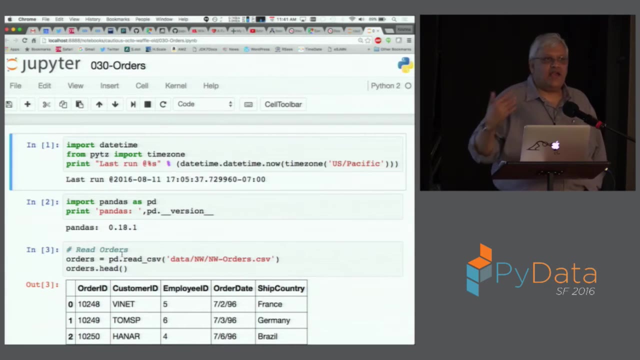 So let us go through another data set That is more interesting: the orders data set Right. So this particular data set actually has got a lot more, lot of history to it. Nothing serious, I don't know. There is this Microsoft Access database. 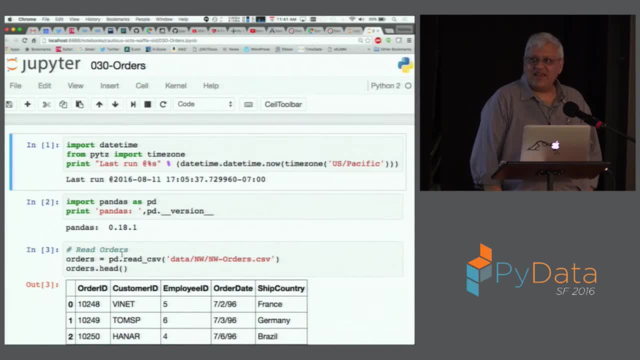 Remember they had some other database earlier as well. right, So in the very beginning that was the only database available And the Northwind- this is like people who sell things. this data set was supposed to be data set, but it's gone. 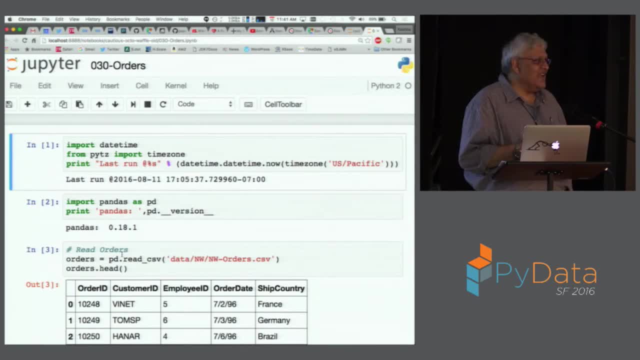 data set to teach you access SQL and that kind of stuff. This was years ago, probably 1990s or something like that, when dinosaurs ruled the earth and that kind of stuff. So then I saw this data set somewhere and I thought, oh yeah, this is an interesting data. 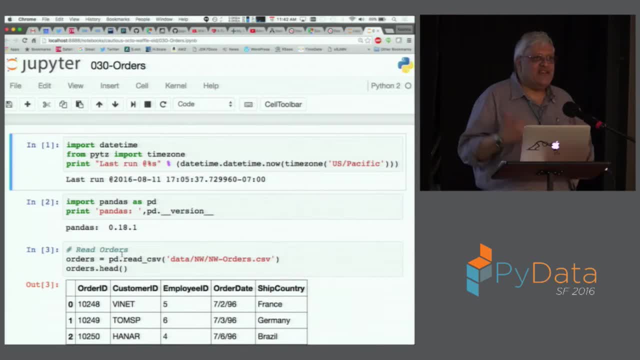 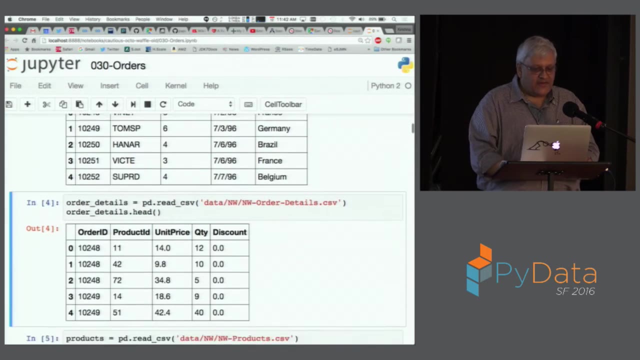 set Now, instead of doing SQL and that kind of stuff. I use it for Spark and Pandas and that kind of interesting. So that's where this comes from. The data set has. it has orders. So let us read the order data Basically: order ID, customer ID. 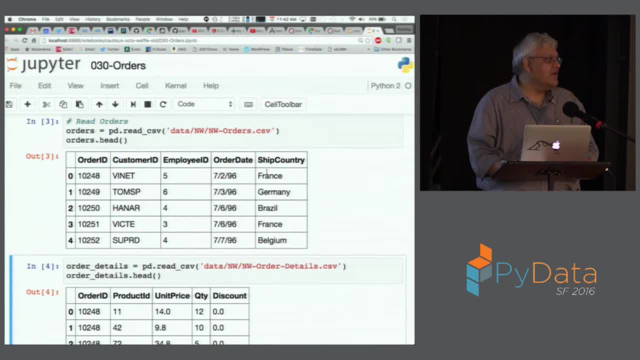 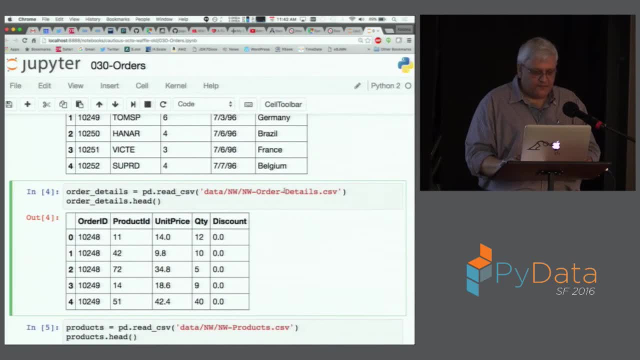 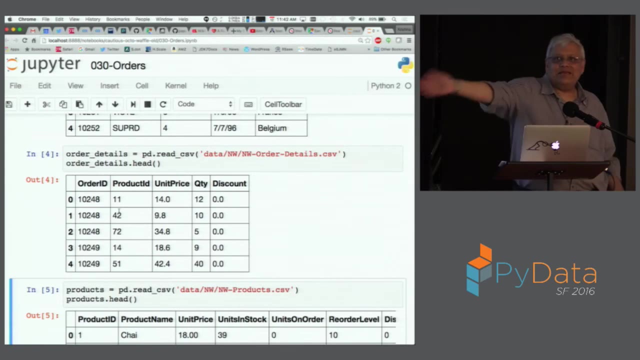 Order ID, customer ID. you have the employee ID, order date and the ship country. Simple So you have these orders. You have the order details, Order details have. so each order ID might have multiple lines. Basically, these are the lines in an invoice. 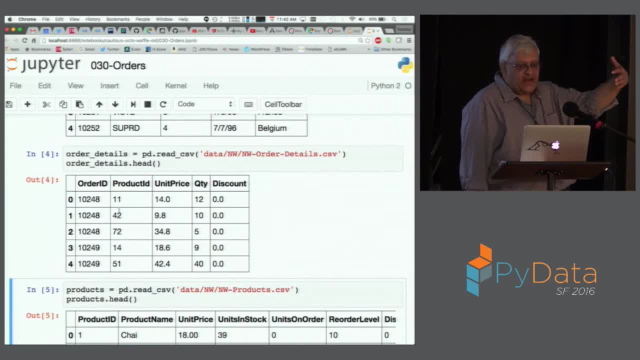 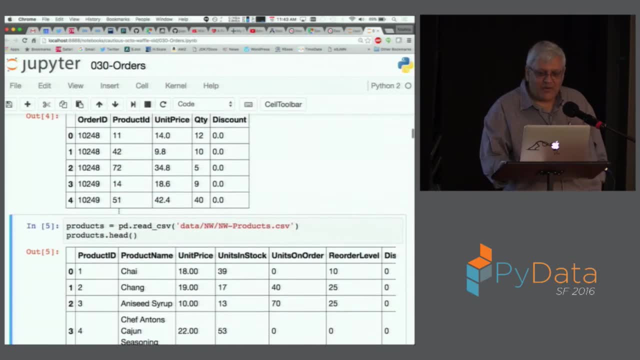 Right, You have the each order ID. then it says product ID, unit, price, quantity, discount, that kind of stuff. These are the lines in looking at an invoice And they also have products and various other things. We are not going to use the products here. They also have employees, So you can use all kinds of 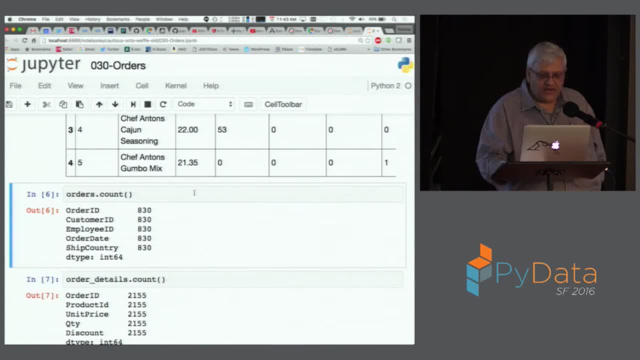 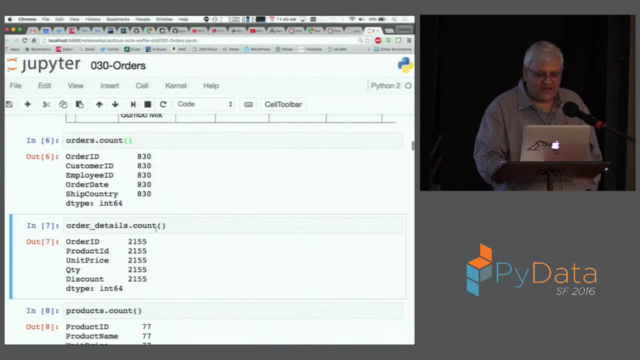 things in there, So it is fine, Good. So let us look at the data Orderscount. This is good, Right, There is no missing data, There is no impute, None of this. Details are good. So there is enough details. 2000 data. 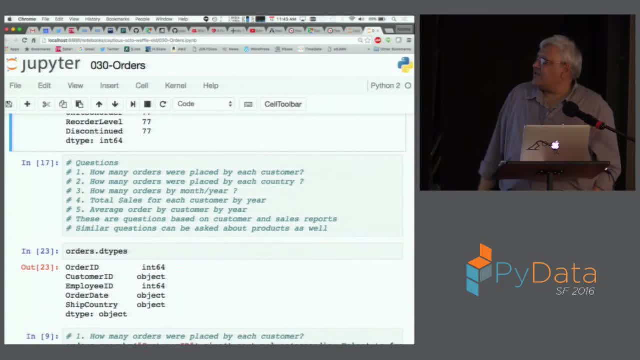 It is there. So now, these questions we need to answer: How many orders were placed by each customer? How many orders were placed in each country, How many orders by month, year, And then the total sales Right. That is what you will look at and say: give me the total sales per customer. 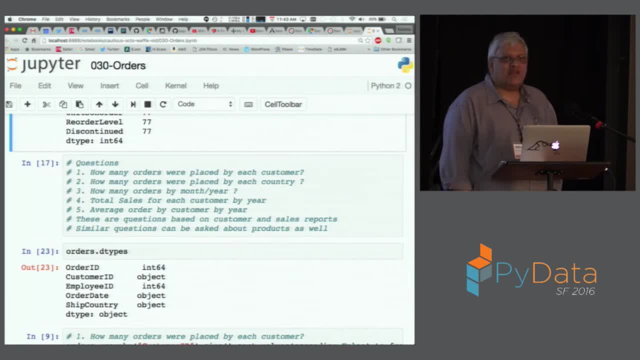 And probably give me the average order. Right, That is what you will look at and say: give me the total sales per customer, Give me the average order, But we have all these. So first question: How many orders were placed by a customer? 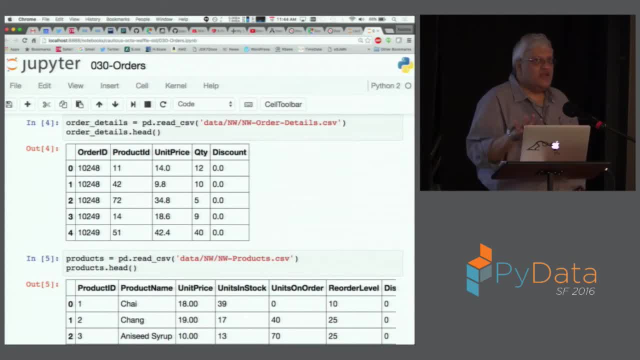 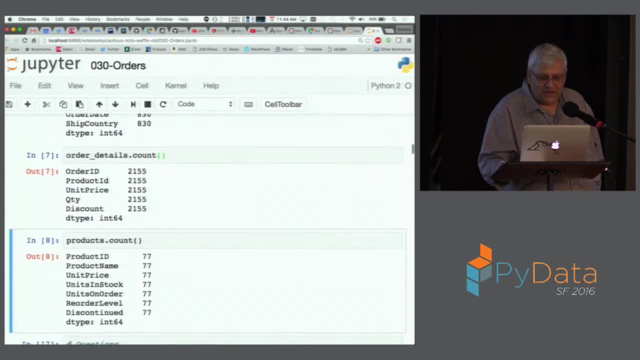 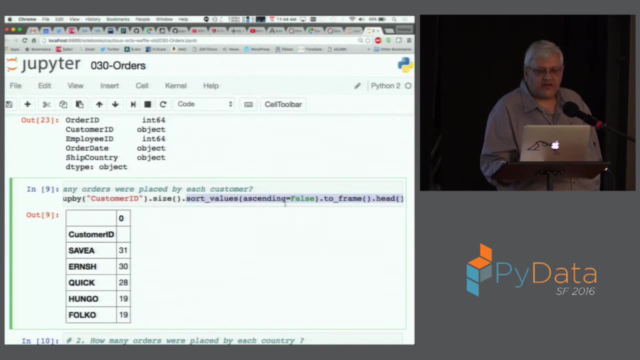 What do we have here? We have the customer ID. So it's very simple. It is a simple group by operation. A simple group by operation. You do the group by customer ID, size and sort value. So this is how you sort things in Pandas. 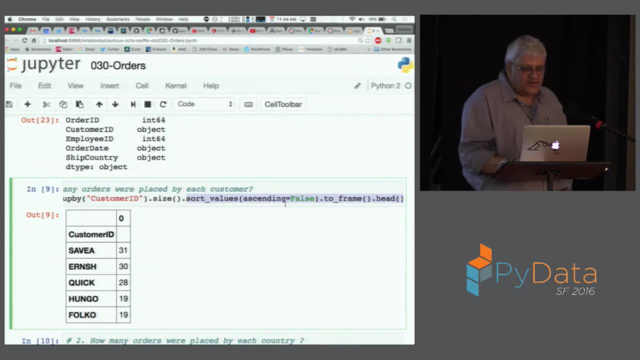 So you sort the values, because what you want is you want a large number of orders. Sometimes it makes it easier- is you just want to sort the values? so you want to get the customers who have the maximum number of orders. So you sort values, of course. 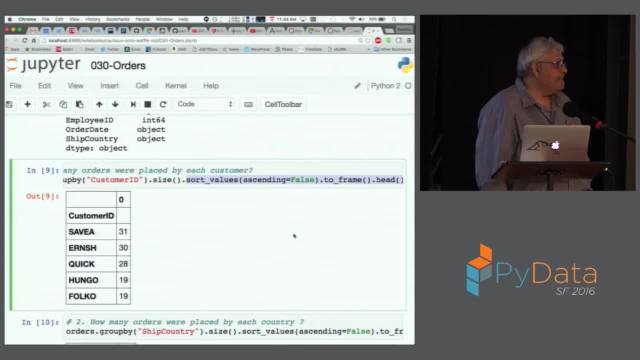 you get to a frame and a head. So it's a simple one, right? Does that make sense? So it's a group by. we have seen it before. you just group by customer, you're done, And then you do some sort values, that kind of stuff. 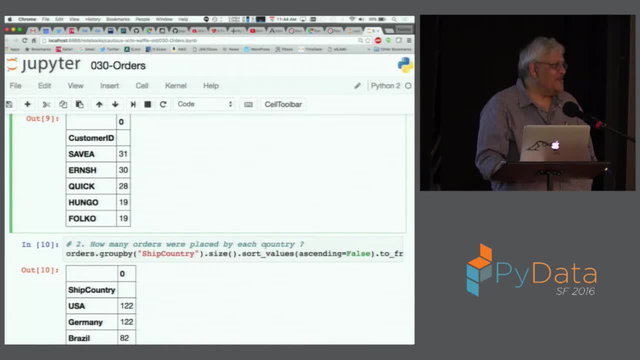 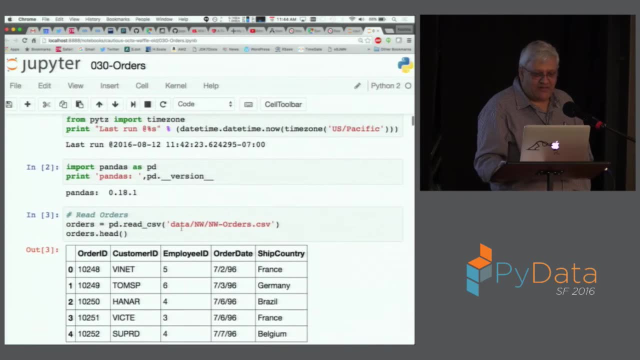 How many orders were placed in each country. Now we know how to do this one Right. It's a group by ship country, Because we have our data here which says you have a customer ID, you have a ship country. you are only looking at the number. 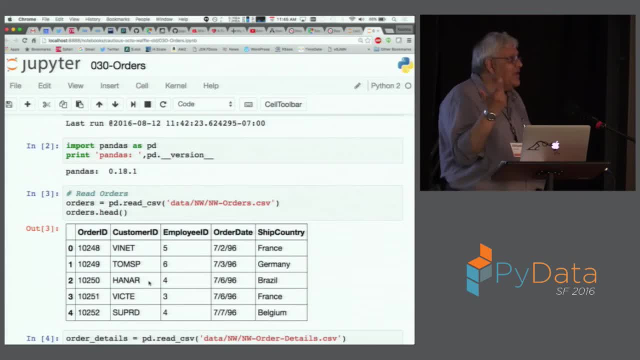 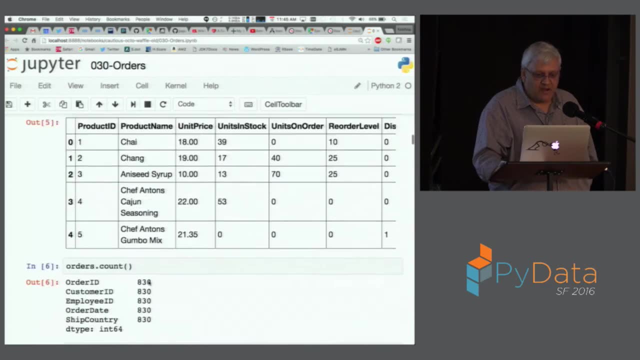 So that is why you use a count or size, right? You look at it and say, okay, how many orders are there for each country? You're done, It's an easier one. But once we get into the questions three, four and five, right, How many orders? 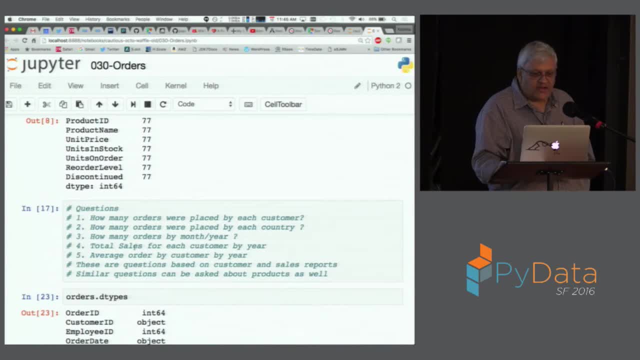 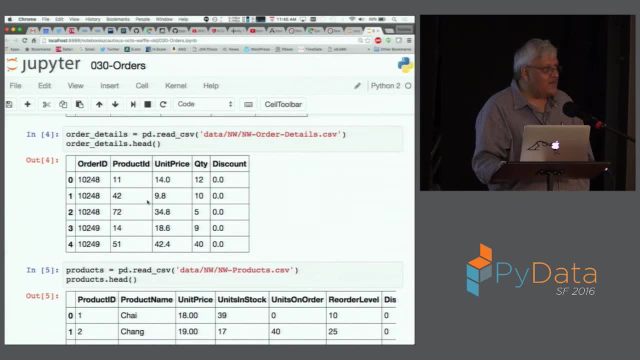 per month, per year, Or give me the total sales, So give me the average order per customer. Now we got a problem, right? Because this doesn't have two things. it doesn't have. It doesn't have any date thing at all, right, It doesn't have. 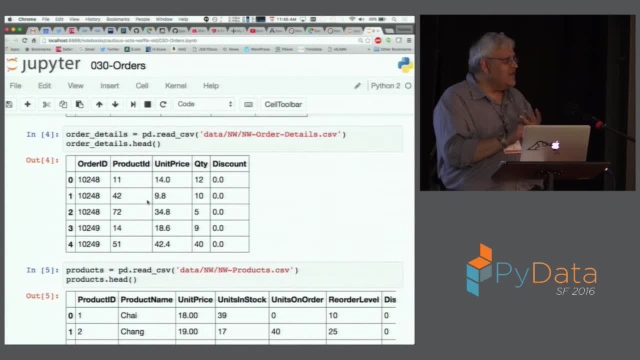 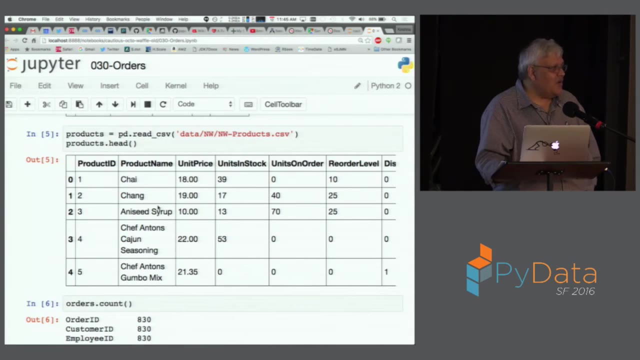 any date thing to get month, year thing, And it doesn't have anything to say. what are the total sales per customer? how many things did they buy? how much dollars they bought? right, Those things are here in the order details. So now, 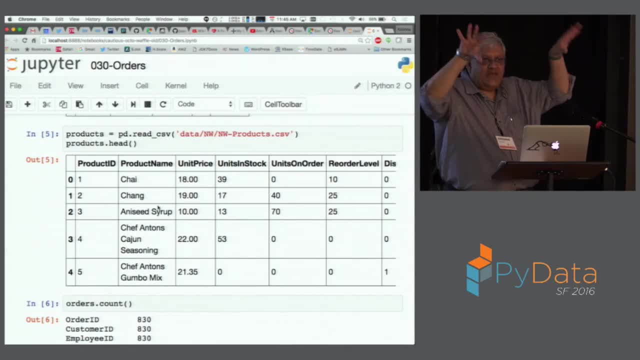 this thing is: do Panda's thing on the order details, get the various information out of this guy, put it back into our orders, this thing. then we know how to do it right. Then we know how to do the group buy. So let us see. 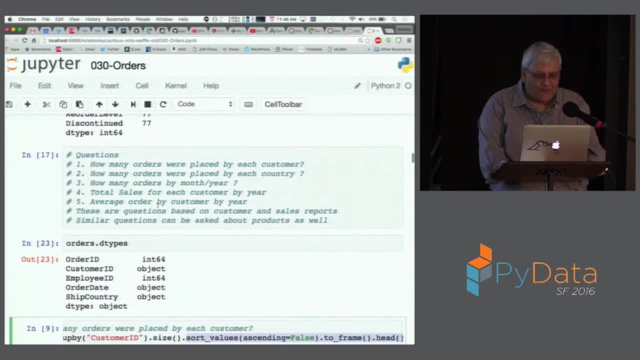 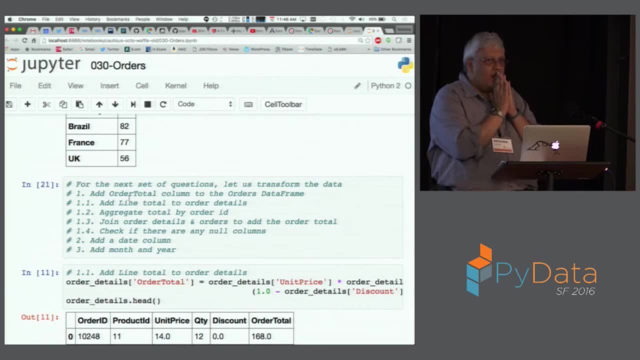 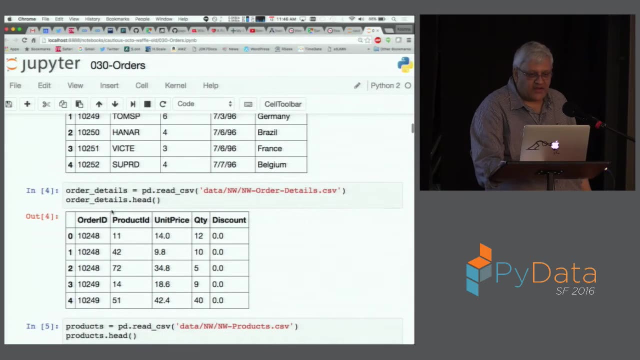 how we start doing that one. It's not that bad. Step number one We have in our order details. order details is a strange table right. It has this product. Sorry, that's this guy. Hmm, I see chai here. Actually I feel thirsty. 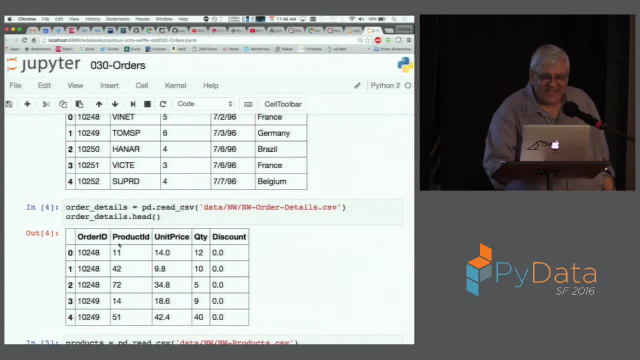 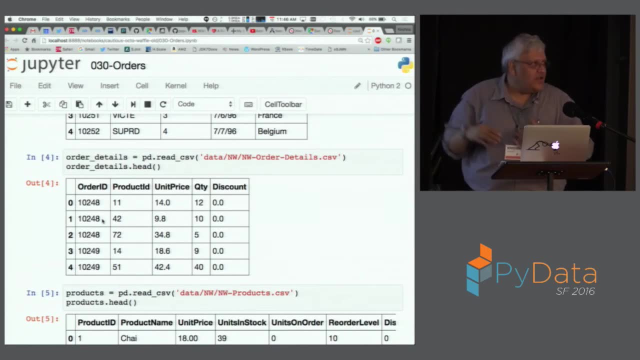 to drink some chai. Maybe we should do it after this is done- See this guy order ID. right, You have multiple lines in an each order and you have the price, quantity and discount. First thing we do. what do we do? We get the total, we get the. 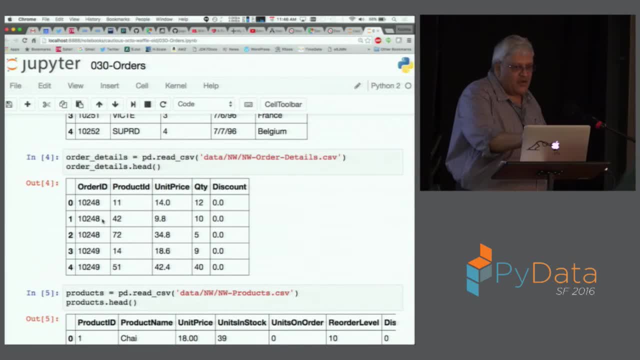 you know quantity price, so you get this total, this thing right. Unit price: you know quantity star price minus discount thing right. So you get the unit price here and then you need to aggregate it for all the orders. 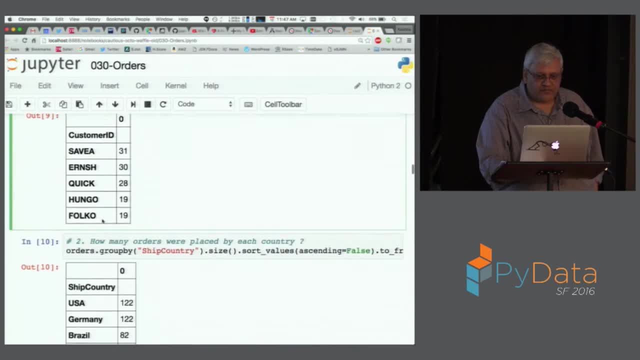 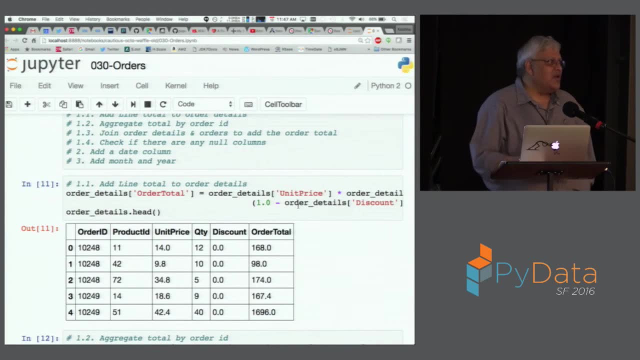 So that's not that bad. You go in. Go in here First. you add the order detail. Order detail equal to unit price star. Remember, all these multiplications and things like that work on a column, right? They are not working on a single piece of this thing, right? 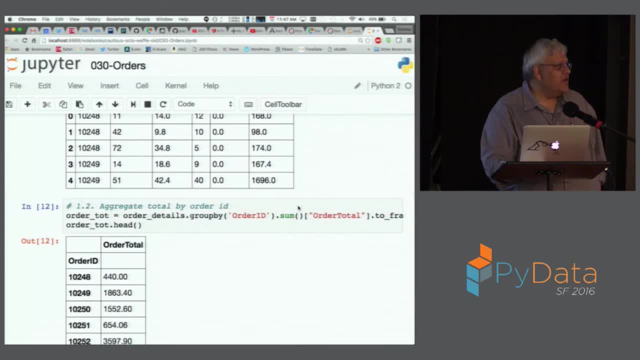 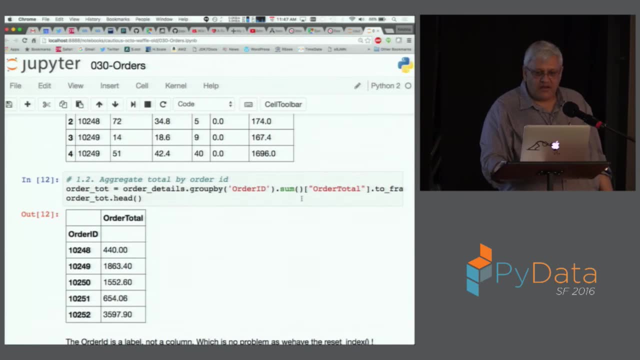 So you do this one, and then what do you do? You aggregate by order ID, right? When you aggregate by order ID, you get this total for each order, right? So now, group by order ID, and the thing that you use is: 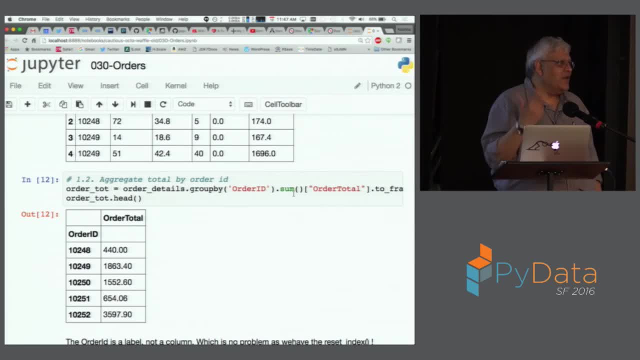 sum right, Because now you want the sum of all the orders. Do the sum, You have the order ID and the order total. So what do we do next? Yeah, no, I mean, what we do is we do a join to the top right. 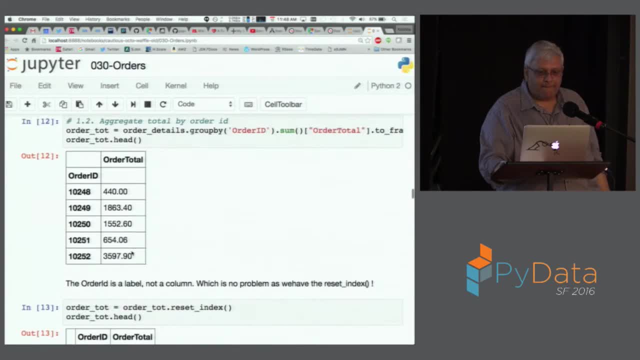 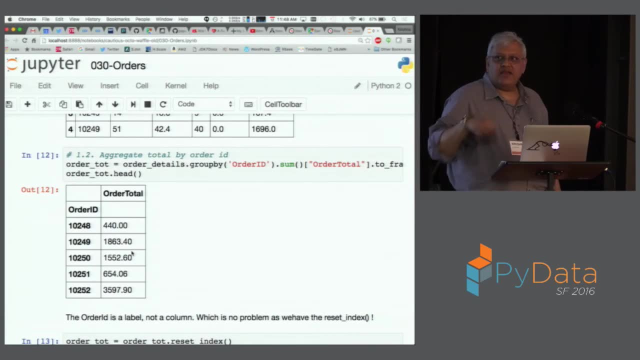 So this is where the merge comes in, right? Oh yeah, This one has a slight problem: This order ID thing, right? What is that order ID thing? That's a label. That's not a column, right, Because pandas. 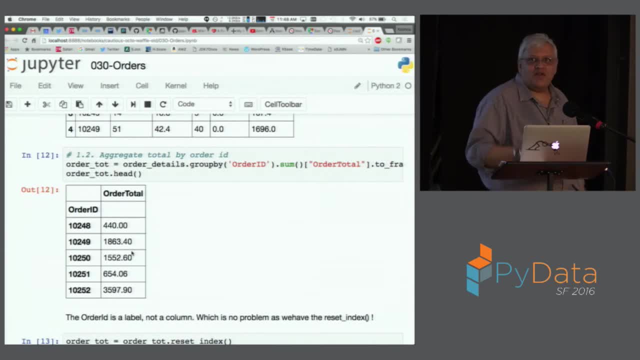 remember: this thing has a. this is a row label. Remember this. we were asking about ILOC, for example. right, If you do ILOC 1, you will get 440.. In ILOC 0, you will get 440, right. 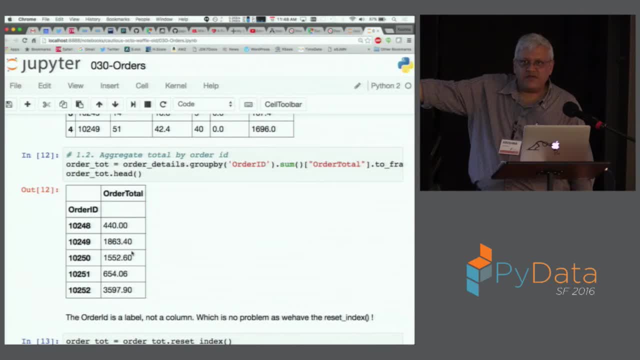 But if you do ILOC, if you do LOC 0, you will get nothing. You have to say LOC 10248, because LOC is a label, right, ILOC is a position. So this is where the ILOC and the LOC comes in the picture. 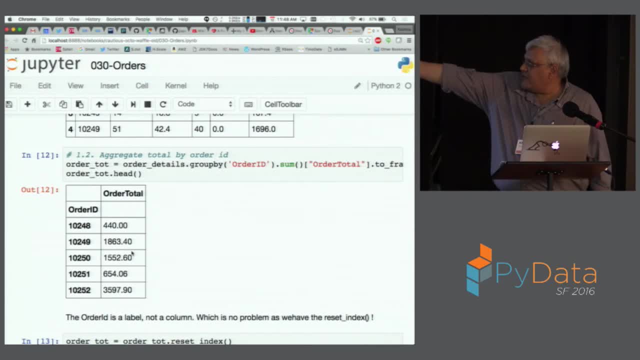 But going back, all those guys right, 10248,, 249, these are all labels for this guy. If you want to join, how do you join? So what do you do? There is a thing called reset index. When you reset index, this is like that. remember we were talking. 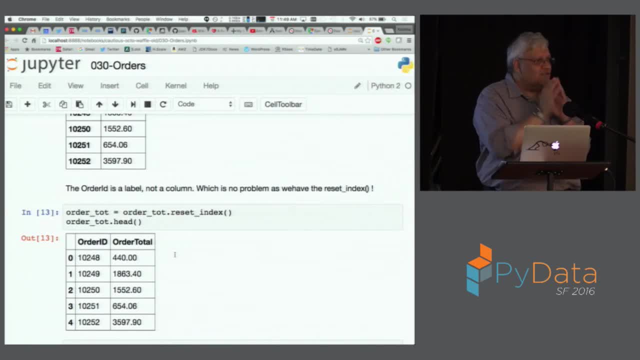 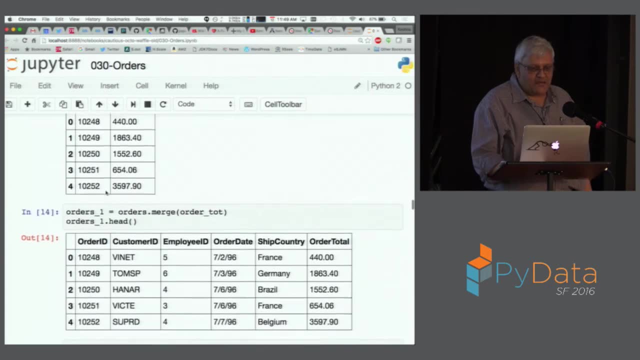 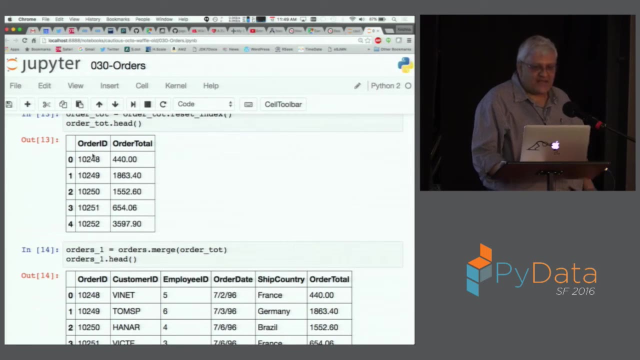 about this? what was that thing? Unstack, Similar to the unstack. suddenly, this labeled multi-index is a single index, but multi-index. this thing becomes a. see that now I just gave you this number right: 1,, 2,, 3,, 4,, 5, this is just a number. and then 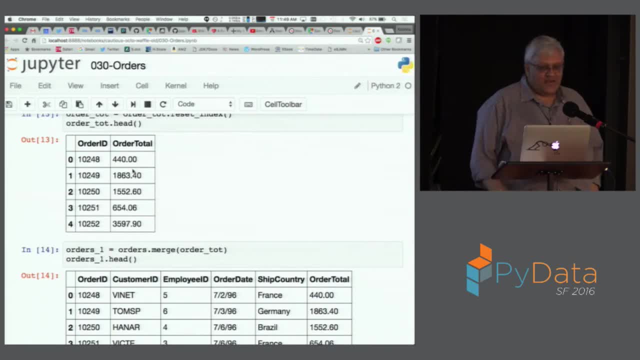 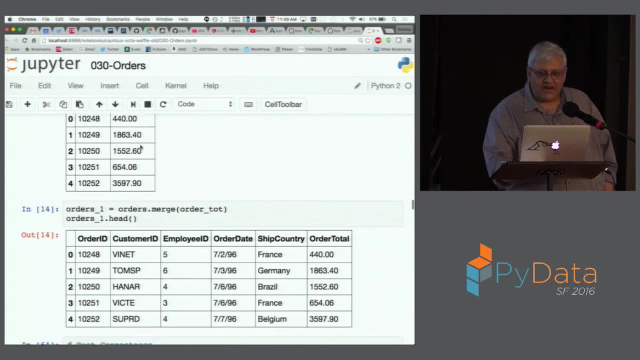 order ID became a normal column. So now you can go back and say: merge. What you are going to do is take this thing, merge into the top one and voila, you have your order total for each customer. right Now we. 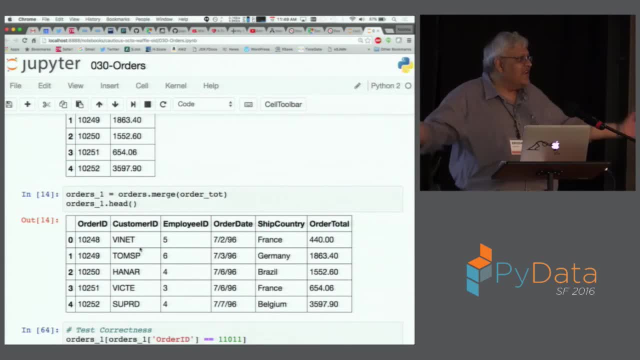 are in good shape right Now. we can group by customer, we can group by country and then we can get the total: how much this thing people came. and how do you get the average per customer? Instead of sum, you use average. Remember the group by is. 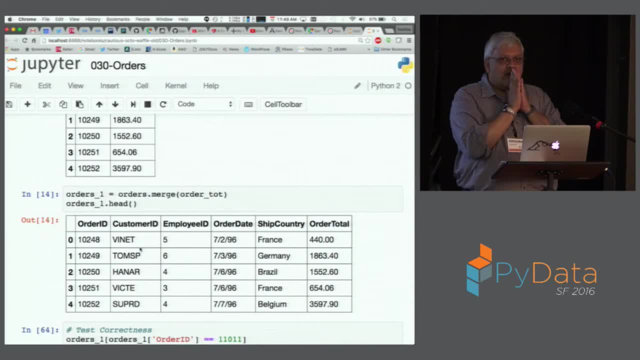 nothing but a. what is that? You know, apply and right, It's a map reduce thing. right, Split, split, apply and come by right. So if you just get a group object, it will split and give it to you, You can apply. 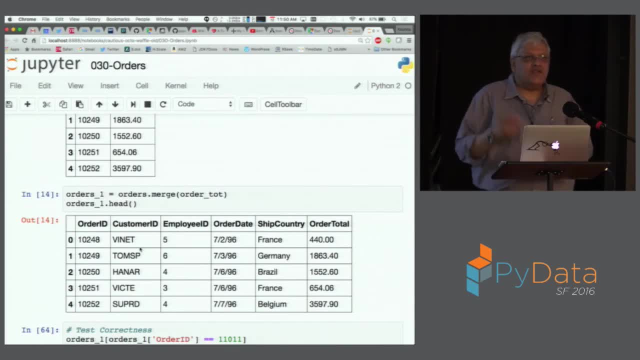 anything you want- I mean, it's not anything you want. you can apply things like size, group. you know size, average mean total sum, et cetera. right, So when you want the average, we take that thing and apply the average. If you want the total, we take that. 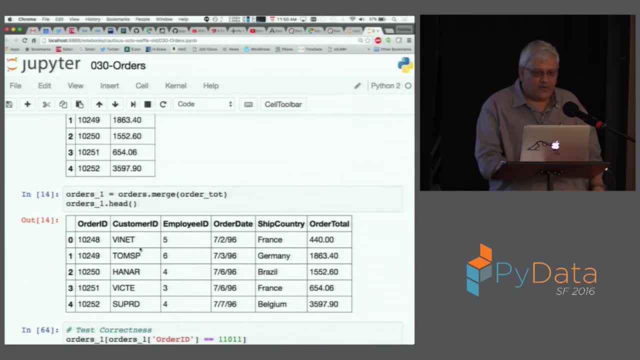 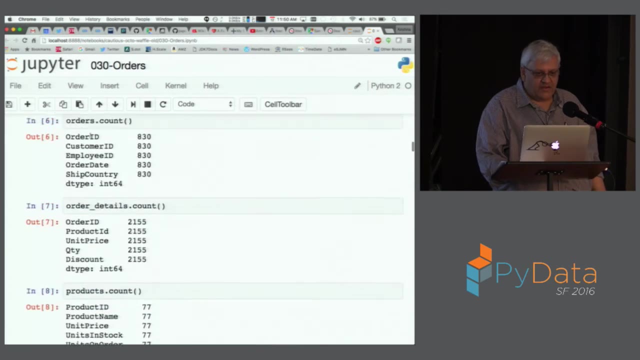 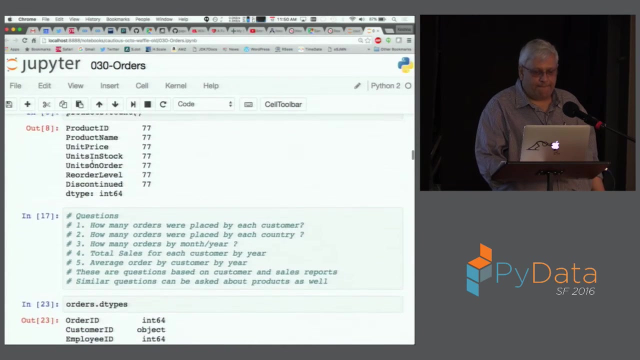 thing and apply the sum on it, And that's exactly what we do. We do the. did the merge make sense, guys? No Merge on order ID. See what happened is we had which one? Yeah, Excellent, excellent. 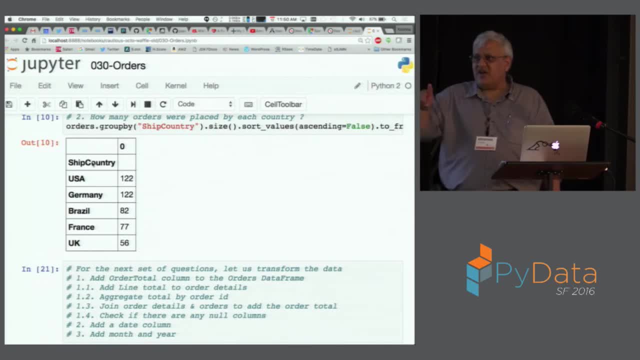 It is by default. It's by default, Hold the thought when we do another one. So it can be default. or you can also give and say left on and right on, and you can give the column name as well. So pandas is so, thank you. Thank you very much. 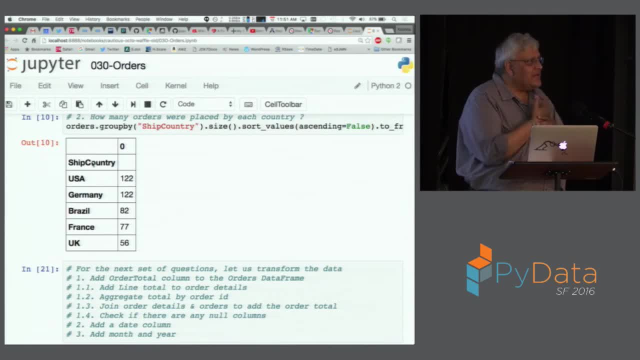 The question was: is it by default, right? That is a good question. The reason that is a good question is because you have two data set and if you have the column names, the same pandas will figure it out. You don't have two. 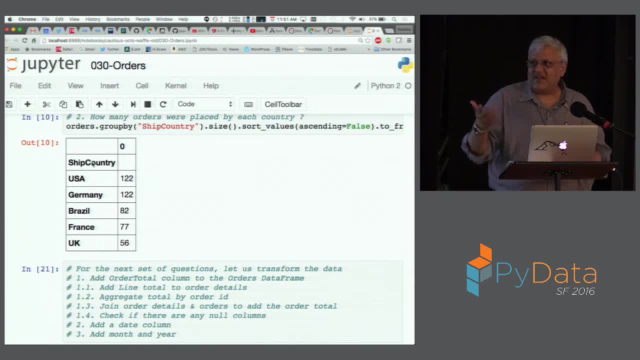 Give it things right. So these are some of the things that it does right. It does that extra step of going: yes, if you have, you know, if you have some two names which are same name but different data, then we are in trouble. 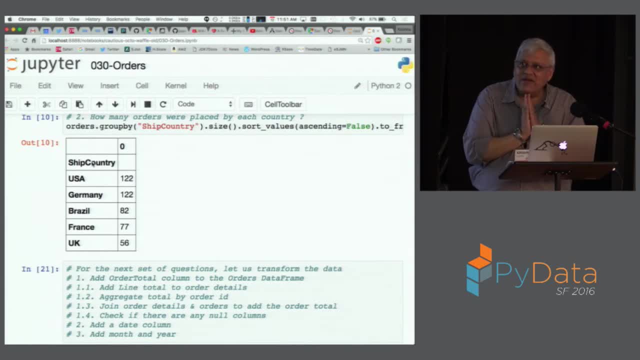 But most probably that shouldn't happen, right? One of the basic tenets of data science is that the you should, you know, you should always name them correctly, right? Whether it is on this table, whether it is on that table, whether it is some other table, you have to name it correctly, right? 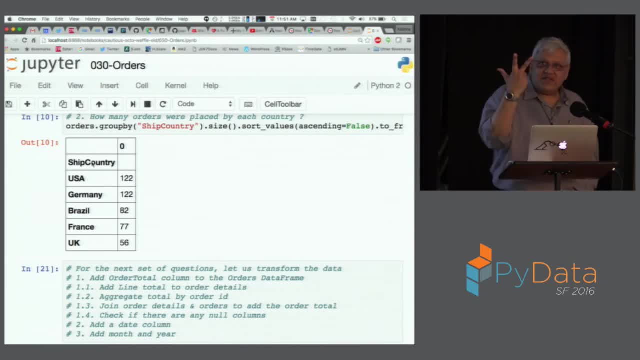 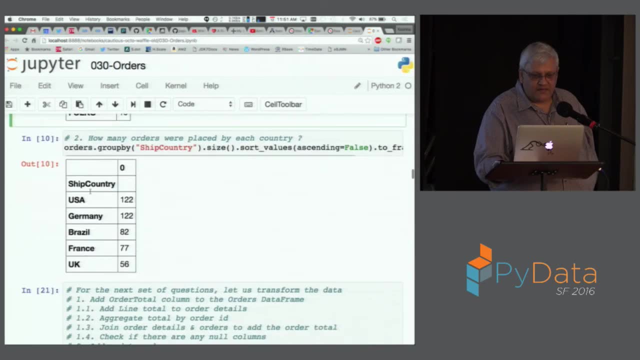 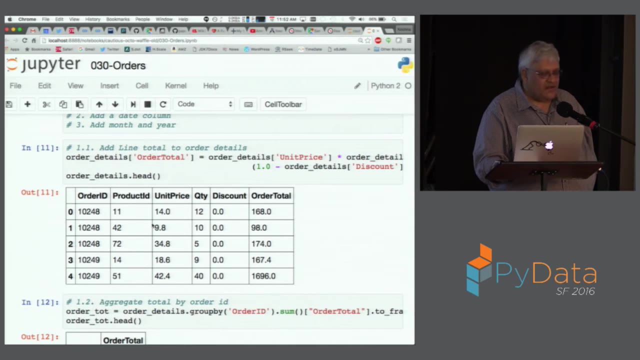 I mean name it appropriately, because if you have same name saying two different things, you are in deep trouble. So so, going back, we have the order ID, product ID. this is our, this is our details. From the details: 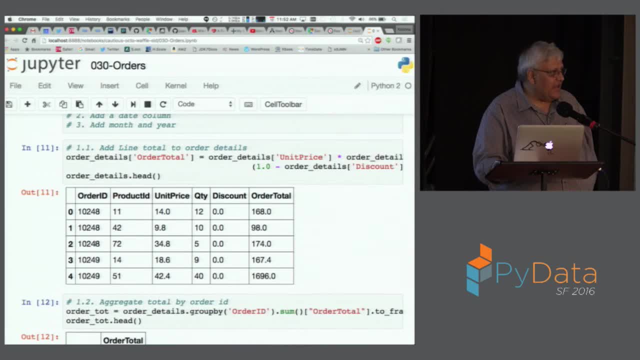 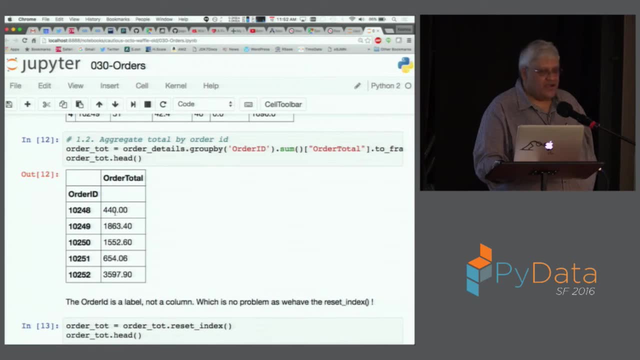 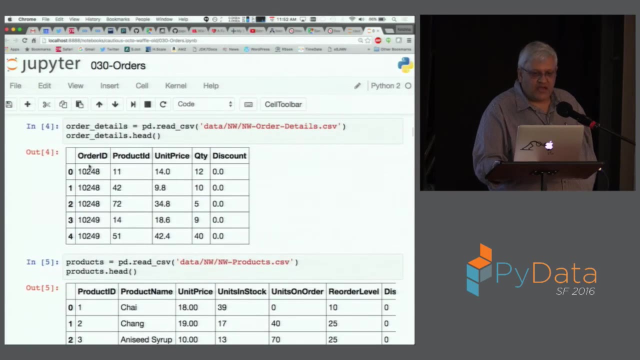 we sum up the total for each order ID. So we get a table which says order ID and the total dollars for that order. We take this table and we go back to our order's table has order ID as well and then we tag in that order total here. 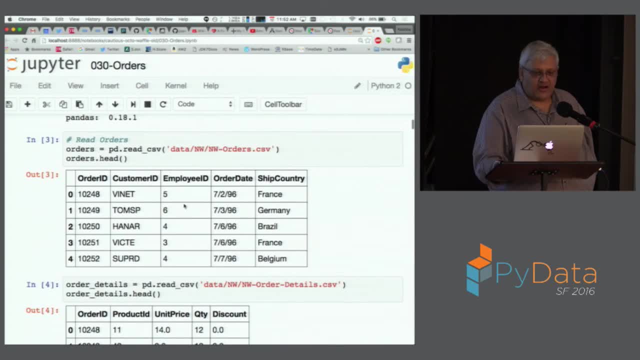 Right, This is the details. This is the order header. Right Order header has the order ID, and so we get the total here. So suddenly we get this nice table which has all these things, And so you see how we were able to get in. 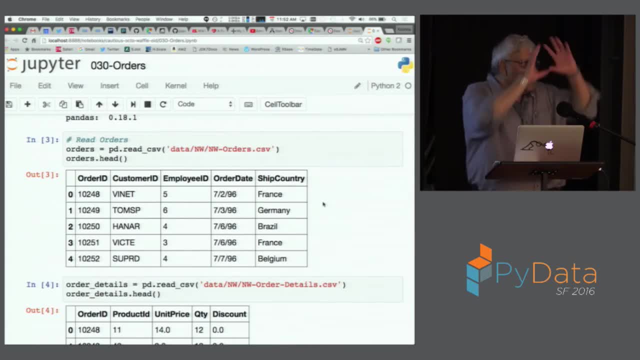 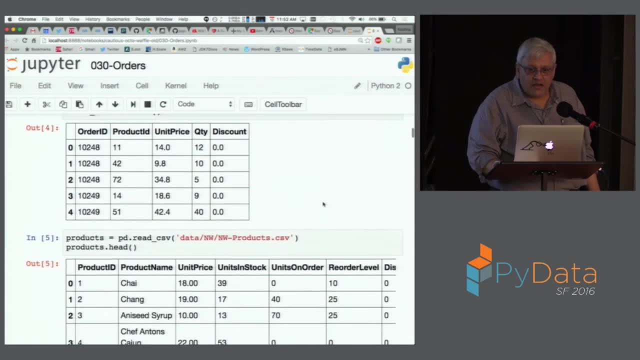 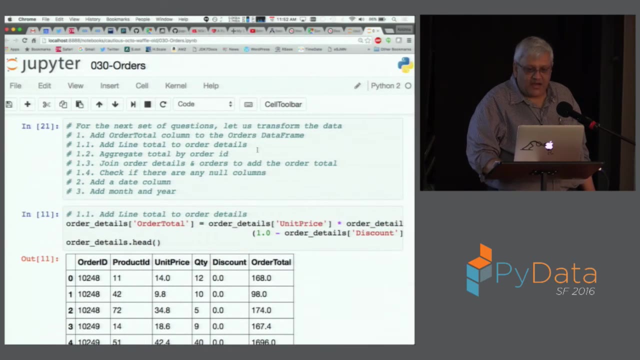 we were able to gather all these things from multiple tables, take these things up and then put it in there. Right Now we, we need, of course We need in our question. you know I'm going to go a little faster, but our question is aggregate by, you know, by month and year and that kind of stuff, right? 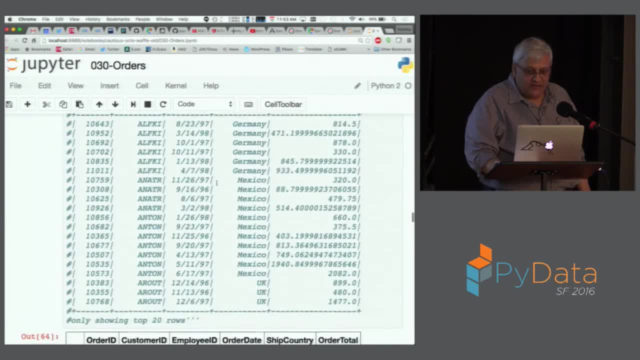 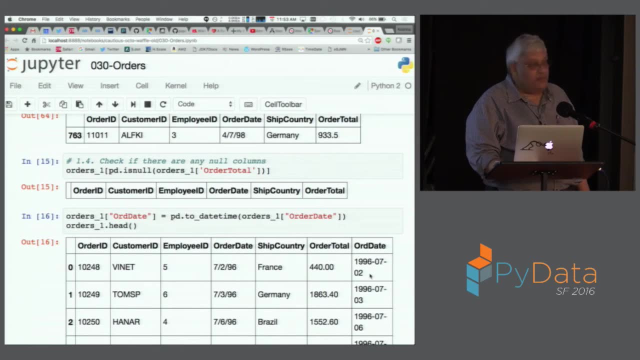 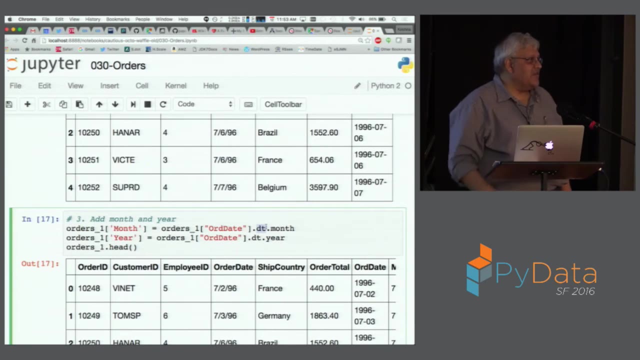 So by month and year. what do you do? You have the. you have the order date right. Turn the order date into a date time. We do the date time, turn it into a date time And then remember this DT- remember I was talking about this- is this name space which has all this date time. 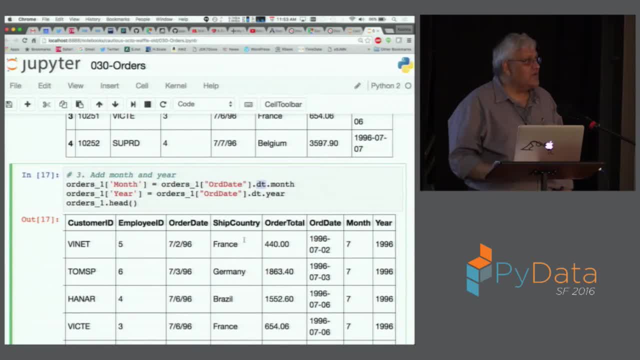 We get the month and year out of there, right? So suddenly you have two more columns, which gives you month and year. Now we are, now we are in good shape, right? We can answer all questions. Give me by. give me all customers. total of all customers by month and year. 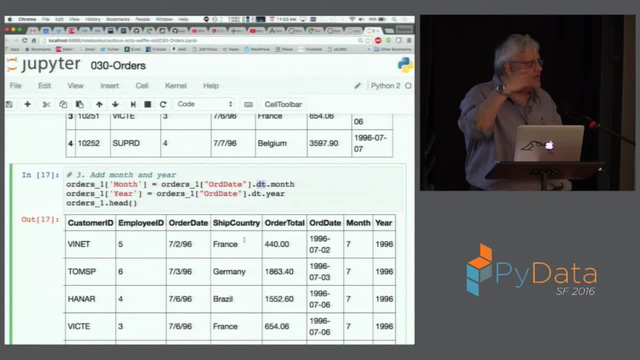 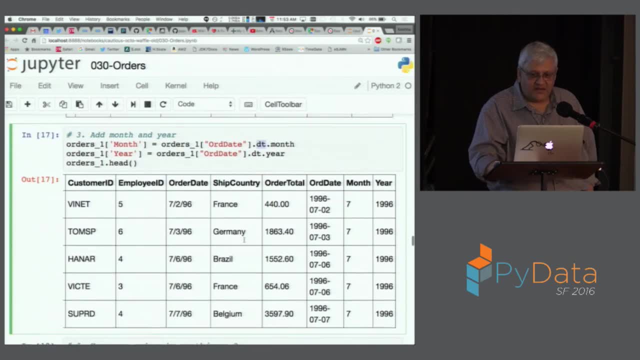 What do you do? Group by year, group by year, month, and then sum right, Because you want the. you know, you want the, the, The, the, the total right. That's exactly what we do. No, no, sorry. first is how many orders? 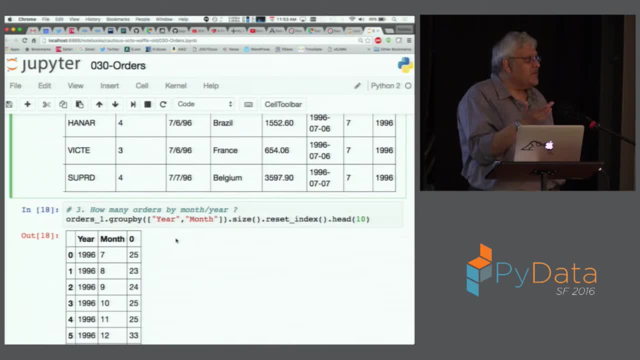 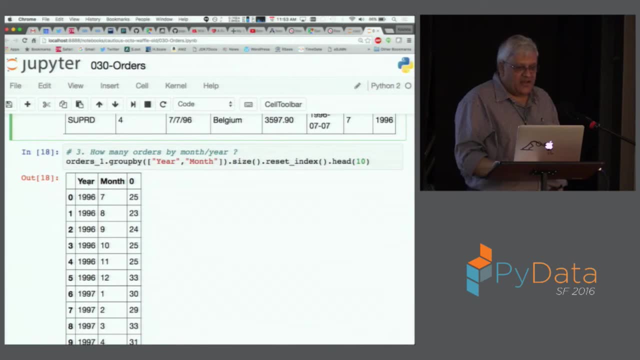 So if you want how many orders, you do the size right. You say okay, how many number of orders for each customer, grouped by year and month? See that one. This is where the multi-index comes in, right. You have the year and month and then I did the reset index and head so that you get this nice data frame model. 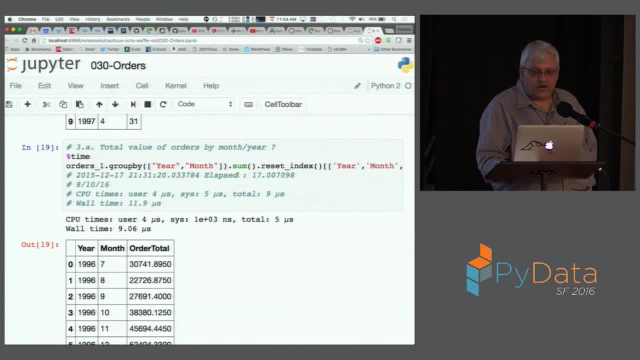 Now the total. if you want the, if you want the order total, you do the sum. remember the the. The thing is: you come, you know, you have the split, you split by group, so you have these records packed by the group and then you can apply the functions that you want. 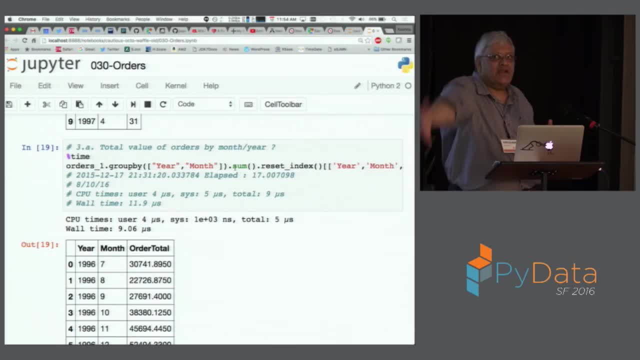 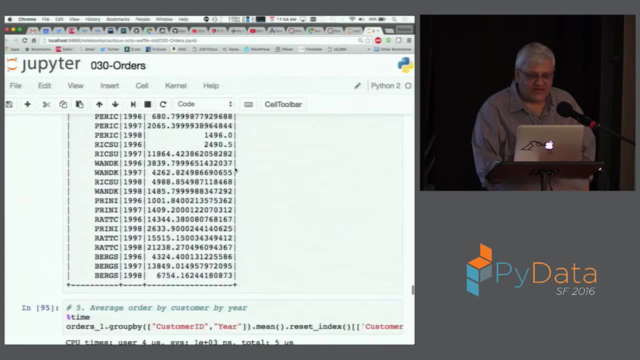 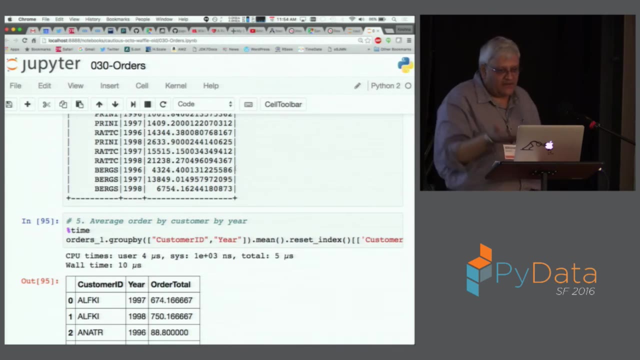 You can apply size, then you will get the number of orders. If you apply the total, you get the total of the business and that's about it, right, The, the, the. then you do the rest of the stuff- average by customer instead of total. and this thing you do, the average. you do the group by customer ID and give me the average and you're done. 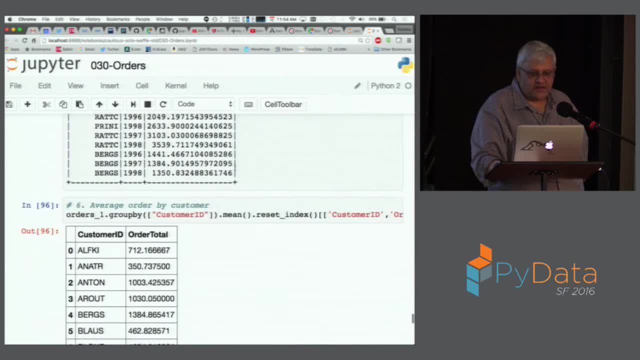 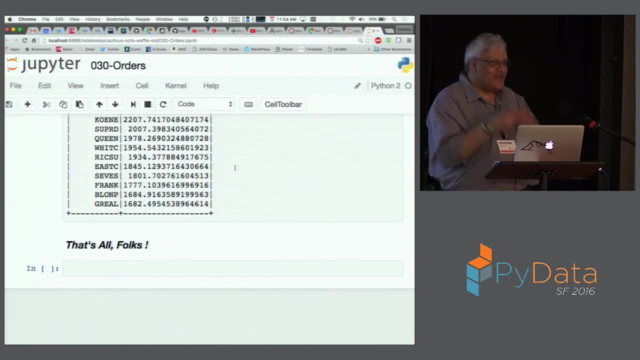 And you know so. so now that you you understand the group by and this thing, you can do all kind of manipulations with it, right? You take this one and also see, remember the: the merge the group by this unstack reset index. if you have all these things, you are in good shape. 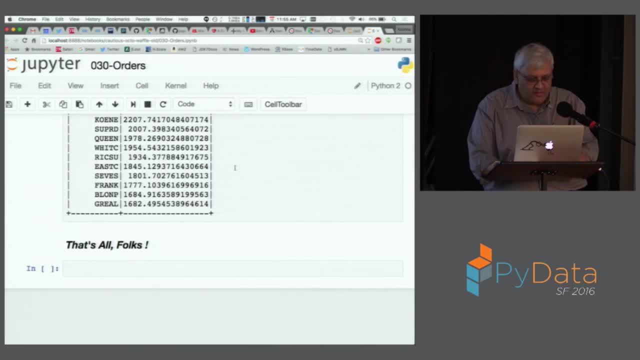 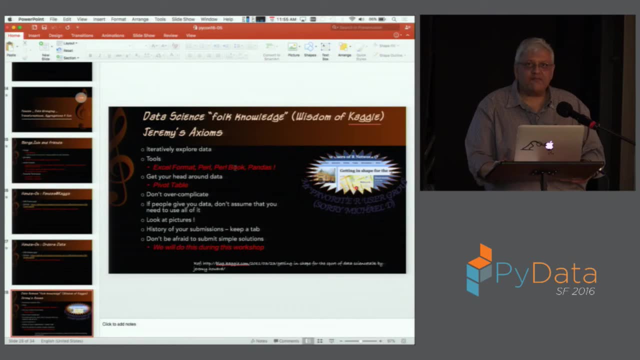 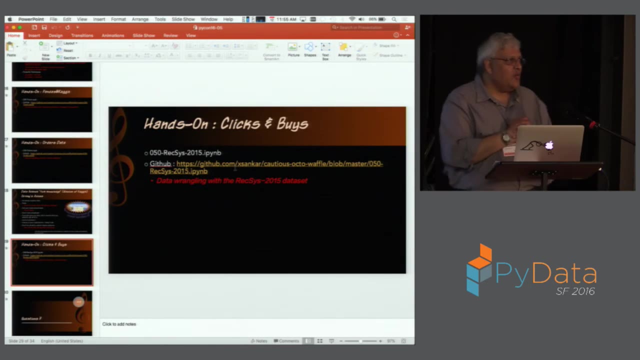 Does that make sense? We have we. we still have enough time. Let me see how I am doing on my time. Yes, excellent, So 20 minutes actually. So so now let's do some serious business, right? 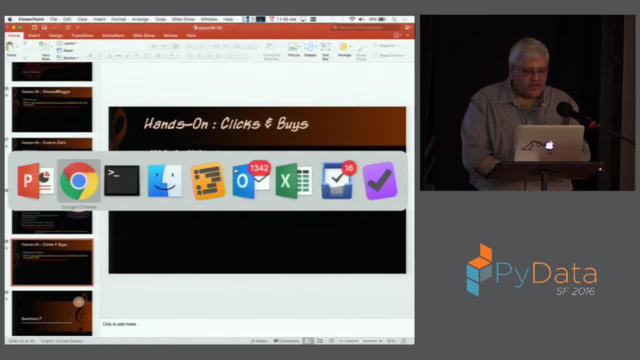 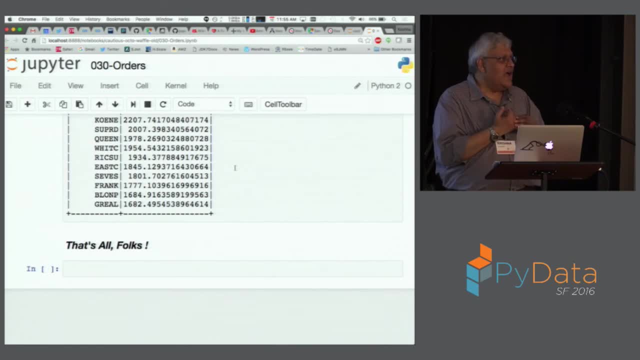 So this is the, the recommendation systems. You know this is a like a RECSIS conference. Usually that happens every year And during the conference there is also a challenge, So that people, you know, do the challenge and then there is a actually RECSIS challenge itself is a. 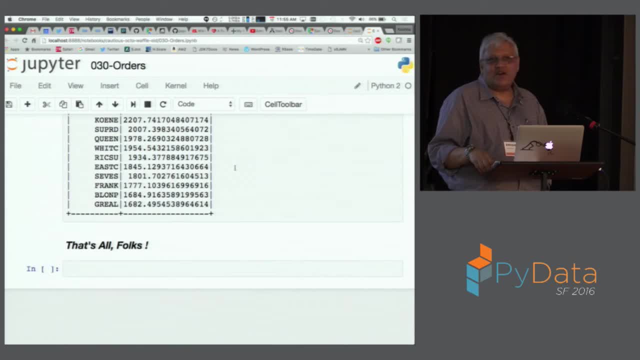 You know is a track by itself. then about 10 or 5,, 5 or 10 papers of the people who have done the top, this thing, you know they discuss how they did that one, et cetera, et cetera. 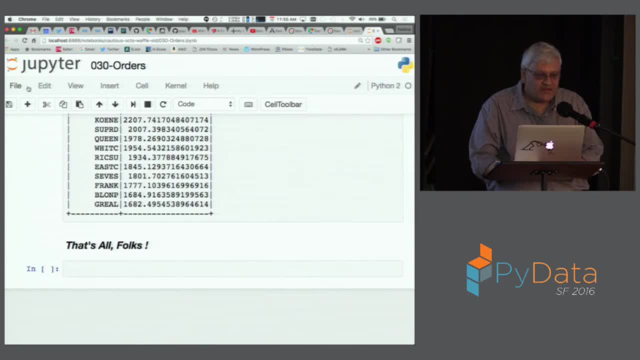 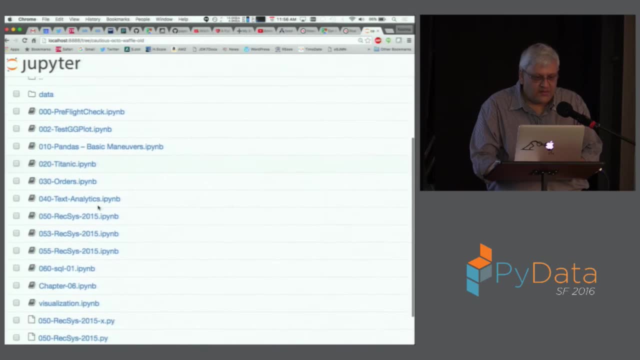 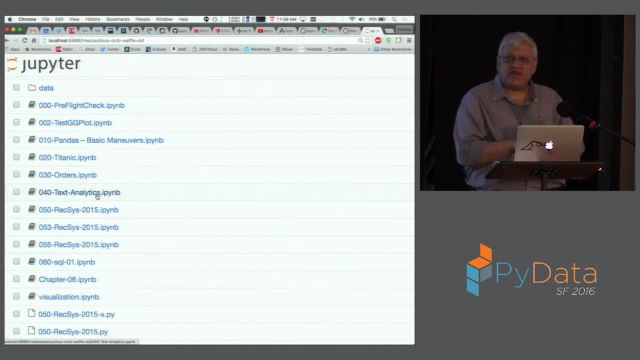 So let us take that data, So let us get this guy out, So let us. so there was another data that I was going to use. This was the text analytics. So the text analytics was interesting, because what the thing? 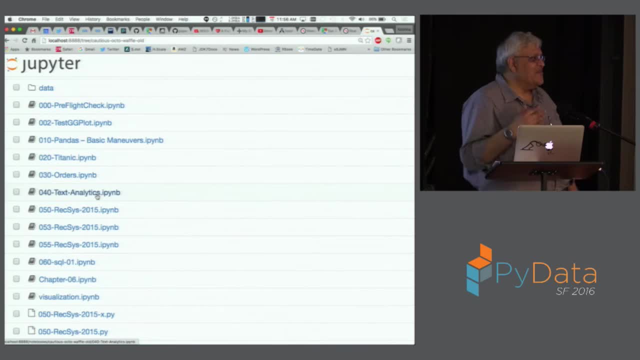 I'm. I'm still, you know, but I didn't. I know that I didn't have to get time, so I was not going to attempt it. The idea was to get the the state of the union right, So the state of the union by the presidents. 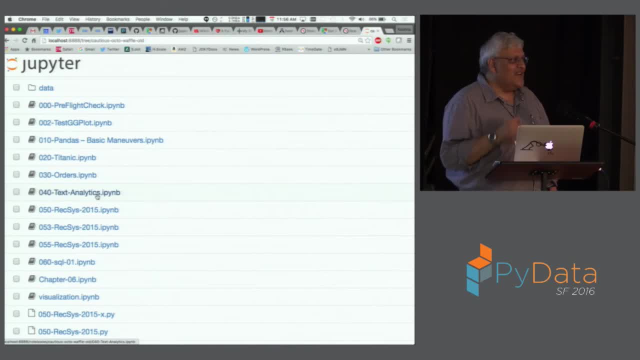 They reflect the times, right? George Washington was not talking about WMD, right? He was not talking about Iraq, right? So, if you look at the state of the union, analyze this thing, get the number of words, the top, top, top words, you'll know. okay, they were talking about union and they were talking about freedom and things like that, right? 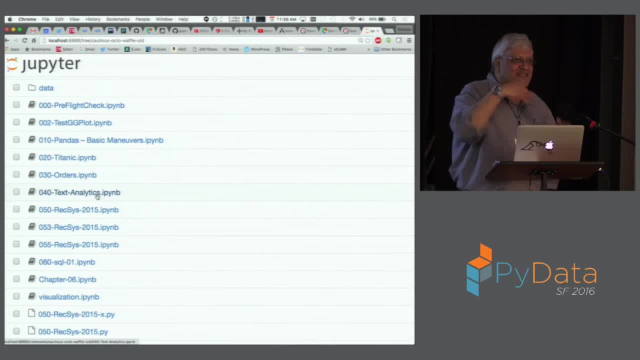 Now we don't care about any of those things, right? So, anyway, so, so, so, that is that side of the story. So so I have the state of the union we were able to, and then we were able to compare and say: what did Bill Clinton say that Abraham didn't say, Abraham Lincoln didn't say, or what did Abraham Lincoln say, right? 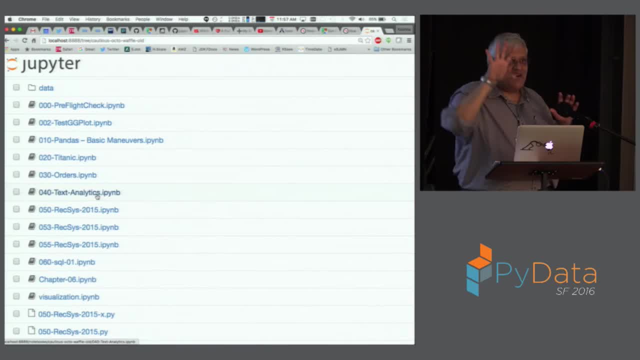 The, the, by looking at the words, you can look at and say, oh yeah. or Barack Obama, what were his major, these things, what were the differences? we could do all kind of interesting things. I have that thing in there but I I don't think we'll get time, so I I skip that one. 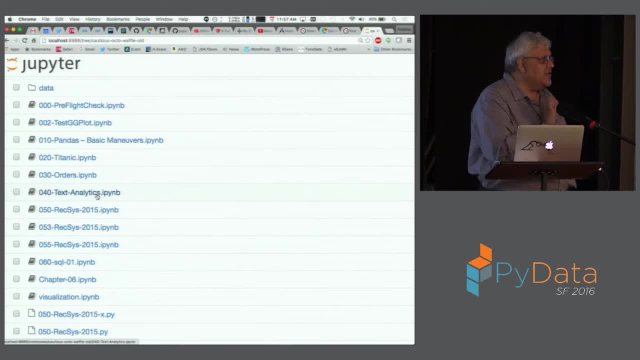 By the way, I also have, But make sure that this data only you look at it. this is like an R data. this is the, the Republican and the Democrat. I'm just kidding. it's the debate debate data right. 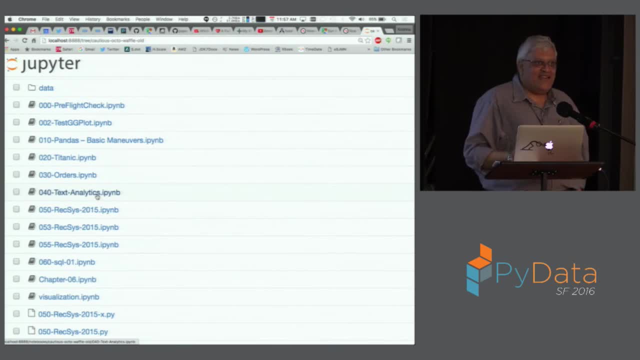 So I have that data as well. Now you can look at the debate data, right, And then say what were the things that that Trump and his gang were talking about and what were the things, Mrs, you know, Mrs Clinton and Bernie Sanders were talking about, right? 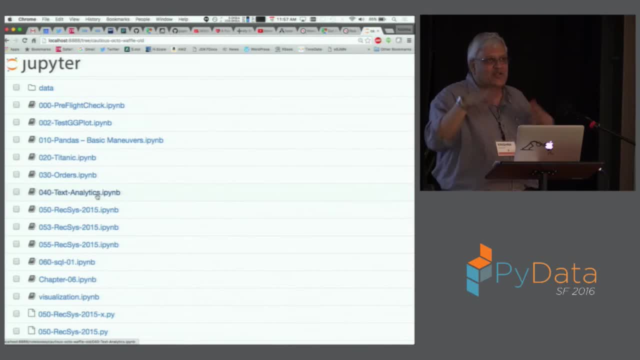 It's an interesting thing. so I have all those things and I was going to go through and use Pandas to take it. But there are a lot of interesting things like split and you have to take common words out, and you have to take commas out, and you have to take quotes out and you have to. all kind of stuff is there. 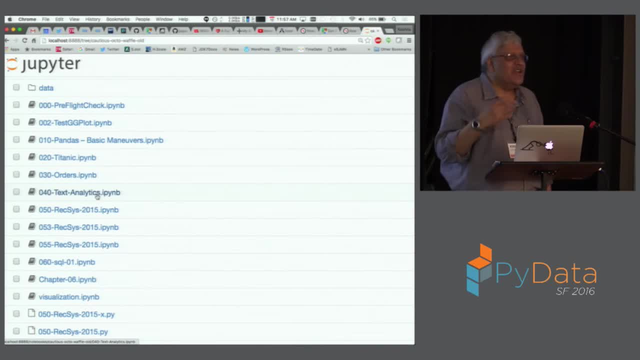 But I didn't get time. so you know I I'm going to leave it up to you to, but I have those things in there. so it's an interesting. it's an interesting exercise in a very different way, right. 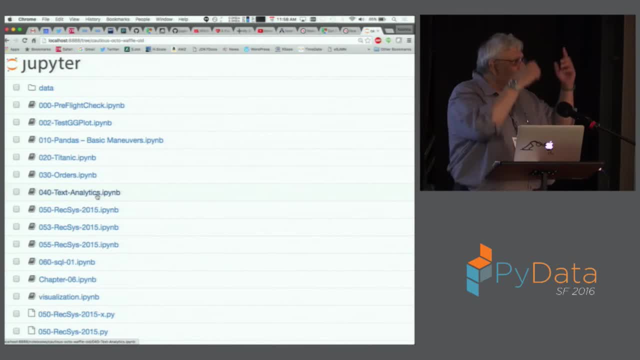 We don't deal with numbers, you're dealing with words. you're dealing with, you know, quotes, words with comma, words with hypons. so so now, that is a very different way of looking at it, that you have to do things with that one. 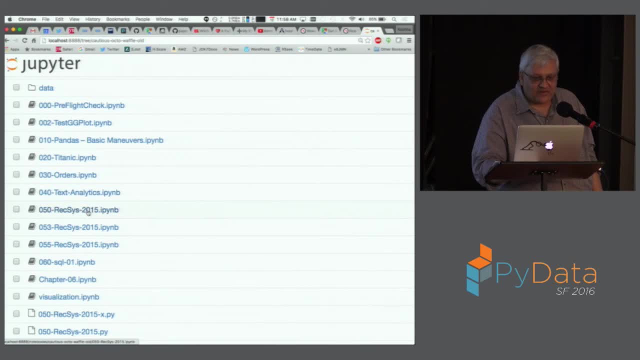 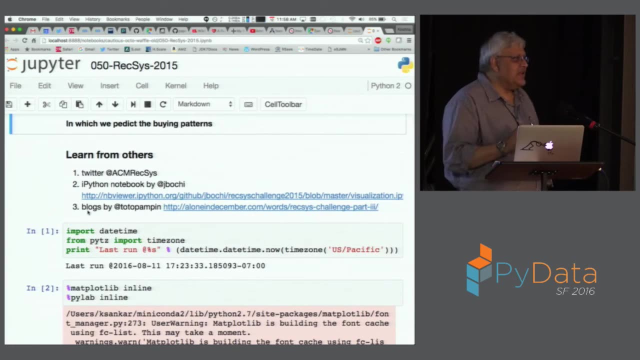 Anyway, I'm going to pass that one and go into this Ruxus guy. I don't have this data in there because the data is like about two gigabyte so I can't put it in GitHub. So what I have done is, if you look at each data subdirectory, I have a readme text in each of the data subdirectory where I put the lineage of the data, where I got the data from or where you can get the data from the source, and that kind of stuff. 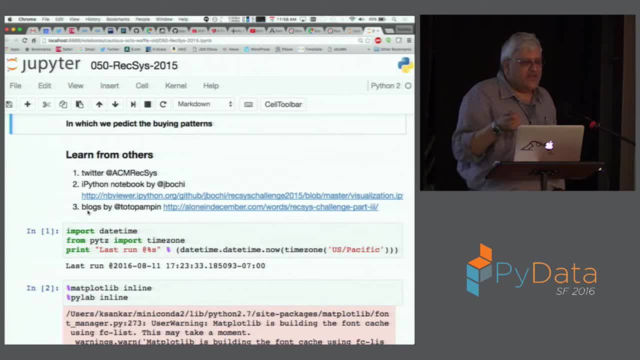 So I'm going to pass that one and go into this Ruxus guy. So if you want to do this one, you can go to the Ruxus 2015 challenge. I have also put the URL in. go to the URL. download the data. put it in Ruxus 2015 subdirectory, you know. unzip it and then you can run this program. 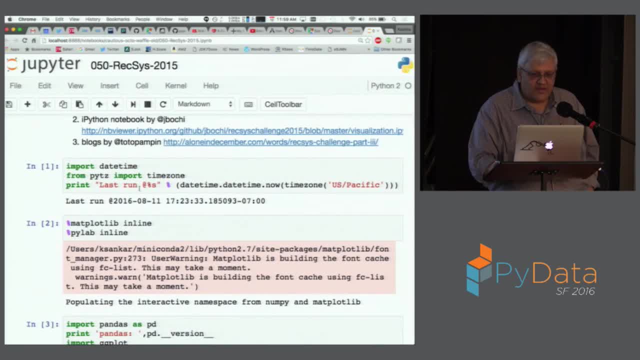 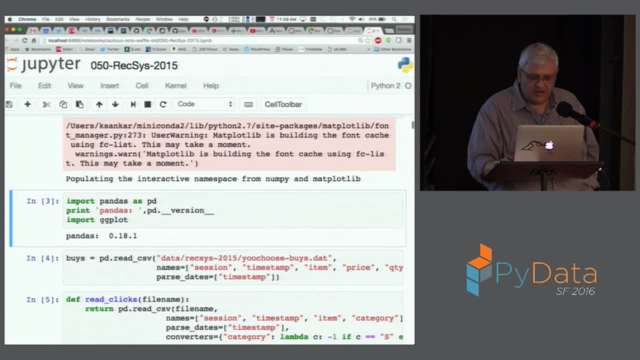 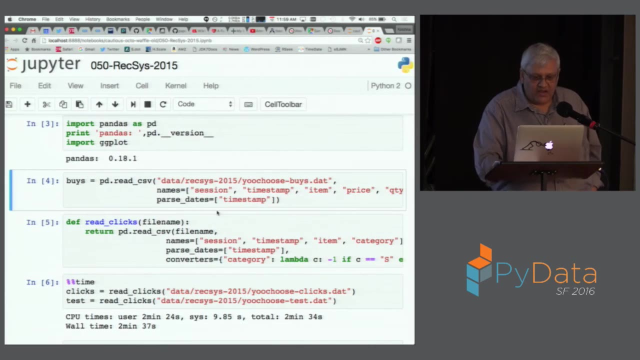 This thing. I'm not going to run it. I'll show you why. So this is. you know, I can run this guy, I can run this one, I can run this one. So there are two files. So what these files are. this file will take about two minutes to read it, right. 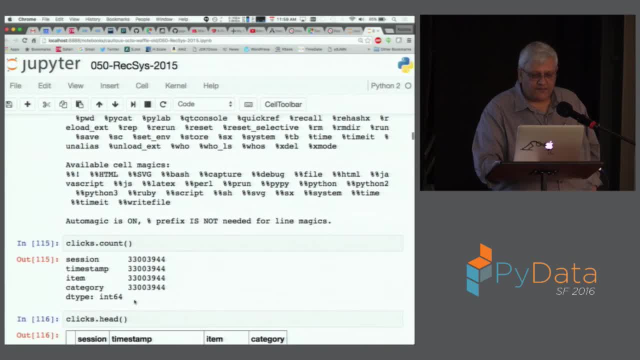 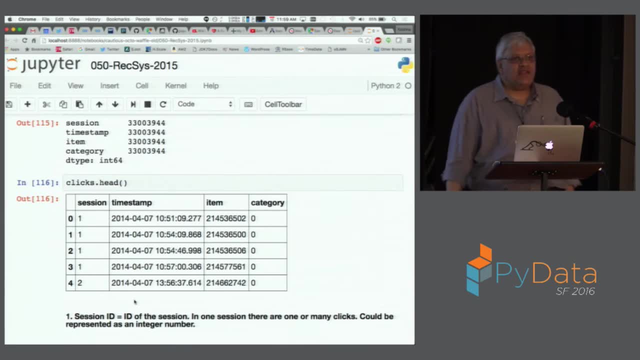 What are these files? So these files are. so this is e-commerce, right? So these are in some sense. these are clicks and buys, right? That looks like a you know, I don't know. it looks like a song group, or maybe it's a good listing for an e-commerce thing. 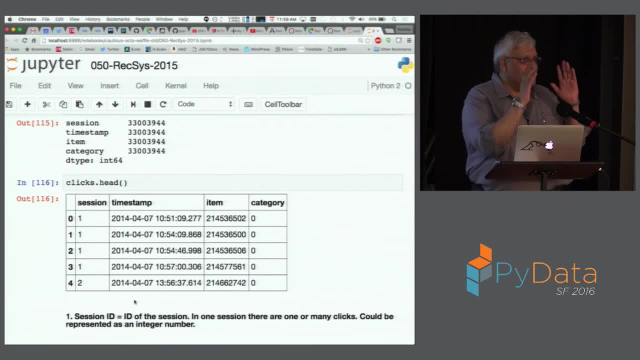 Right Clicks and buys Anyway. So it has session ID, time stamp, item and category. So these are the things that people click, right? You go into this thing, you click on a particular item. it has a time stamp. it also has a session, right. 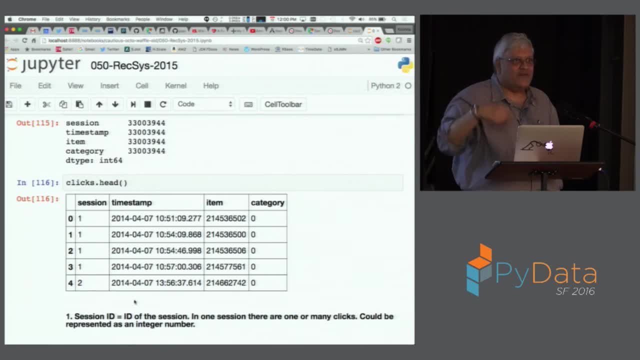 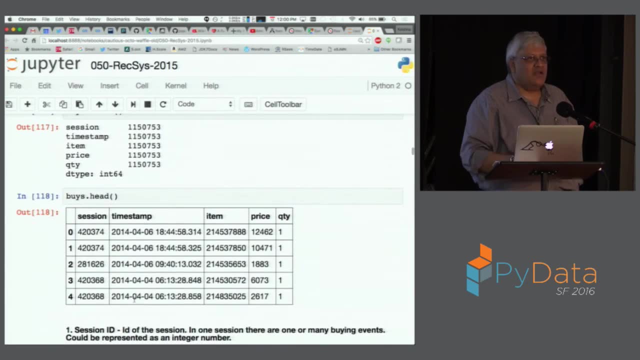 So you go in for a particular, you know time, click, click, click, click, click. you do a few other things And it also has the buys right. It has the same session ID, The time stamp. 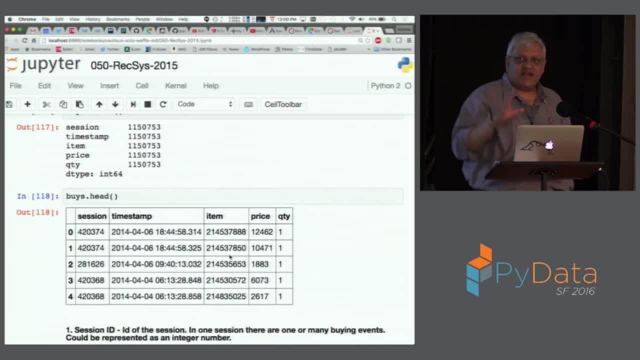 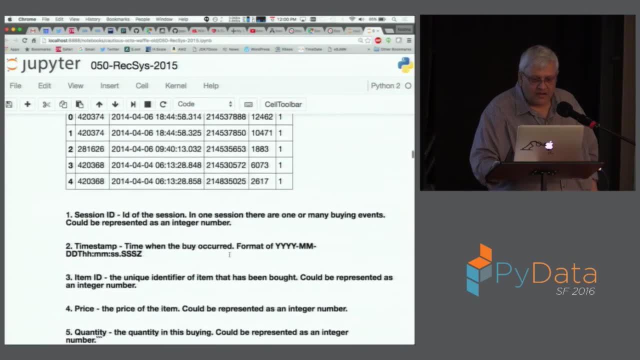 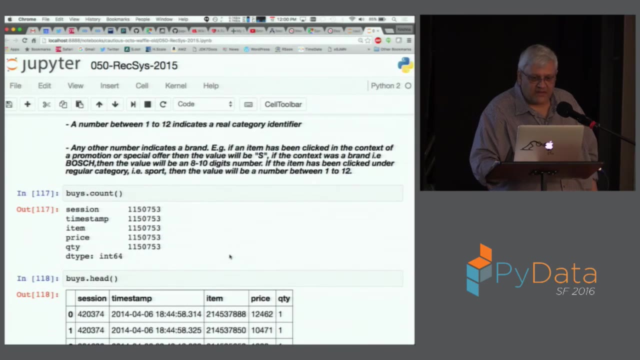 And the item buy Right. Naturally, the clicks will be huge, right It is. if you look at the clicks, there are 33 million clicks or something like that. right, About 1 million buys records, right. 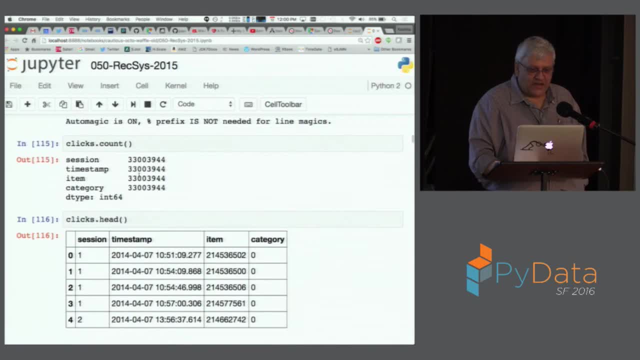 It is 1 million and the clicks are about 33 million clicks, Right. So that is why this data is like about 1.5, I mean actually 1.2 gigabytes total approximately 1.95 gigabytes or something like that, right. 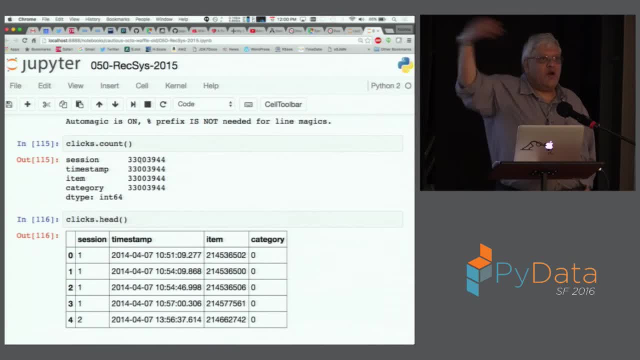 So you have like 33 million clicks and out of them, 1 million buys. You have the session IDs and that kind of stuff. So our mission, if we choose to do so, is to predict right. 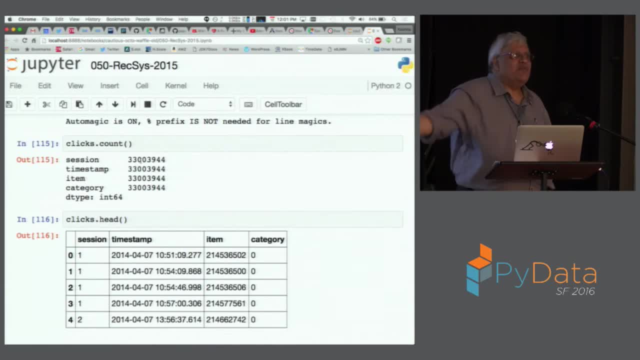 They will give you a set of clicks and say: predict what people will buy, Right. So now the question is: how would you, how would you know? What would you do? Look at it Right. So thank you. 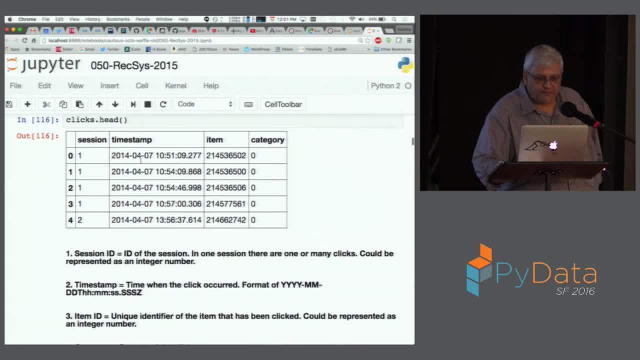 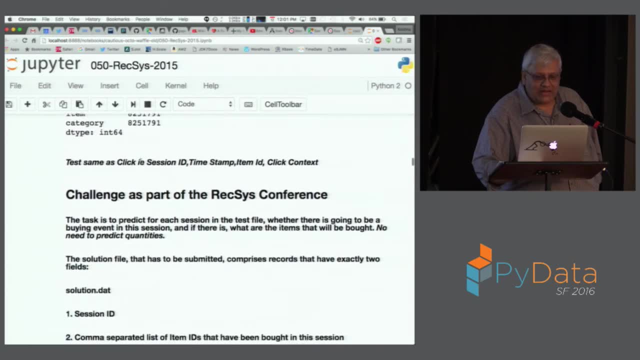 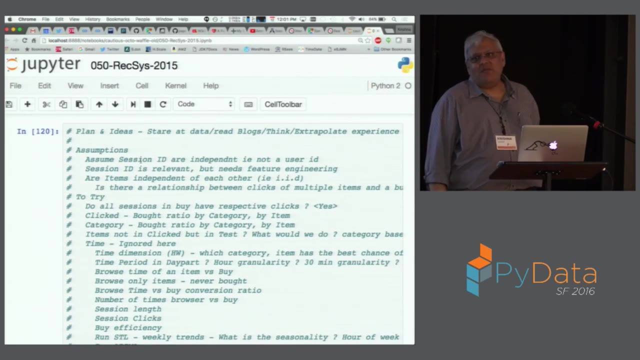 So you look at it. So you have the head, you have the. so you look at the count and the head Right. So then you have all kinds of things that you can do, Right? You look at it and say maybe some items people buy more frequently. 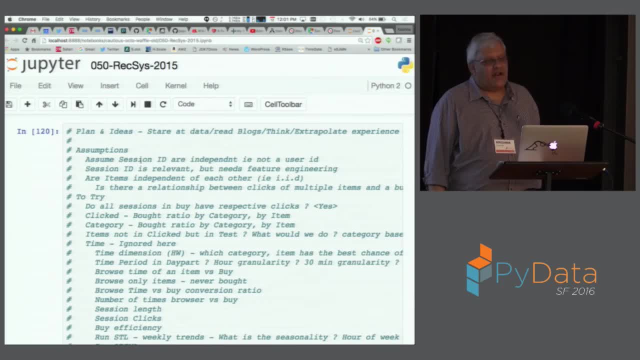 Maybe some items people buy on Friday, Right, Maybe some items people buy without looking, Right, Because these are utility items. Right, You're not going to look at multiple things. You look at it and say: you look at it, I want this, click it, buy it. 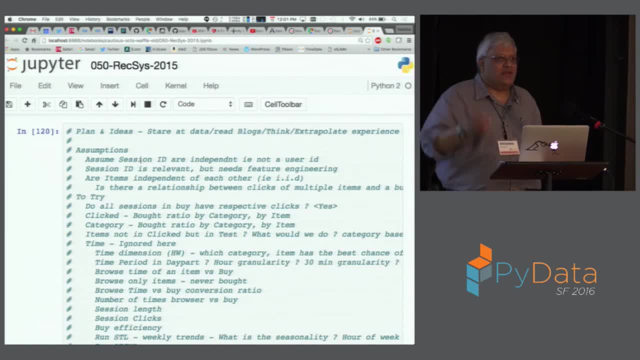 There are other things. you spend a lot of time. Maybe you do the repeat this thing, et cetera, et cetera. So there are all kinds of things that we can do And we have these 33 million records here and we have this 1 million record here. 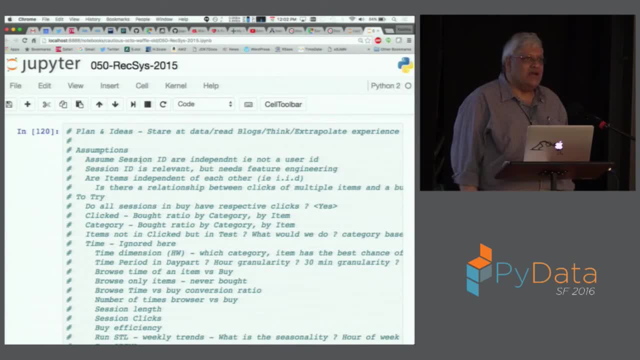 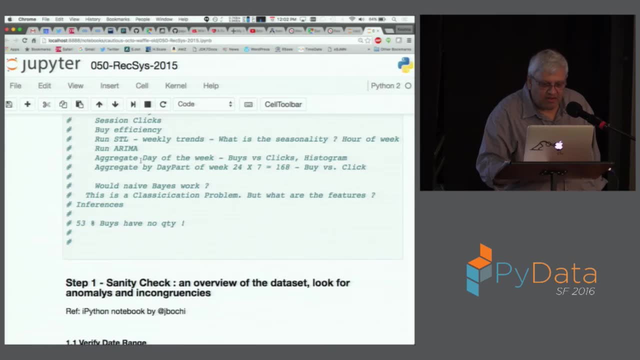 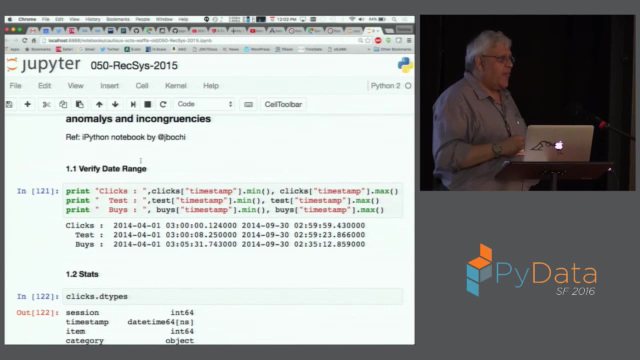 So now let us use Pandas to look through this data, and I think we have, you know, 15 minutes to look at it, And, of course, after that, this thing will self-destruct, Right? So the first thing, there are two, three pieces. 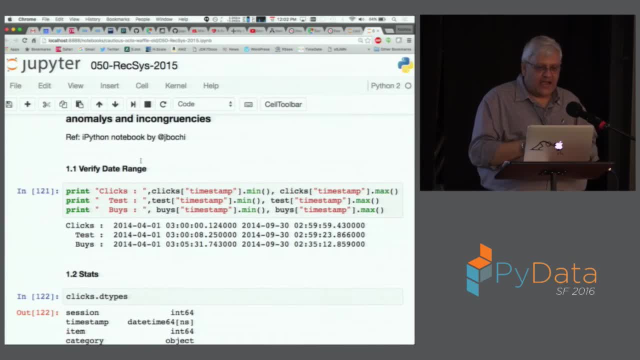 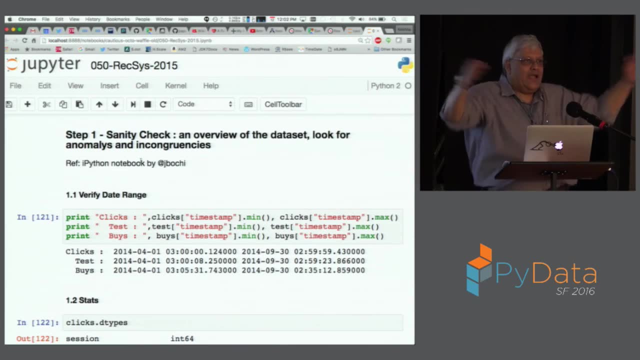 First thing, when you get the data, you look at the data and make sure right anomalies and incongruencies and that kind of stuff. Right Things out of whack. This thing is not there, That thing is not there. 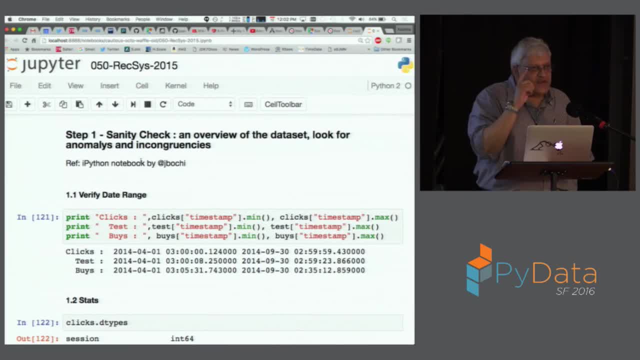 Because you do want to make sure that the data is clean in some sense Once you have that one. the second thing is you look at the data. You look at the data and say how many items, What did people buy, How many sessions. 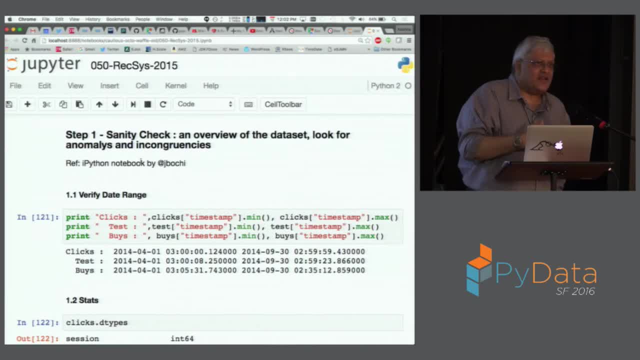 Did every session became a buy, Did everything that bought had a session, had a click, et cetera, et cetera. And the third thing is you extract features. You look at it and say, hm, I think I need day of the week. 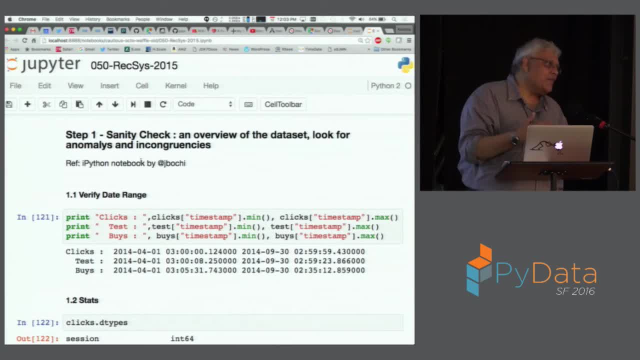 Right, People do things on Monday. Monday probably not many people are going to buy things. Maybe Friday people will buy more things, Right? So if you look at, if you want to predict whether some click will turn into a buy, you 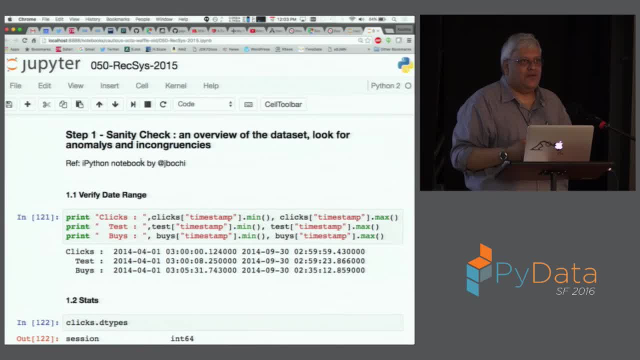 look at it and say, yeah, this is a weekend. I think there is more possibilities, Right? Or you look at the day of the week- Sorry, You know. you look at the date. You look at the month. Maybe some items people buy during Christmas. 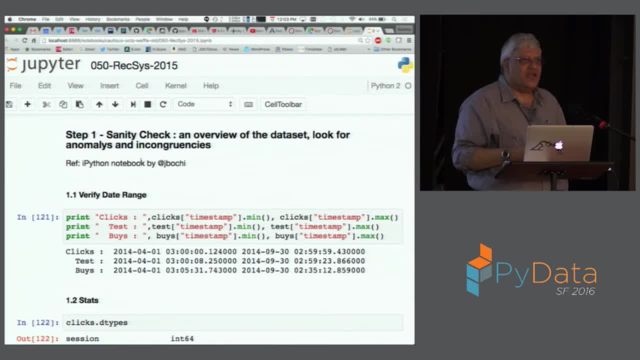 Some items people buy during this one. So if you know all those things, you will be able to do things Right. These are some of the transformations, So this is where you extract the features. Let me cover in a part of these things, a little of all these things. 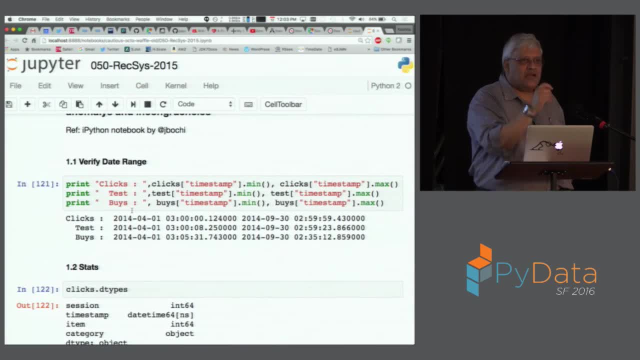 First is verify the date range Right. You have the clicks and the buys. You want to make sure that the date ranges are right. If you have some clicks without any buys or some buys without any clicks, you can't make anything out of them. 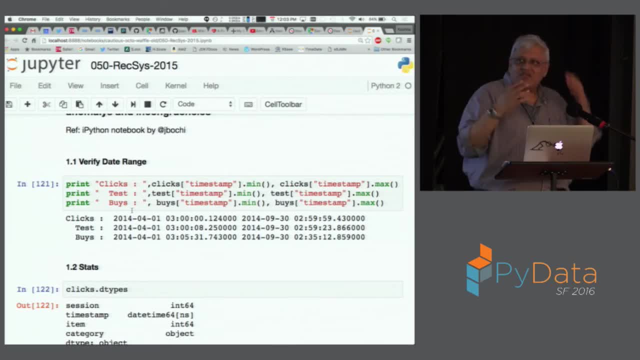 Right. So what you might have to do is you might have to just delete those records. Luckily, we don't. So this is this thing Right. Oh yeah, So we read this one When we the read: CSV, right. 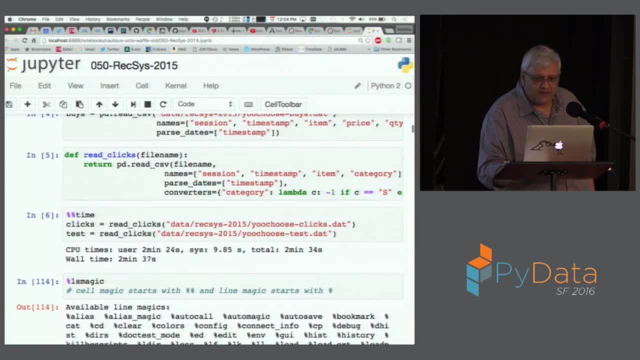 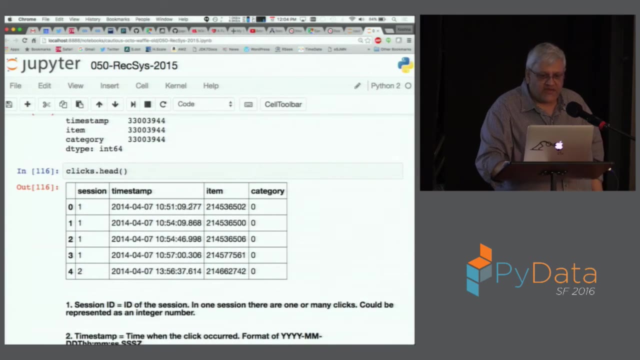 In the read CSV we did one trick: We did parse dates as timestamp, So we didn't have to do anything. The read CSV itself parsed it and it gave you the this guy- as a timestamp. In fact, this is where you know we have the. so if you look at the D types, you will. 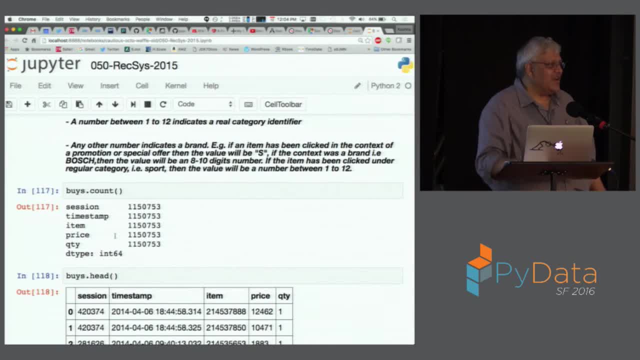 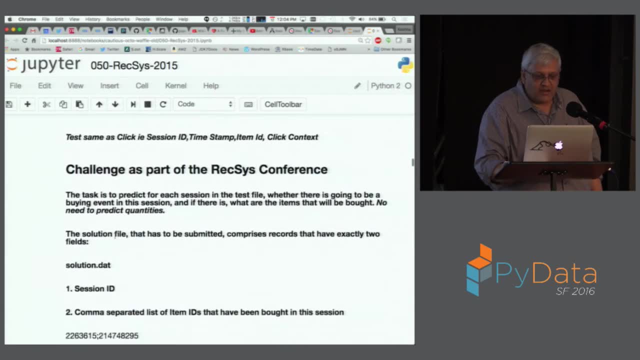 see that it is a timestamp. So that's a good thing, because we already have the, because this time is important, right, That is already a timestamp, So we are in good shape there. So what we do is we look at the timestamps and say: give me the min and max. 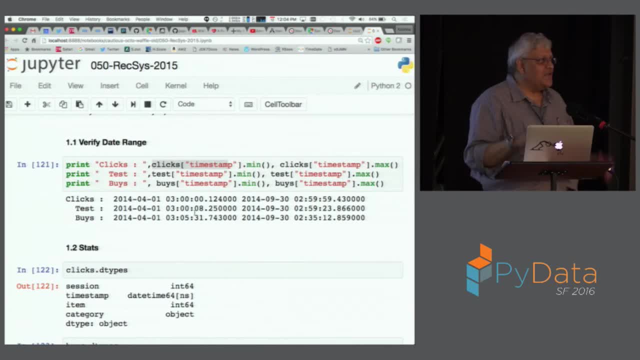 Right. Give me the min and max of the clicks and the tests and the buys and make sure that they are within this thing And they are Right. The clicks are between probably 3 am and 2 am on two days. 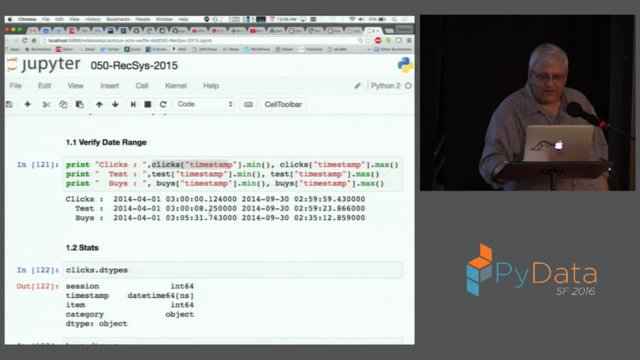 April 1st to 9 am. April 1st to 9 am. And these are all within the. so we are in good shape, Right? We don't have to do anything on the date side, So let us do some stats. 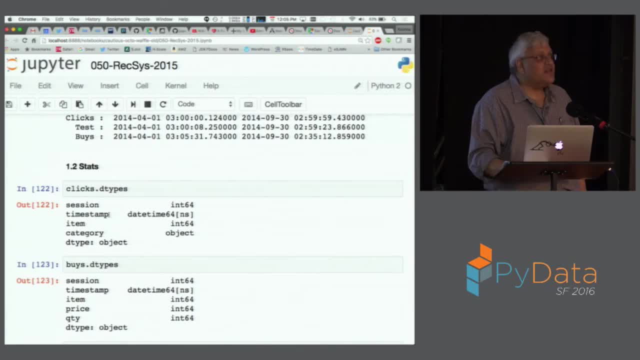 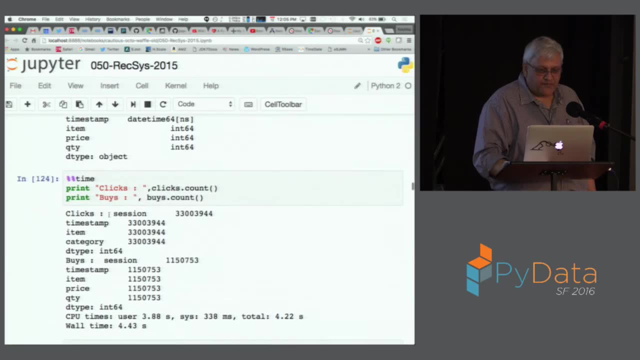 Right, The D types. This is where we know session is an integer, The timestamp is a timestamp. We know that it's a timestamp, We are in good shape. So now we do the count. Right Now we know how many. you know how many records are there. 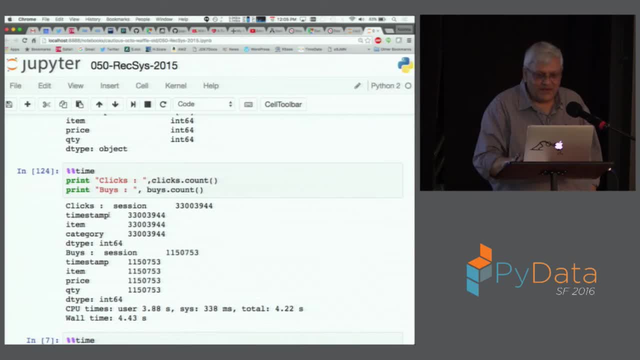 That's the next thing to do. And look at that and say how many records are in these things? We know the count, We know how many records are there. That is good. So first question: You look at it and say ha. 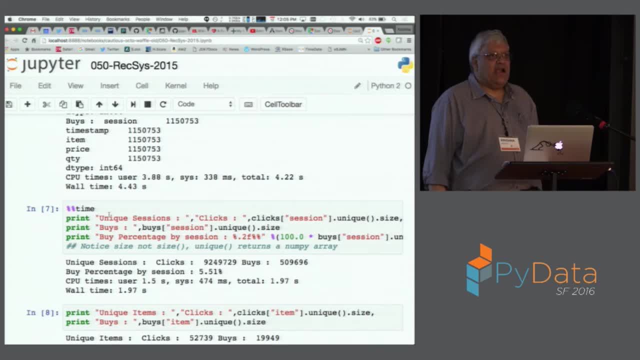 What is the first thing they have given? They have given us the session ID, Right, So let us look at it and say: how many sessions? What is up with these sessions? Are all these good sessions, All these bad sessions? First is unique sessions. 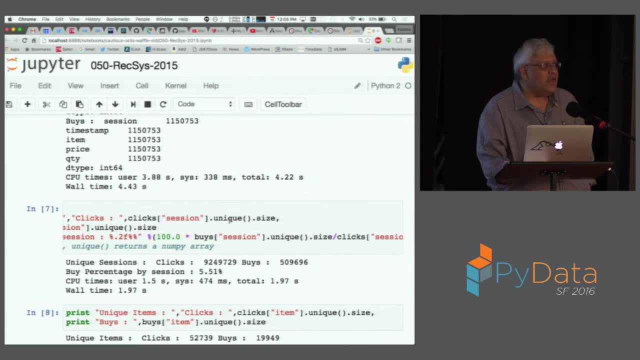 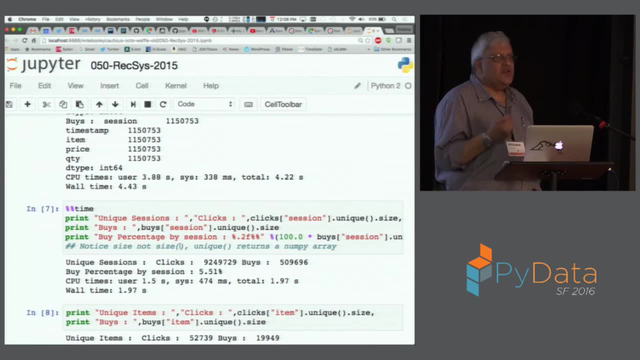 Right. So what do you do? Click dot session And you do the unique and size. So you know number of unique sessions. You know the number of unique sessions that resulted in clicks Unique sessions that resulted in clicks Right, And then you do a percentage. 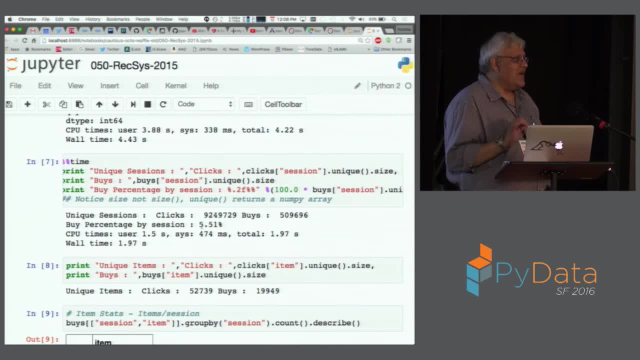 So you have an idea. Oh yeah, 5% of the sessions have, you know, become buys Right, Unique sessions. So that is good, Because that means people click a lot of stuff, then do a thing Right. 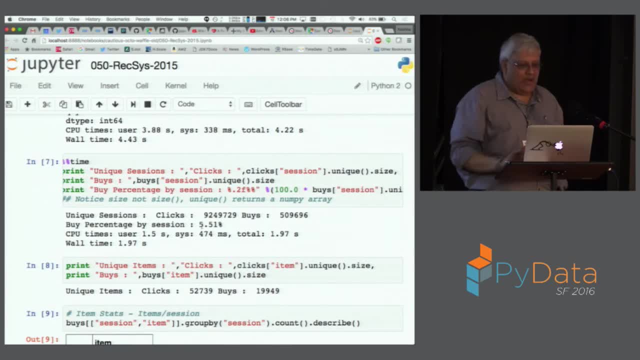 5% of the time the clicks turn into a buy. So that's a good thing, Right? So you see that how we can do unique, we can do size, and that is how we get that particular thing out. Next one, same with the buys. 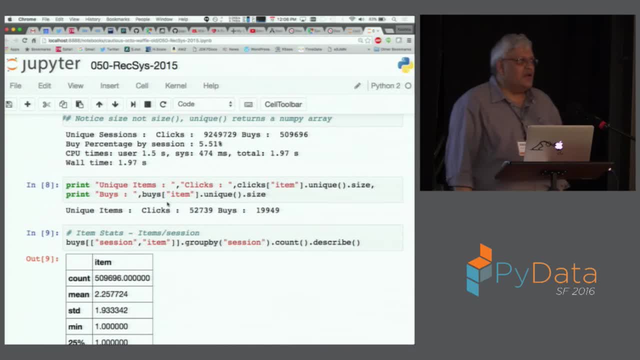 Right, Yeah, Unique items. Now you look at it and say, huh, did all items? end up people buying all items? They didn't Right. If you see people clicked on, say again: click item unique Right. 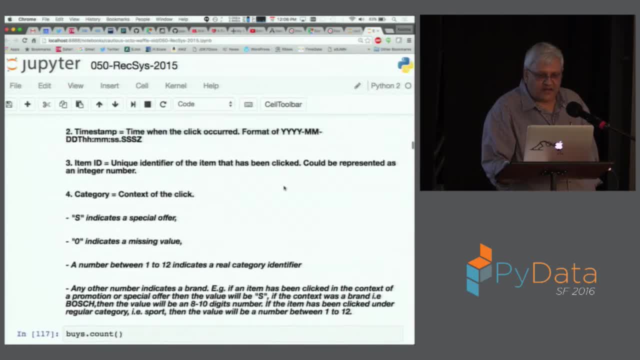 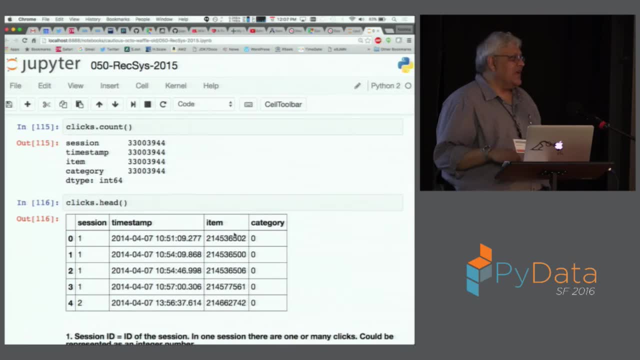 Because we have this. when we go back here, the things that we have are session time stamp item, Right, So we're not doing anything with the category, but that's a whole set of things that we have to do on the category. 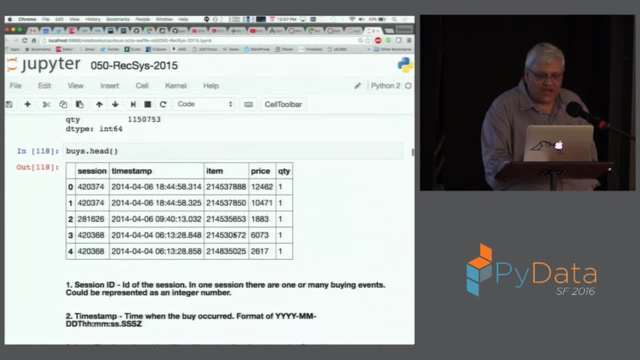 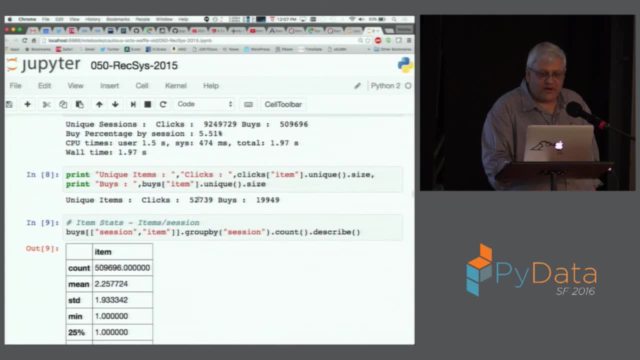 So we can do similar things on the category. So we go in and say, okay item, Give me the items That's interesting. So people clicked on like 52,000 items but they bought only 19,000 items. 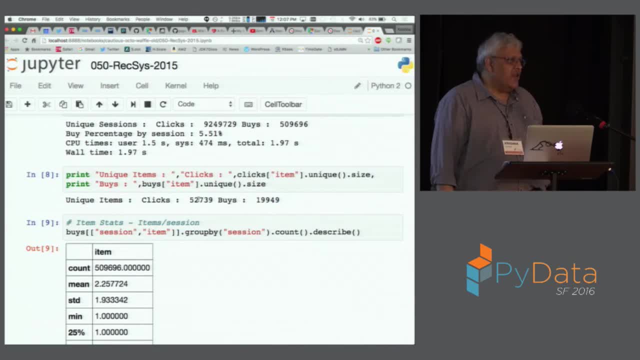 So keep in mind, Right? So this is what I was talking about. So now we are not going to say the you know whatever, 52 minus 20, 32.. Right, About 32,000 items. We are not going to say people are not going to buy them. 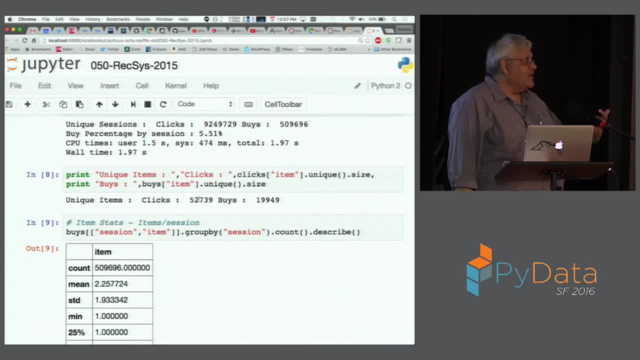 Right, Remember, this is a slice of the data, This is a sample of the data, Right, But people would buy other things, maybe other times. So we cannot just predict and say no, they're not going to buy those things. 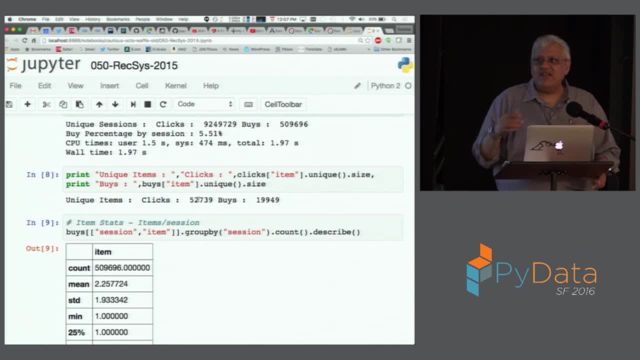 So that is where it gets more interesting, Right, But be careful that you won't look at it and say, oh yeah, because people didn't buy on the test data, people didn't buy on the data that we have. we are going to follow that. 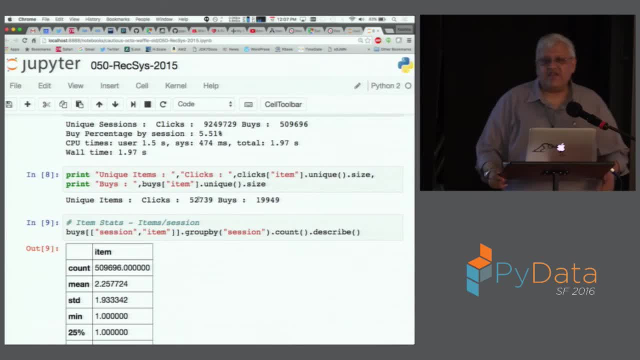 one. You can't do that Right. This is where I was talking about saying that you know the you know. this is a you know. there are things we know and there are things we don't know, And we need to know each. 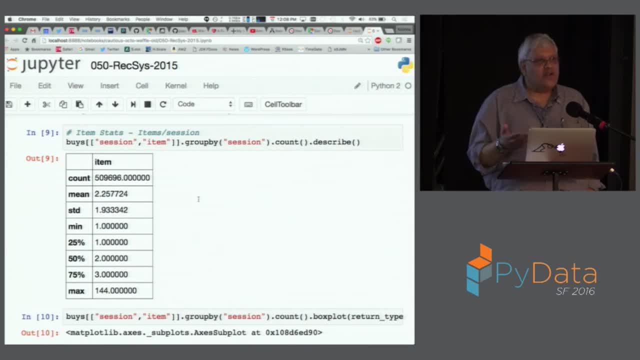 Right, So the describe, So describe gives you count the standard deviation, et cetera, et cetera. Right, You can look at it and say: yeah, mean, if you look at the item the maximum, some people 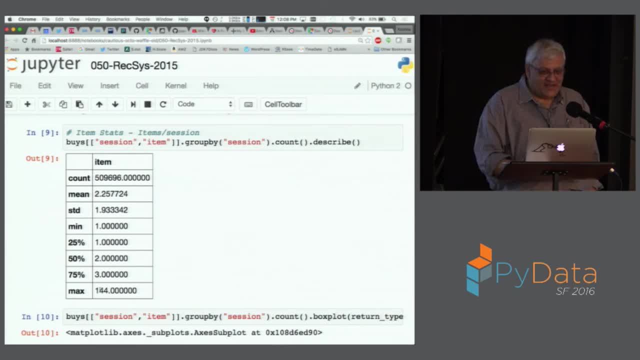 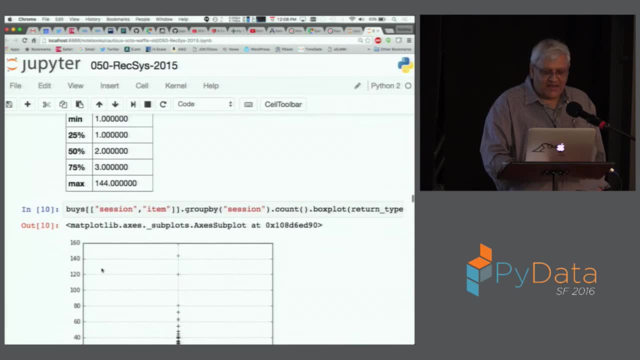 have bought like 144 items in their shopping cart. whatever it is. Minimum, of course, is one, One or two or three Right. So three is a major one, Right? If you look at it Now, you can go back and say: give me a plot. 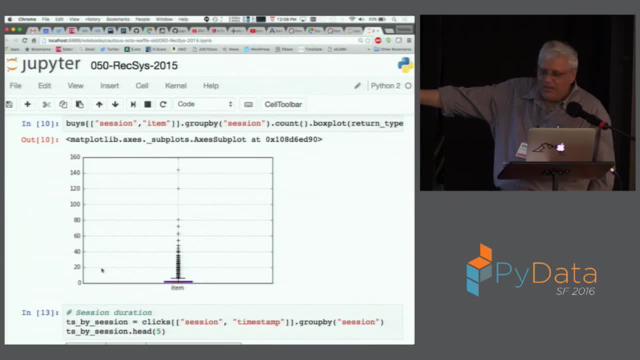 So you have a plot and you can look at it and say, oh yeah, between the mean is probably two or something like that, one or two, And then about 40, 50. And then there are these outliers sitting in. 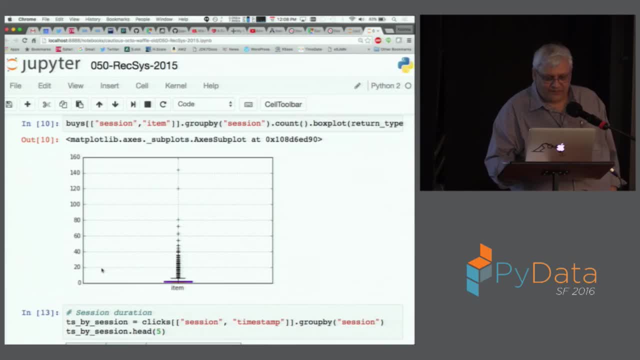 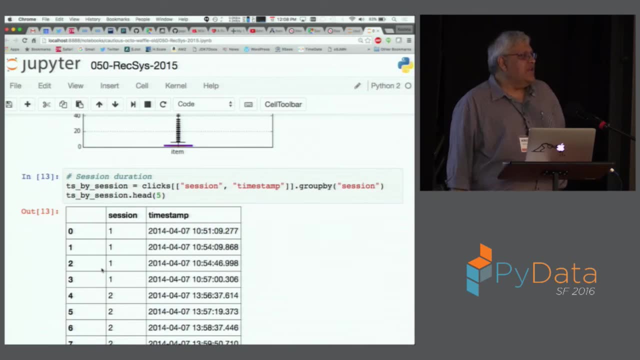 Right, So you are able to get that one. So, oh yeah, Another interesting thing: Right, You want to get the duration Right. So the important thing is, if people spend more time on clicks, do they buy or they don't? 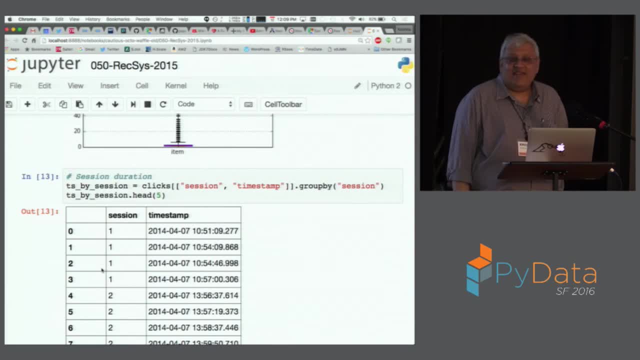 Right, You can look at it both ways. Maybe people are bored and they are just clicking, So if they spend more time, maybe they won't buy anything. Right, If people want to buy something, they will go in, click on it, buy and walk out. 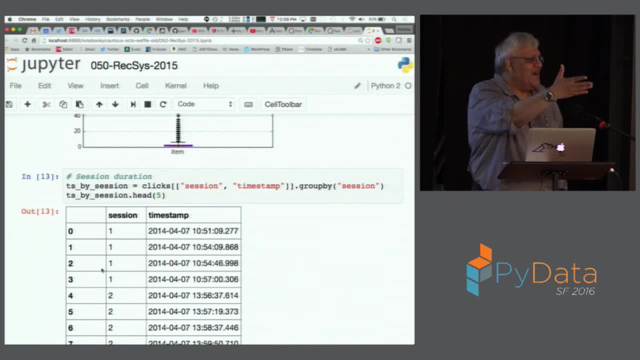 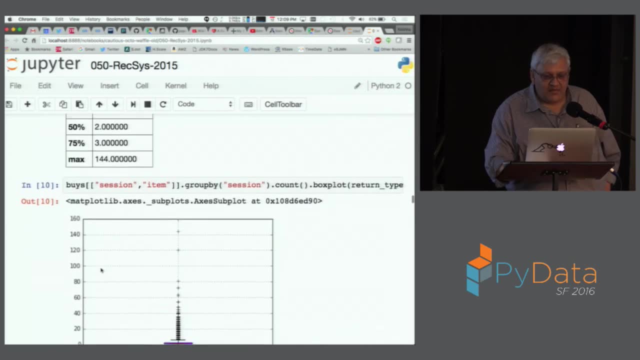 So you can look at it and see if the sessions are shorter. most probably you'll end up buying Right, Because shorter sessions. what else do you do, Anyway? So now let me ask you a question: How would you get the duration of a session? 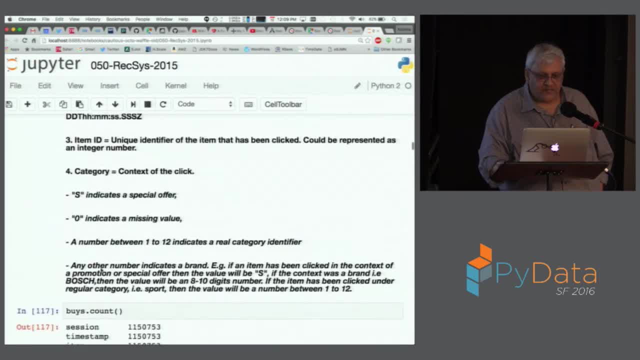 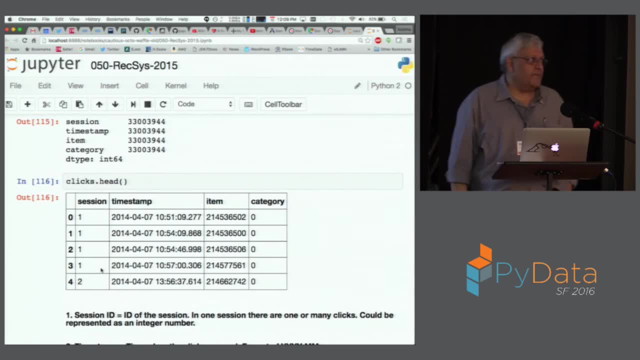 Right, This is what we have, Right, How would we get the duration of a session? So this is a very interesting this thing, Right? So what do we do? Yes, Yes, 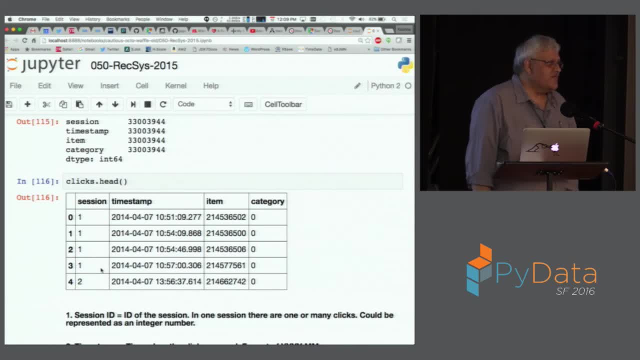 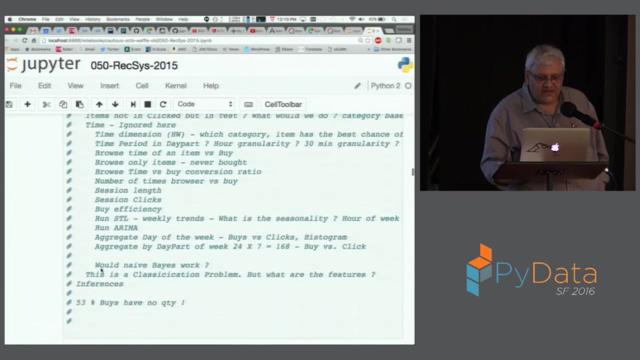 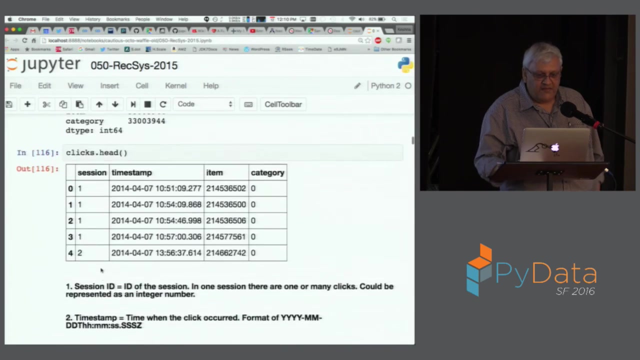 So group by. What we do is first remember. it's not easy If you look at it, even if 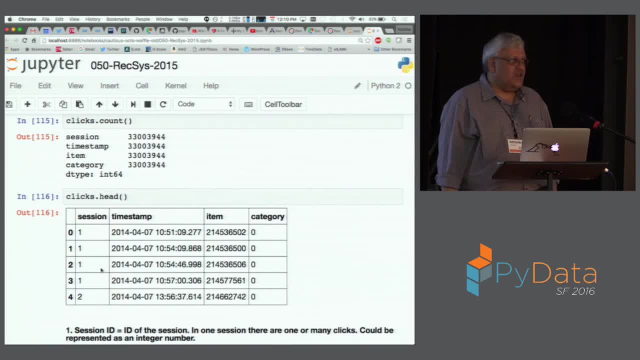 we want to do it. it's not that straight forward, Even if you have to do it. what you have to do is you have to go through each session and then go through the time stamp. give me the minimum time stamp. give me the maximum. 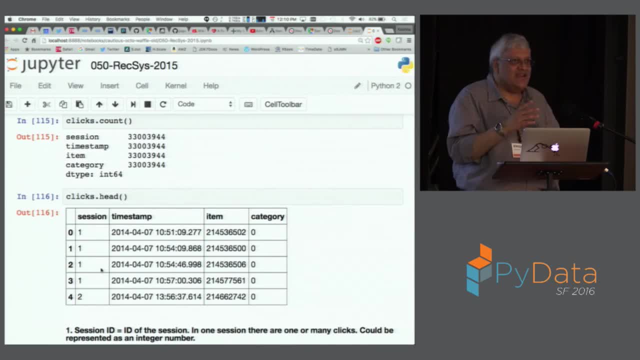 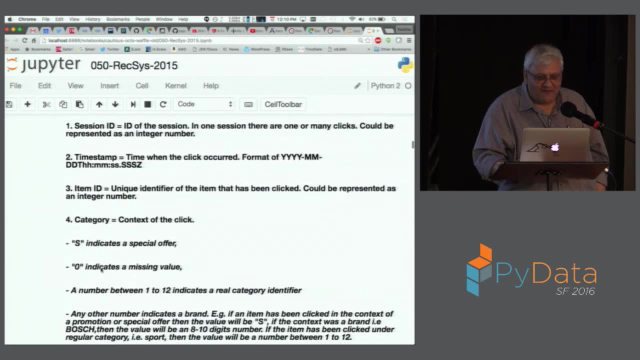 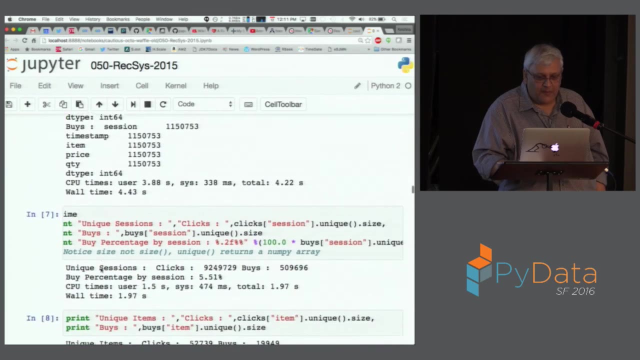 time stamp. It's a lot of work in there, Little generations here and there, to get that one. Pandas does it very well. Pandas does it very cleanly. So what do you do? First thing you do: it is not even in. 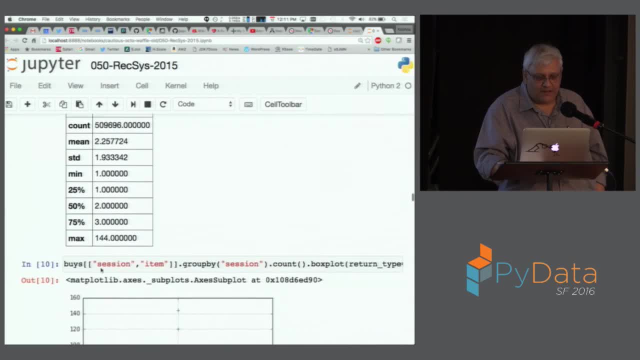 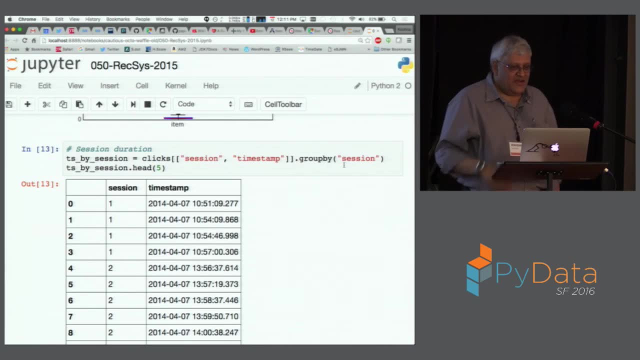 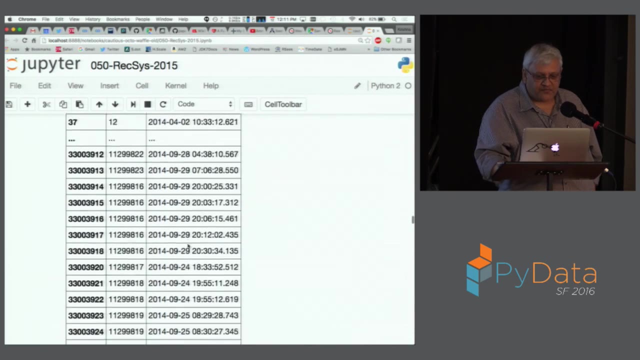 Pandas, it is easy, but it's not. you just have to. first thing you do is you group by session. So you group by session, you have these sessions in there. Then remember, when you do group by session, what it does. 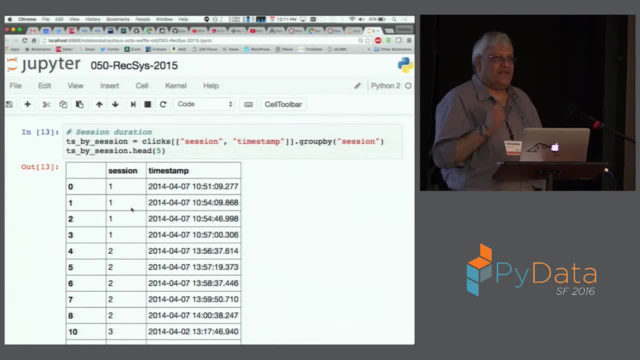 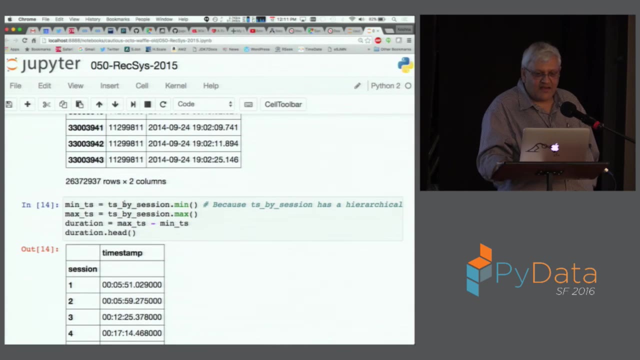 is. it turns this session into an index. If the session is a column, we can't do much with it, But if it is an index we can do things with it. So you turn that into an index and you just do a min. 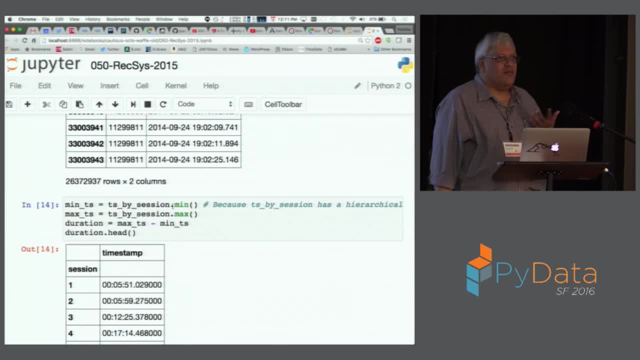 Let me ask you this: if you do a min on a column, what would it give you? The minimum of the column? it will give you one number. It will say this whole column minimum is two. But because this is a multi-indexed- remember this is where the 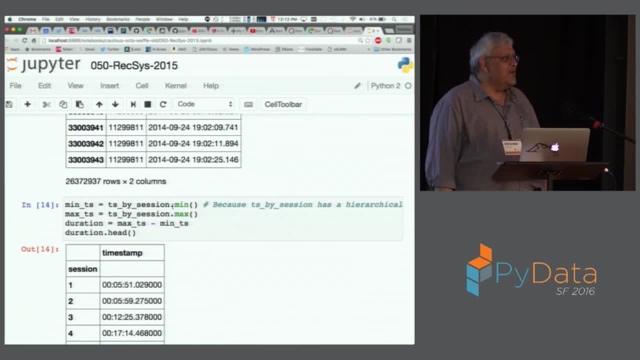 label the multi-indexed column. what does it give you? when you call about minimum, It gives you minimum for each unique index. So it returns a column Session ID and the minimum for that session ID. So that's an interesting one, right. 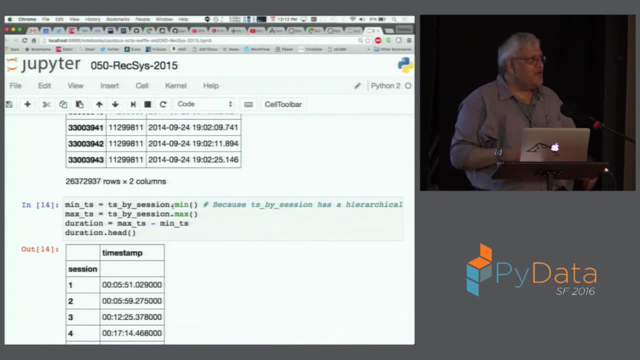 That's exactly what you're talking about. So now what do you do? Indexed column right. First you index it by session. You say: give me max, give me min, So you actually get two things with the session ID in there. 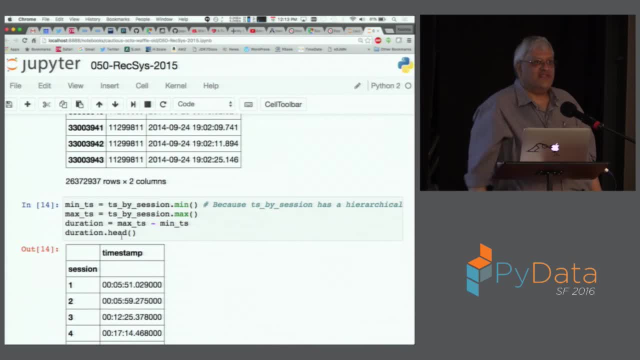 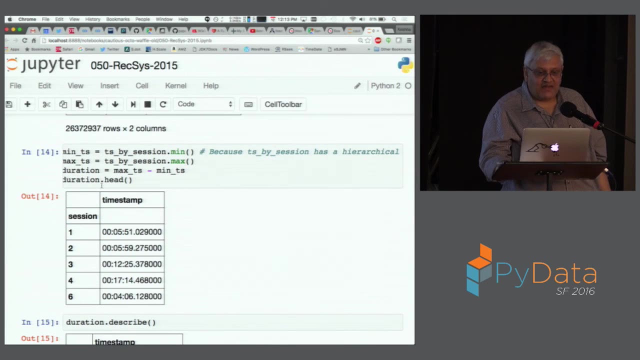 And then you find the difference, you get the duration, Because the max minus min is the duration. So that's an interesting trick to it. So you do a group by you, get this group by thing, and then you do the min and the max, And then, when your duration is min minus max again, 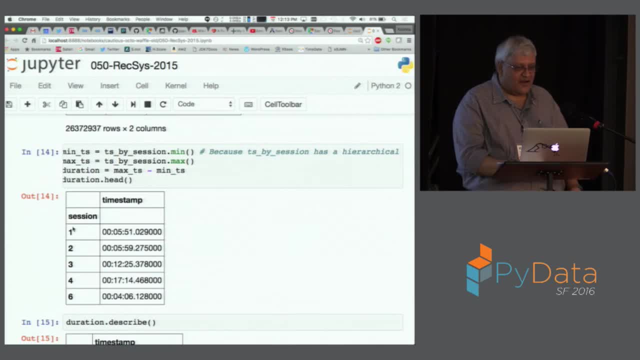 these are all column operations, So in the end you get this nice column with the session and the timestamp which says the duration of that session. So that's a good right. It's a very good nice operation that gives you that very powerful. 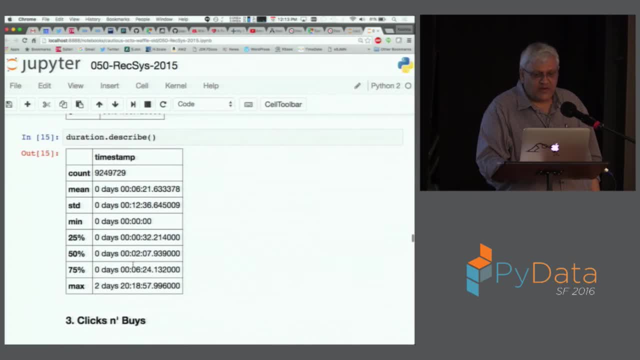 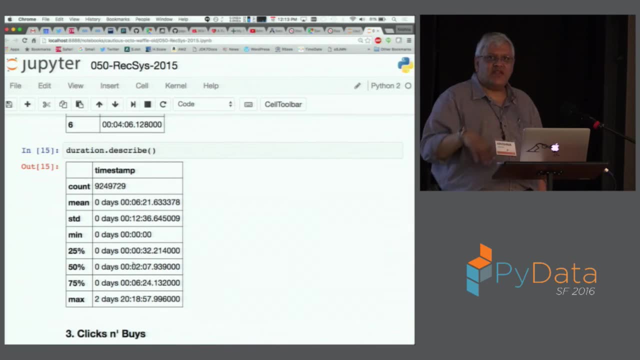 operation. So now you look at the duration dot describe et cetera, et cetera. right Now you can look at it and say: maximum durations, minimum durations. You can actually put this duration into something else. Yep, Two more minutes. So now, how many more minutes do I get? 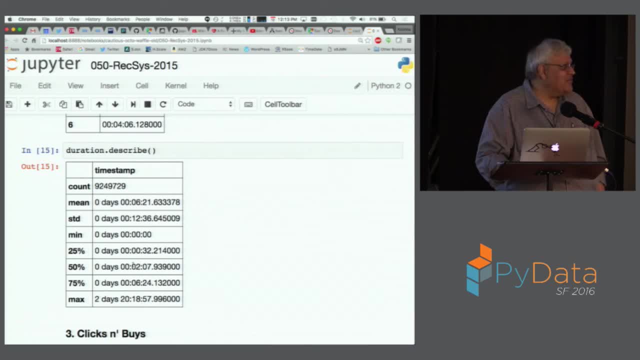 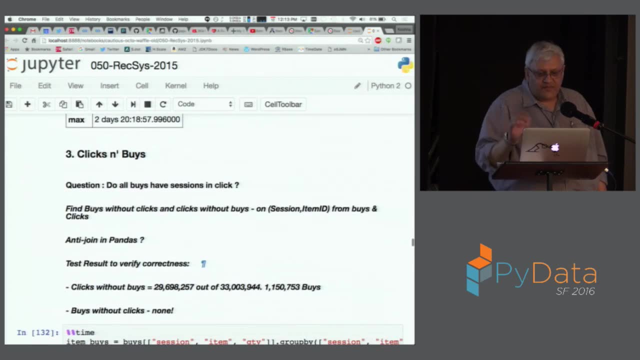 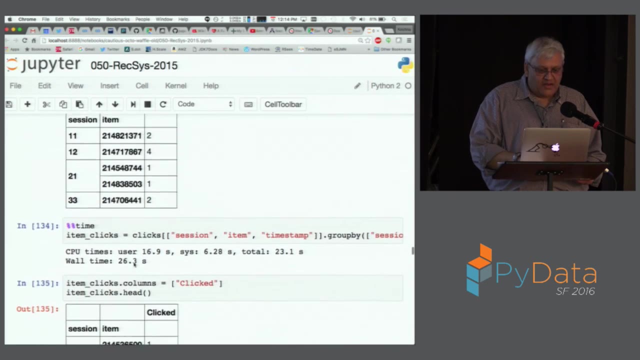 after this is over, Can I get 500 more minutes, or how does it look? So, anyway, I will quickly. there are actually, you know, there are more things in there. The other thing that you do is you want to compare, click, and so I'm going to take five more minutes. 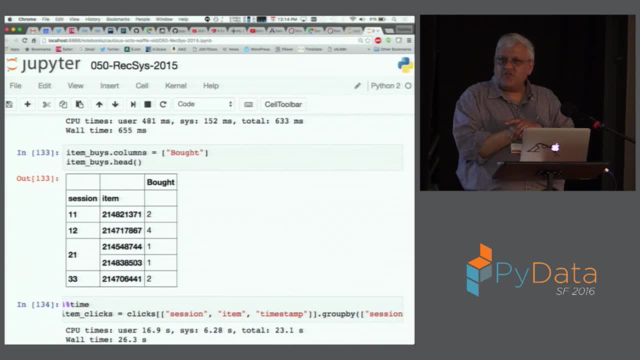 Is that okay? Five, ten maximum, ten more minutes, Is that okay? I don't want to stand between you guys and lunch, but on the other hand, I'm actually more hungrier than you all, probably, So I might run out, Anyway. so now another thing you want. 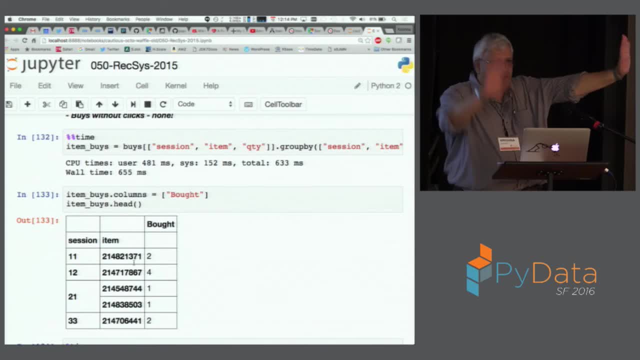 to look at. You want to look at it and say: I want to compare these buys and I want to compare the clicks and buys and look at it and say: how do they line up for each item right? How do you do that one? 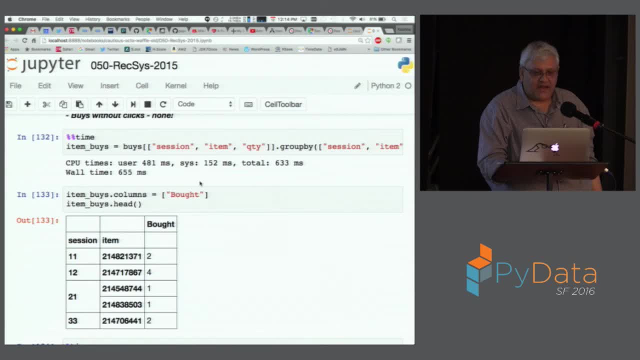 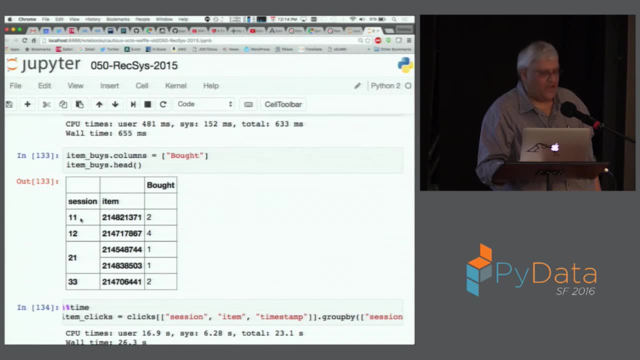 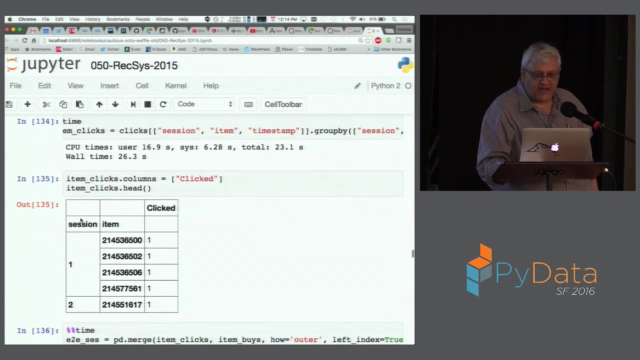 First of all, you group by session item and the quantity, So you get this for each session, for each item. what did they buy? right, And the same way. on the click, you do the same this thing, right. You do the session time and the time stamp. 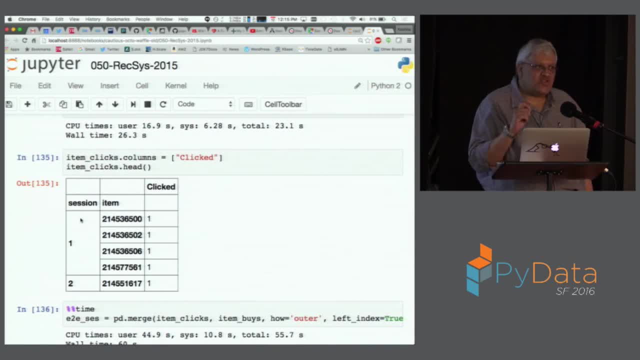 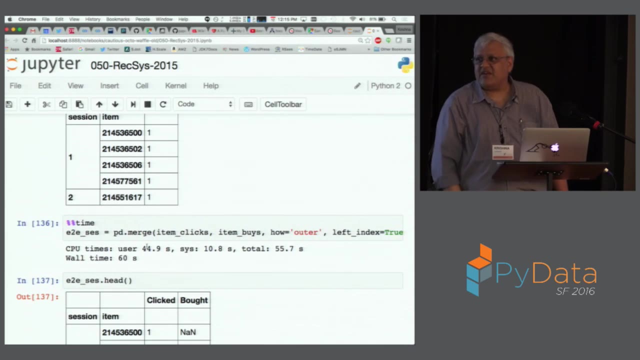 So you know that for each session, for each item, how many clicks they made, right Now what you can do so you have the group by and you do a merge. So this is where earlier you were asking about the indices, right? 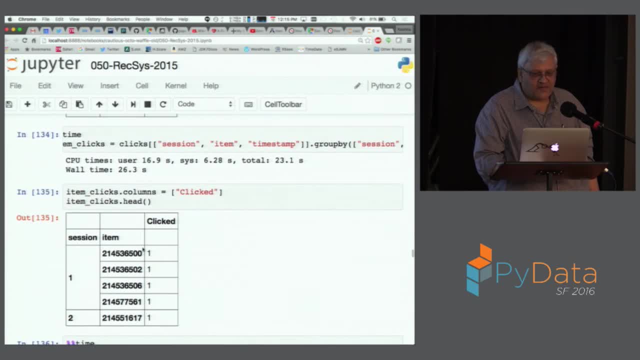 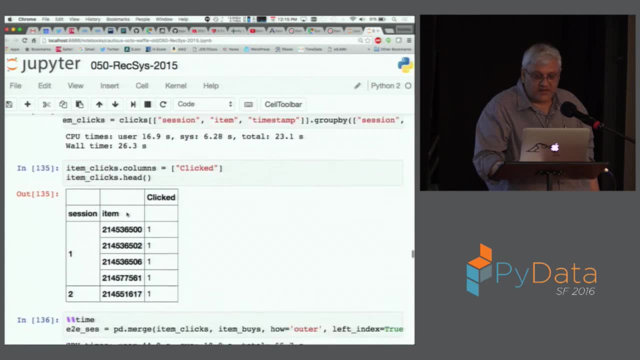 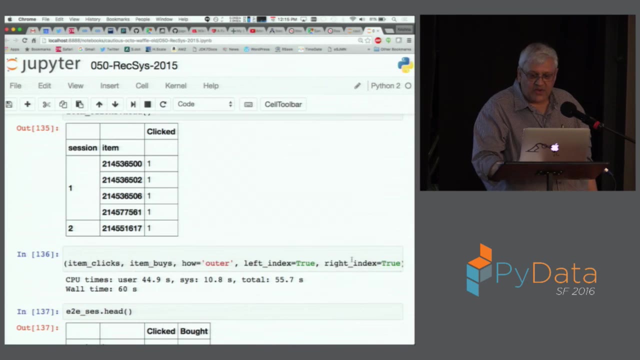 So remember these two columns, these two data frames are. these are indices. So when you do a merge, you can say: merge on these two. how is outer? and left index is true and right index is true. So what you are, 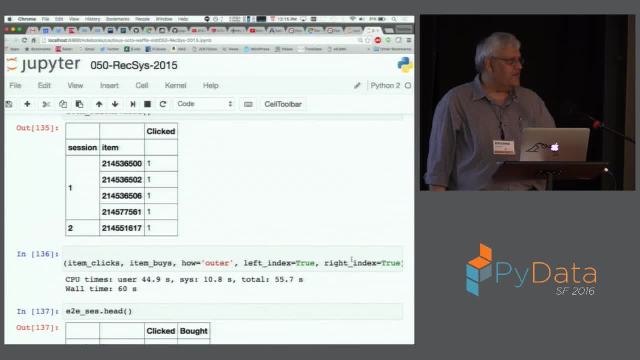 saying is: don't merge on same named columns but merge on the index. Our index is basically the session and item ID, So it merges that one peacefully. It looks at it and says, oh yeah, this thing has this, this thing has this thing. 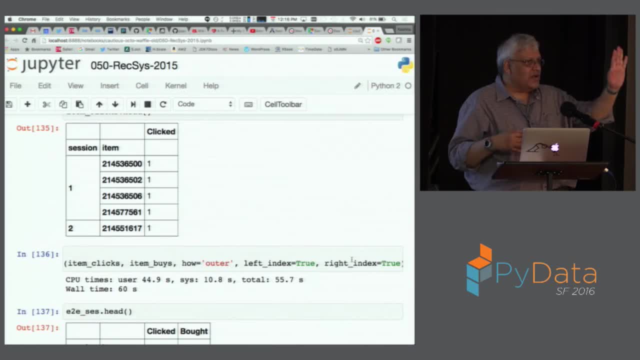 and you have the outer join right. When you do the outer join, you have the clicks and you have the buys right. So it will include all the clicks, it will include all the buys and if you didn't find the corresponding, 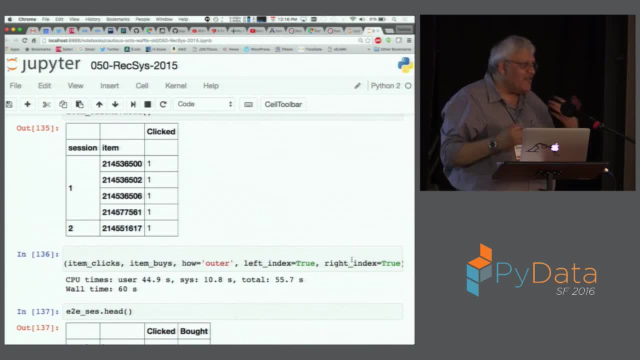 clicks, it will put NAN in there. So this is where we actually want NAN. So then we can look at it and say: are there clicks without buys, are there buys without clicks? that kind of stuff, Anyway. so you do that one. 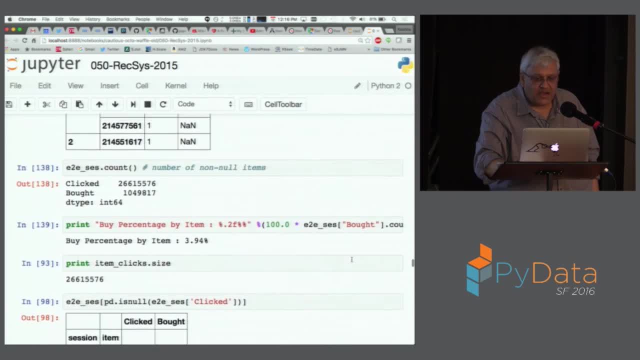 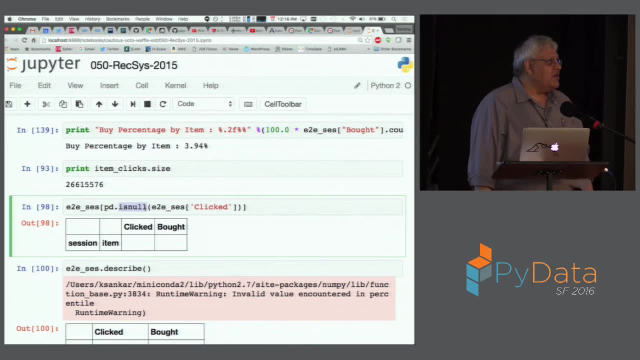 and you know, and then you can do count and so you can look at it. So this is where you are asking a question, right? The is null thing. So I want to find out if there are any buys without clicks. There are none, because we can look at it and say there is none. 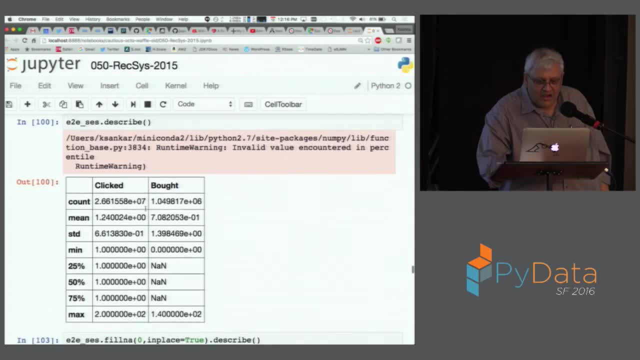 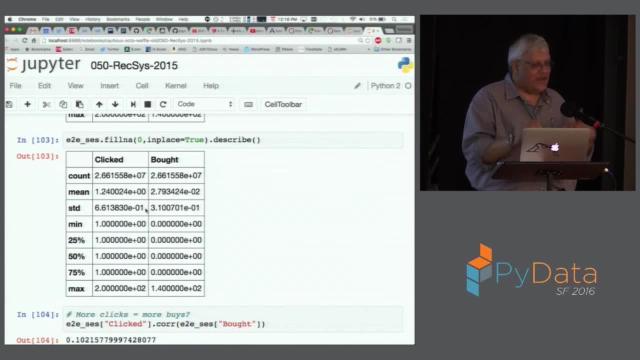 So anyway, so this is where you can use is null to find out There are more maneuvers like this. By now you know right, You have the group buy, you have these things and you manipulate with these things and you get more and more interesting things. 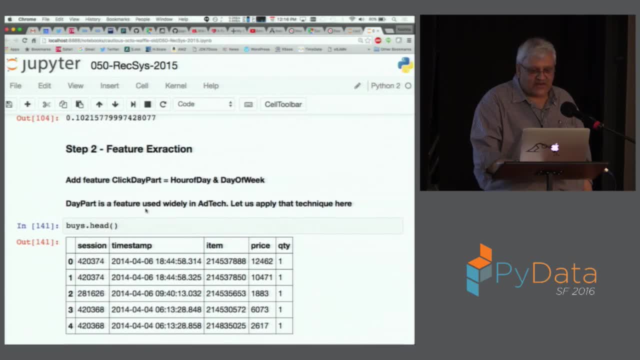 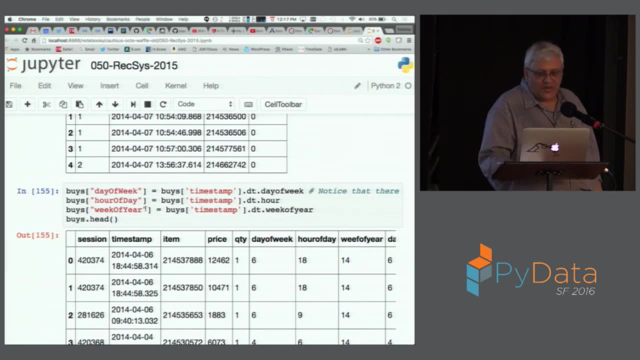 The feature extraction. one of the feature extraction is the. so this is what I was talking about. right, The hour of the day and day of the week. right, So you can do the extraction. Now you know that. right, You create a column, you use the DT to get the day of the week. 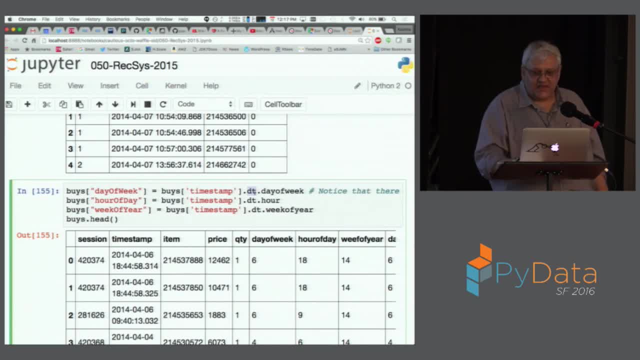 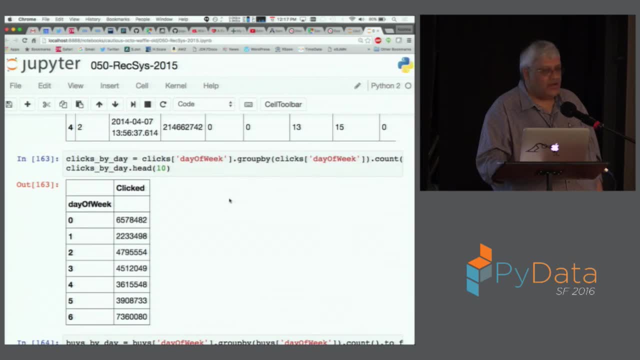 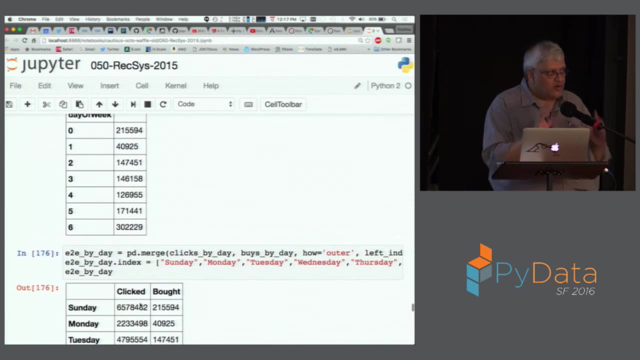 hour of the day, right, Because you already have a timestamp So you can actually get these things in. and once you get those things in, then you do a group buy. When you do a group buy and you change the and you change the. 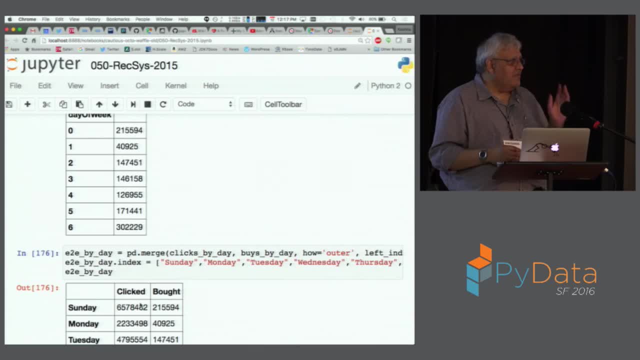 you do a group buy and then you do a our join right. When you do a group buy and join, you will get the number of clicks per day, number of buys per day, right. You get this guy and then you change this one. 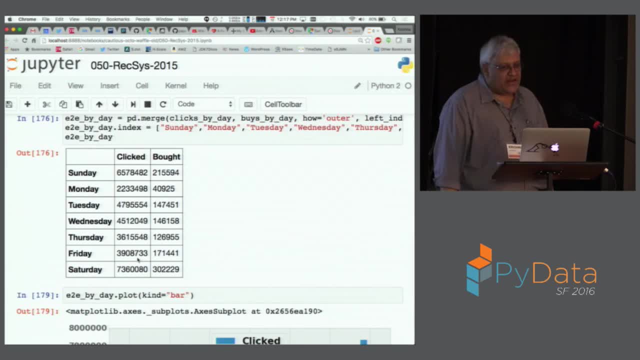 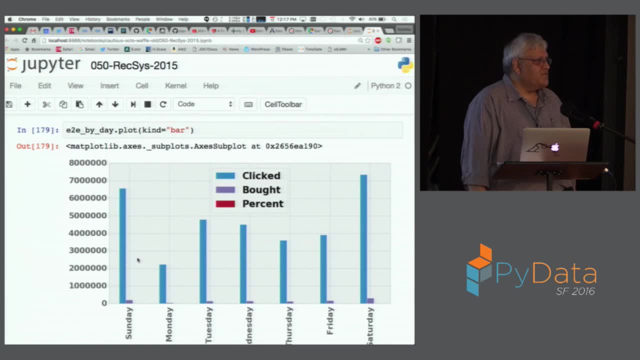 and you get this nice table. It says: on Sunday, these many clicks and these many buys, right Now you look at it and say: you can actually plot a graph if you want to plot a graph. right, You get the nice graph plotted, because you just plot it and say: hey, see, see how we 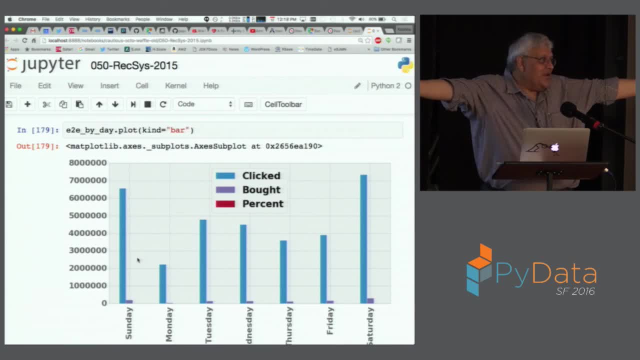 had this huge data right- This is like 33 million data right. We turned this around, we added columns, we did group buy, group buy, et cetera, et cetera, and we got this nice, this thing that looks at it and says now: